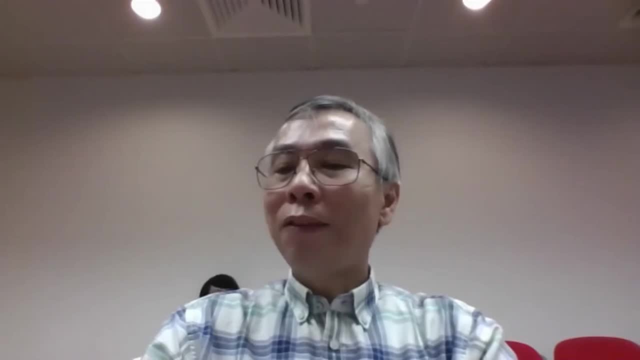 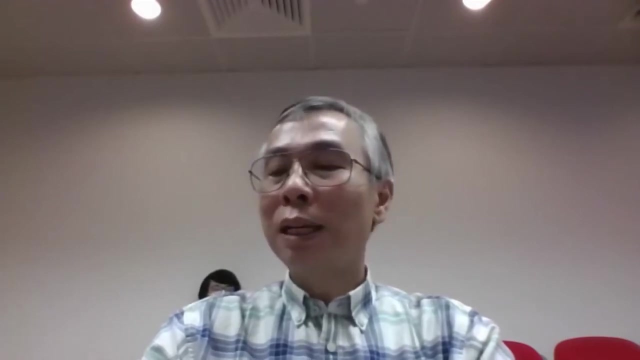 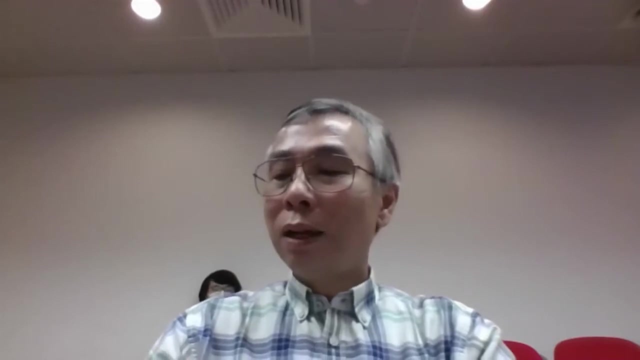 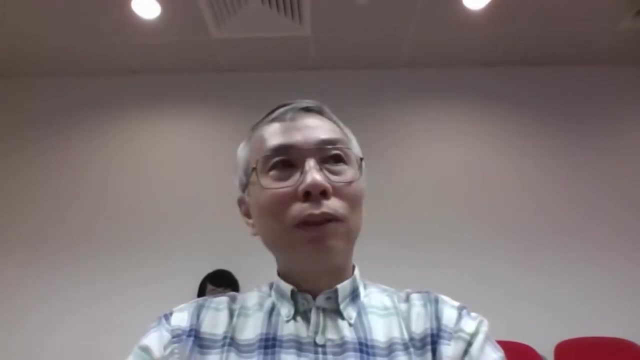 he is going to bring up several studies carried out by his laboratories, including a field survey of insects in local farms and genetic studies in insects in light to make new biotechnological applications, and genomic studies in establishing new models in agriculture to shed light on these neglected areas. Now please welcome Professor Hui to the floor. Professor Hui. 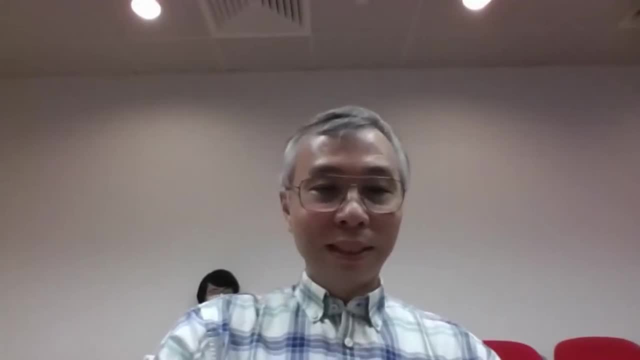 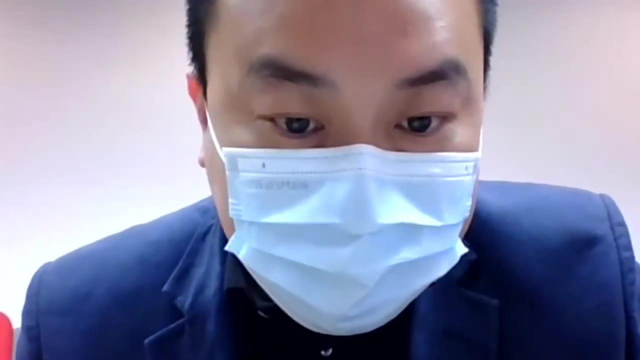 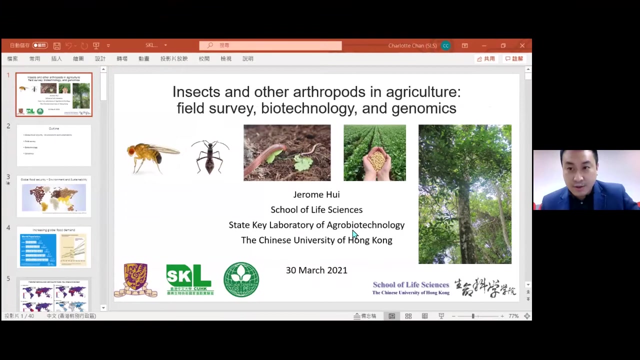 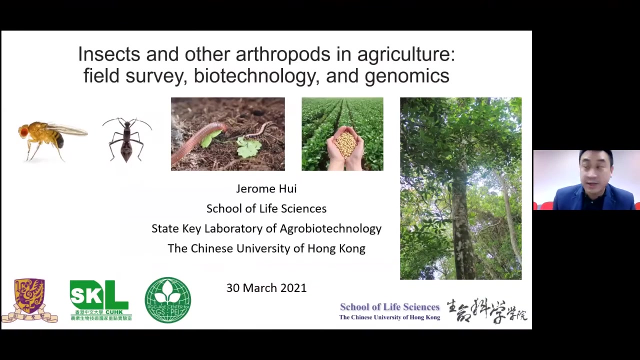 please? Thank you, Professor Lam. Can you hear me well, Okay, Thank you, Thank you everyone. Thank you, Professor Lam, for the very introduction and also an invitation. I also thank Joanna for the organization So well. I wasn't expecting that talk in the room and finally, it's later to be. 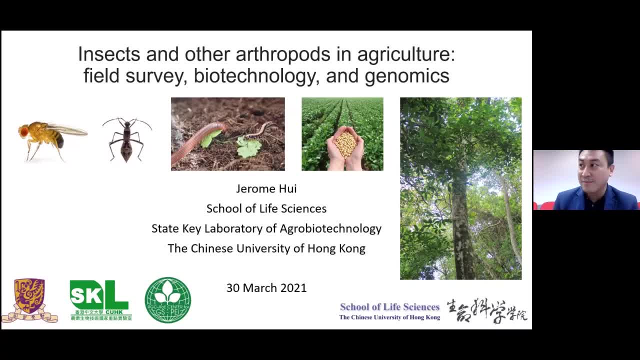 assumed. I mean I understand that people also coming from the other part of the world, I mean coming from South Africa, I mean so thank you. I mean I hope it's not going to disappoint you. So what I'm going to do today, I mean I'm. 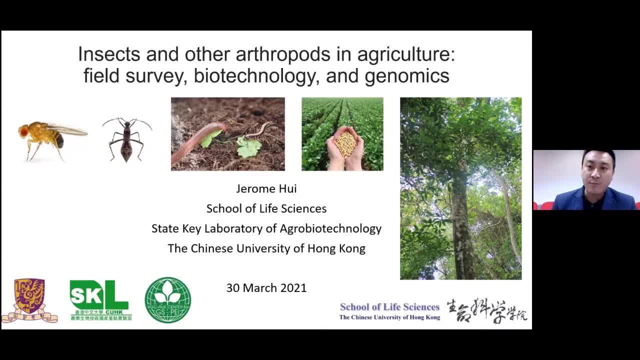 going to talk about insects and other arthropods in agriculture. So, typically, what I'm trying to do, I mean I understand that many of us, I mean our interest, I mean we'll be trying to improve the crop yields. I mean, while this is 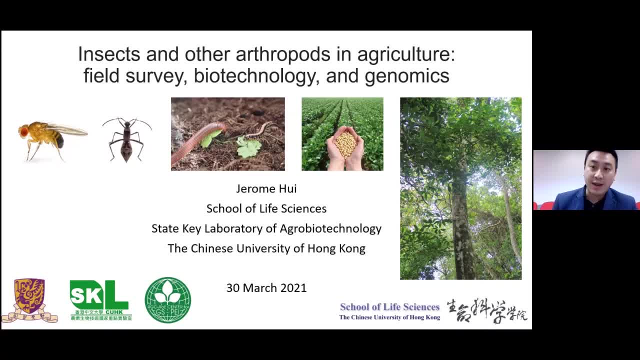 certainly very important. I mean we, especially in my group, we think that understanding the insects and other arthropods in agriculture can actually help in that way. So typically I mean I'm going to talk about insects and other arthropods in agriculture, So typically I. 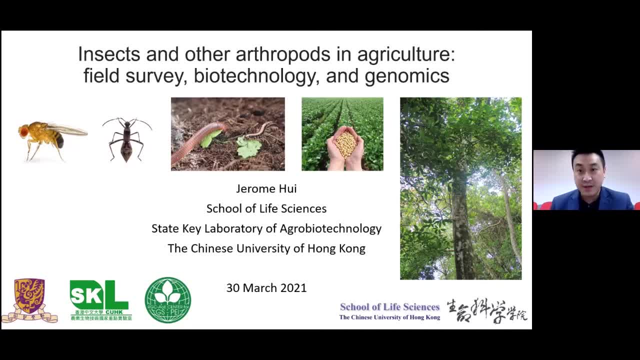 trying to do, go through several studies that have been ongoing or published coming from my lab. So I come from the School of Life Sciences and also State Key Laboratory of Agro-Biotechnology, and of course, I also need to thank the Area of Excellence I mean for funding the research and also organizing this. 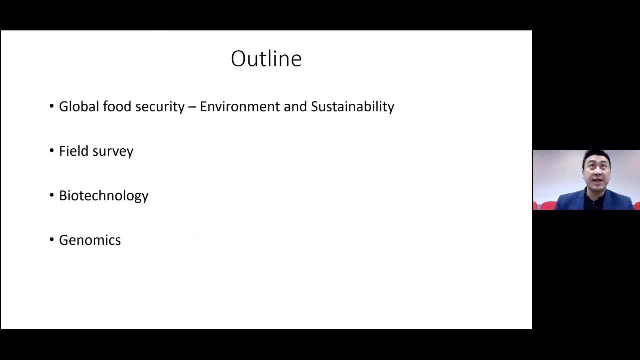 talk. So in the next 30,, 40 or 50 minutes, what I'm trying to do is I'm going to go through four big directions. I mean I'm trying to group them together. Of course it will be all relating to plants and insects and other arthropods. For the first part, I'm 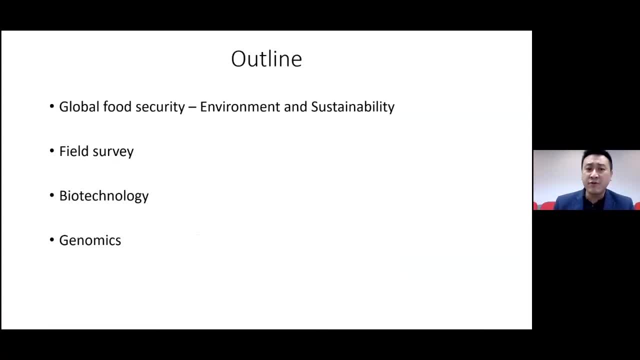 going to give a very brief introduction about global food security, especially relating to one of the major theme of our University, which is on environments and sustainability, and then I'm going to talk about an ongoing field survey that has been carried out by people in my lab. I mean, I will mention them later and then 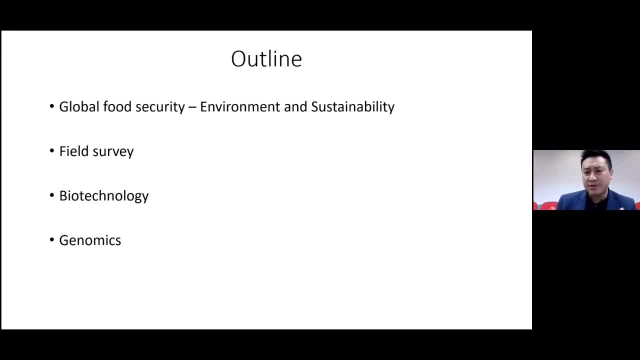 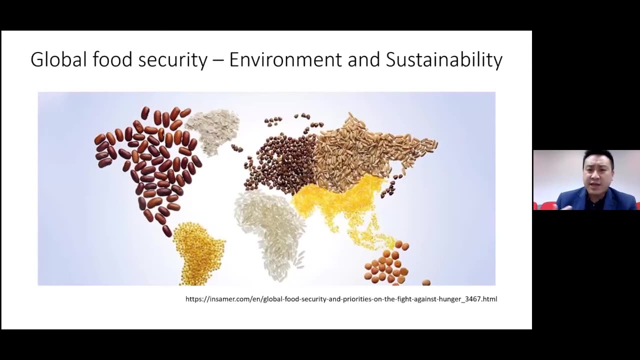 And then from field survey. when we understand what they are there. what kind of biotechnology can we do and how can we learn something from genomics? Of course I mean many of you know I mean food security is a global issue. 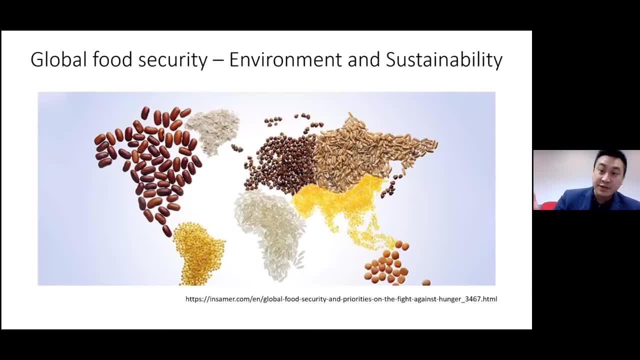 I mean I just take a picture coming from the internet. You obviously see that different places are heavily reliant on different kinds of crops. I mean this may be oversimplified. The point is clear. Nobody wants hunger. I mean we want to have food security. 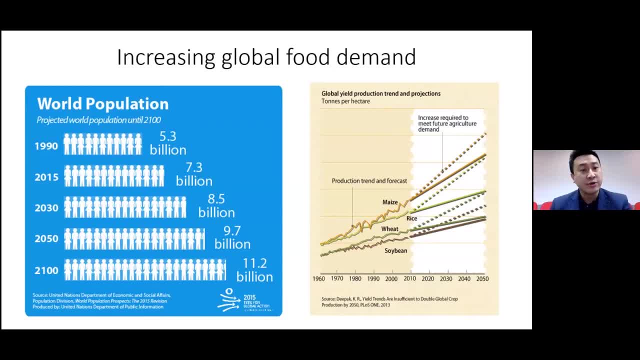 And especially that, if you look into the world population, world population has been increasing and seems to be predicted to be keep on increasing. So from 5.3 billion to now, I mean what we were expecting would be more than 11.2 billion. 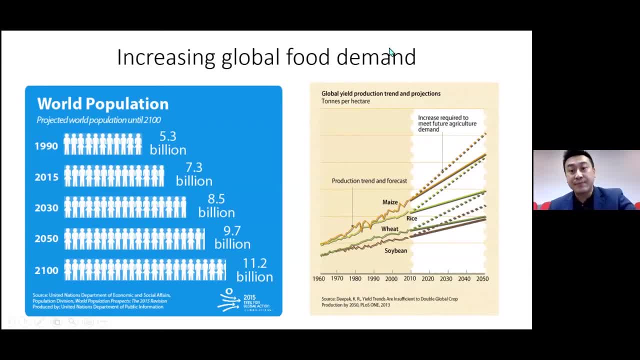 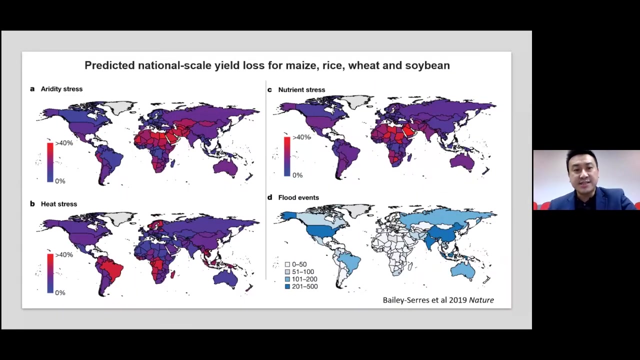 I mean by the time of 2100.. And when you look into the global yield production, you see that it's actually need to be an increase, ever increasing trend for the yield in order to meet this kind of increasing food demand. This is a study not carried by us and by the other groups. 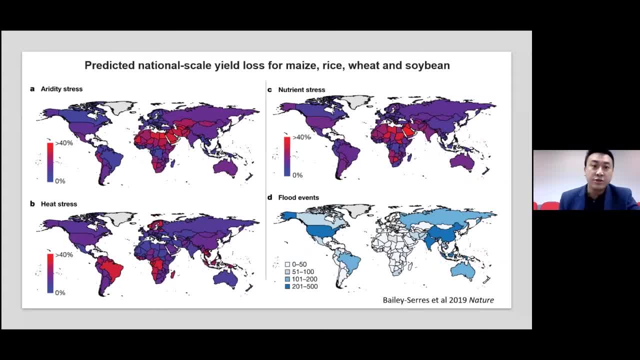 but what is it showing you here? I'll bring you through that. So this is trying to predict the national scale yield of loss for maize, rice, beef and soybean throughout the whole world. So there are different reasons for them to cause. 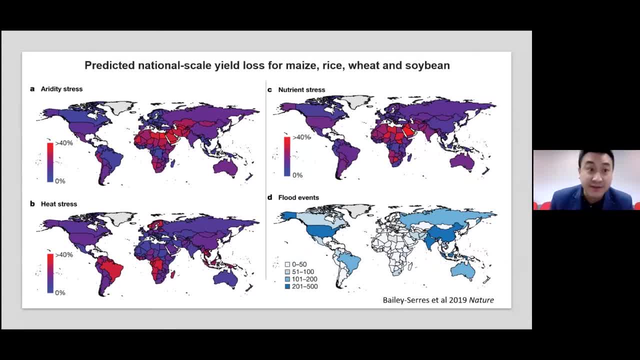 for the loss. It could be including the environmental factors changing, like the de-stress or flood events, et cetera, But one thing that I would like to point to you is the coming slide, which is global loss, which is global loss of crop production. 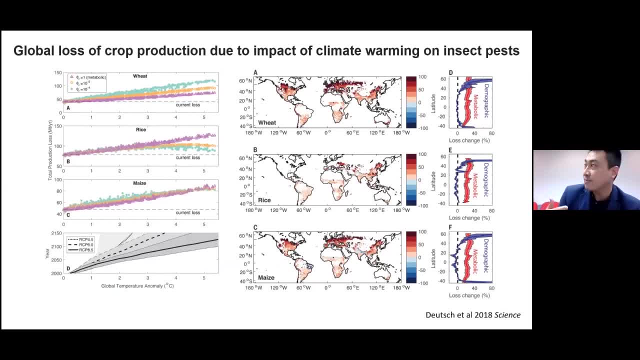 is also due to the impact of climate warming. At the same time when climate change, insects numbers will also change, And typically when for those that are insect pests they will be intense, seems to be increasing. Again, this is not a study done by us. 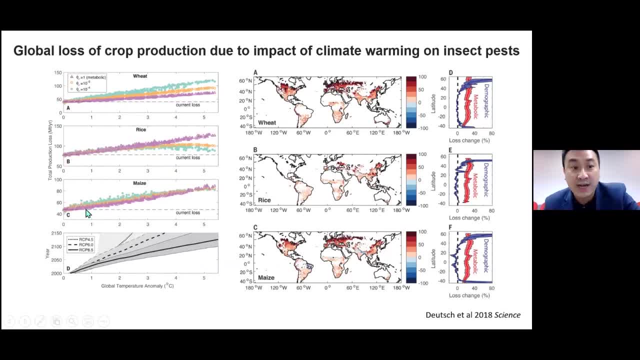 but when you look into, if you follow my mouse cursor, weeds, rice, maize and soybean, et cetera. So throughout the whole world climate change, I mean it actually increased the metabolic rate for the insects. So basically what the point I mean to bring over here. 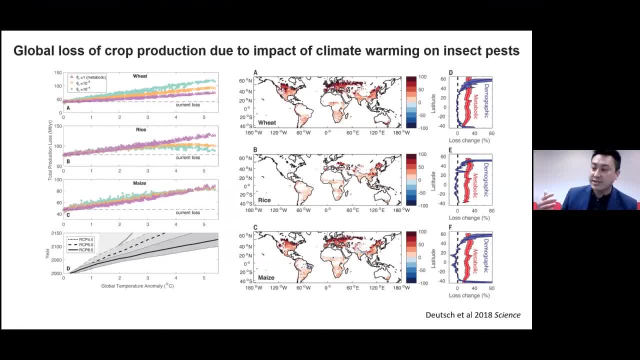 is that, well, when the temperature is going to increase, you increase the metabolic rate of the insects, And when you increase the metabolic rate of the insects at the same time, I mean you have more and more insects, I mean the generation time is going to get shorter, et cetera. 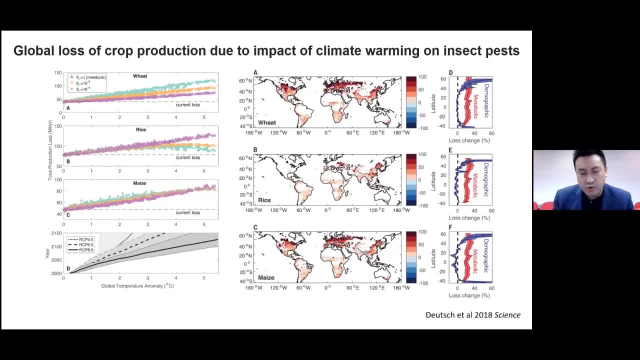 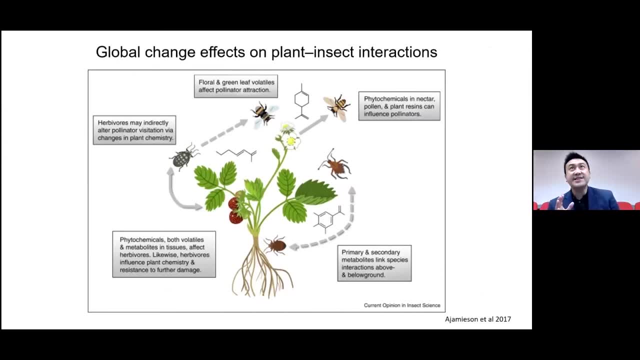 And then eventually, if you have more insects, you lose your crop yield. But what I'm trying to show you in this slide, I mean, is that insects and plants- I mean typically, when we are talking about crops- are actually very, very related. 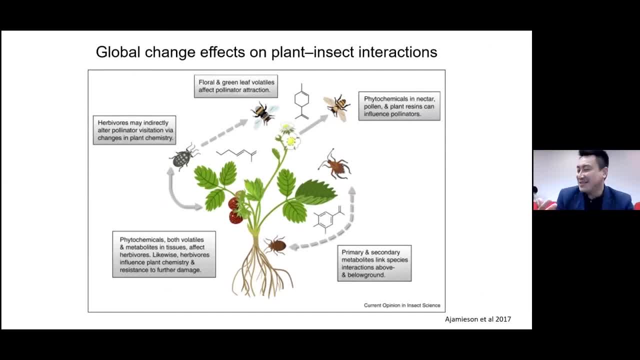 I mean you. well, we don't think insects as just a term. I mean, unless you will be differentiating them into two big groups, if you want. I mean So unless you will be thinking about something like pests, I mean, to which they will be targeting your crops. 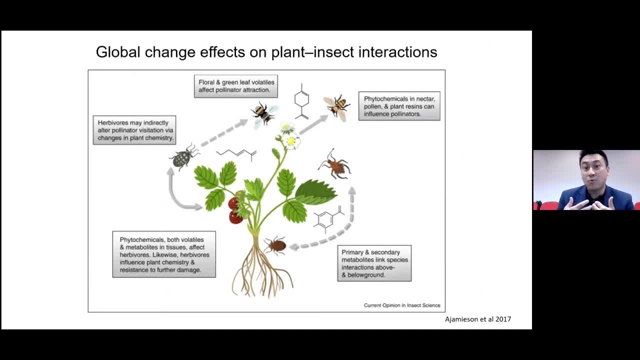 But at the same time, some insects are good. for example, They will- I mean like bees, I mean, or some insects that will be taking away your pests. So we also have beneficial insects Other than the two types of insects. 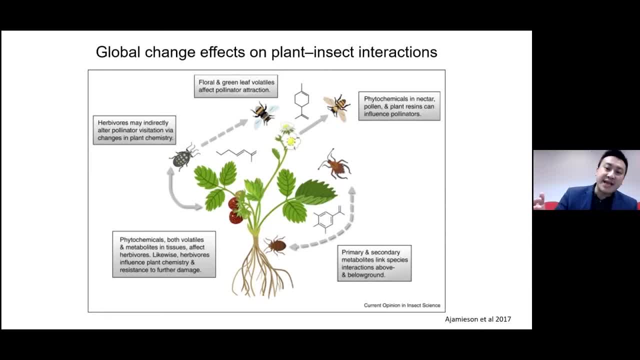 the other thing that we need to consider is that plants and insects actually have evolved a kind of interaction, For example. I mean, I don't have time to go through, I mean, so I picked up one very good review. If you're interested, you can go and read it. 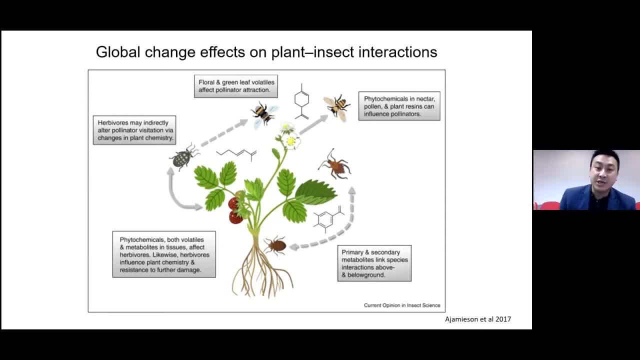 So basically plants would produce terpenes to attract- I mean bees, I mean et cetera- other beneficial insects At the same time, I mean insects will also pose some different interactions onto the plants. So plants will also go back into defense et cetera. 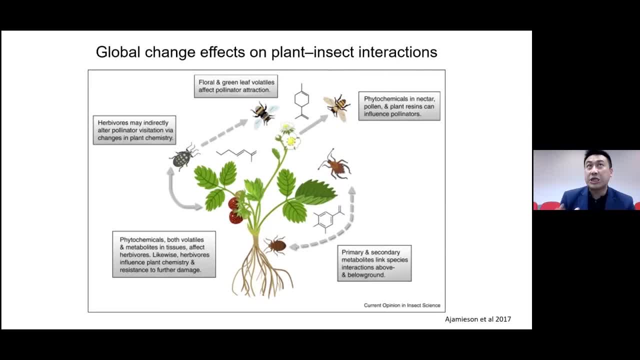 So it's a very, very interesting interactions. But when we look into modern day of trying to estimate a crop yield, well, usually many people will think, oh, insects may not be so important Because traditionally many of us have been thinking if we can keep on increasing the crop. 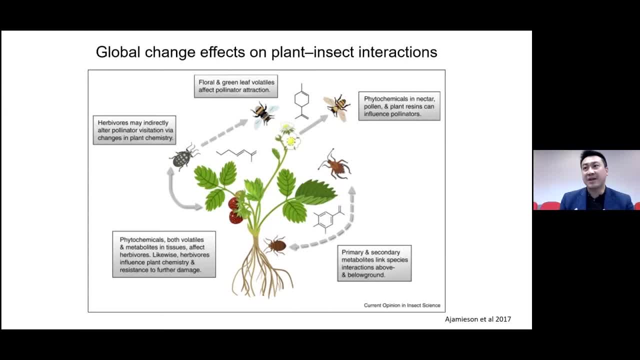 yield. That should be fine. But now people think that because of climate change, that insect interaction, especially the influence for insects on the crops, actually increased tremendously. So even though if you can double your yield, well, the insects, if they, grow even quicker. 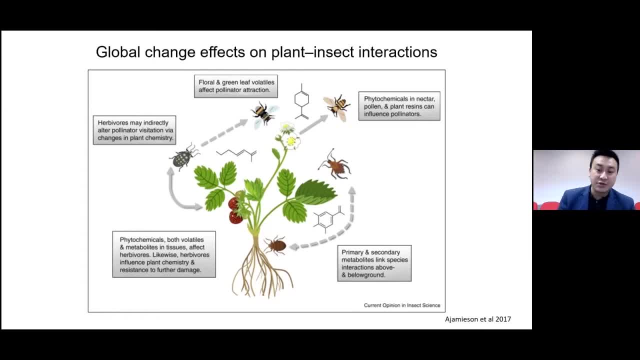 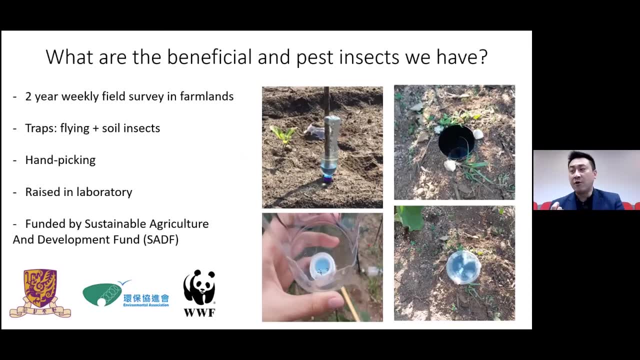 you can completely demolish or damage your crop production. So I hope I will be able to bring you the importance for accounting, the fact and factor of insects into agriculture. So now I'm beginning to talk about studies carried out by my lab. So one thing that the first thing we come into 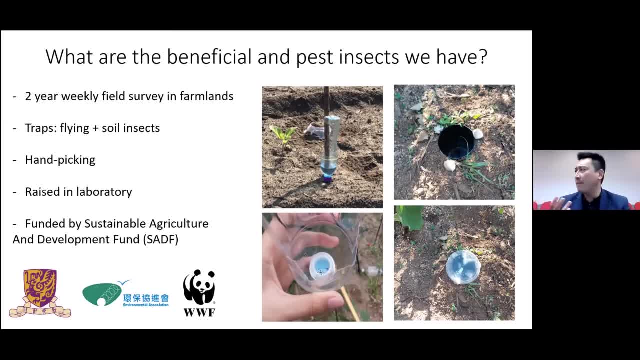 is the thinking: well, what are actually the beneficial? or the pest insects that we have here in Hong Kong? So very fortunately that we have been funded by the Sustainable Agriculture and Development Fund. Together we have been working together with the Environmental Association and also. 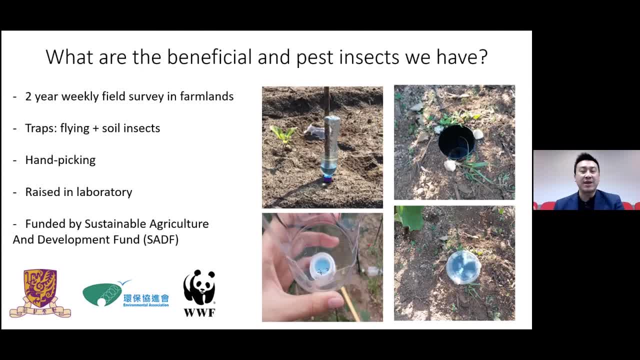 the WWF of Hong Kong, But together of course. I mean we have some very talented personnel in the lab which I will mention later in the next slide. So we have been doing a two-year weekly field survey in farmlands. 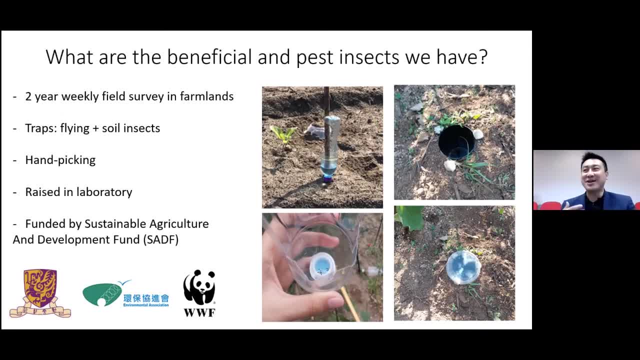 So these young people, I mean what they're trying to do is they go to the field, they set out traps like what I've been showing you here, trying to look into doing the flying traps for flying insects and also doing the traps for the soil insects. 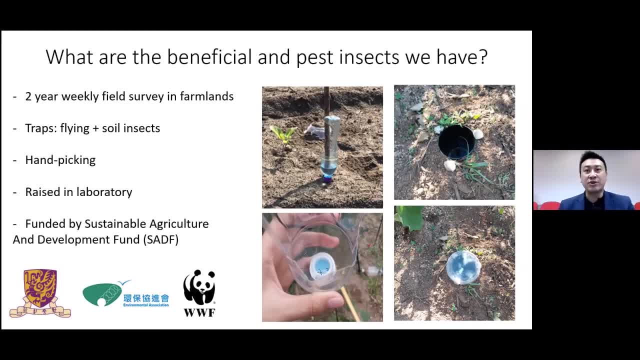 They also do hand picking And then we also try to raise some of them in the lab And the way to try to do that, because now we don't really have a big clue or we don't have understanding what is actually happening in the farmland in Hong Kong. 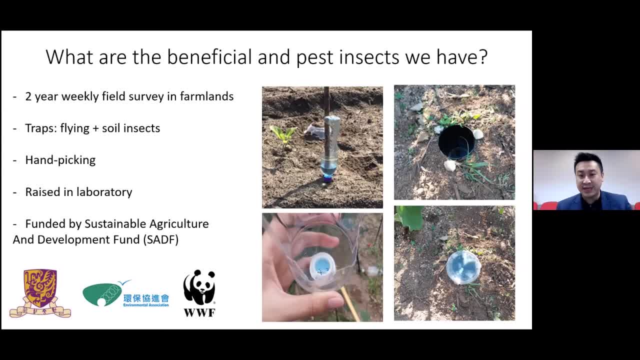 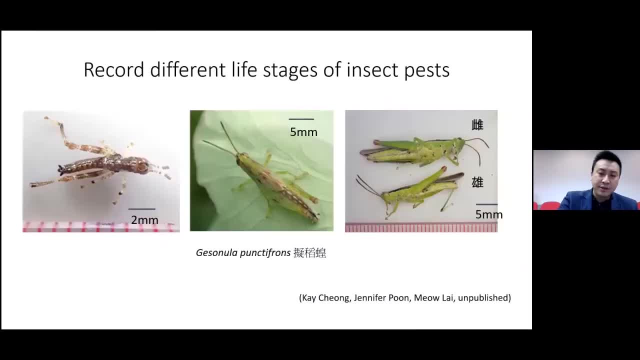 right now and through this study, which is still an ongoing study- we're in the second year now and we will finish it by the end of the year- I want to share with you some exciting results we have got. So typically, I mean, if you look- 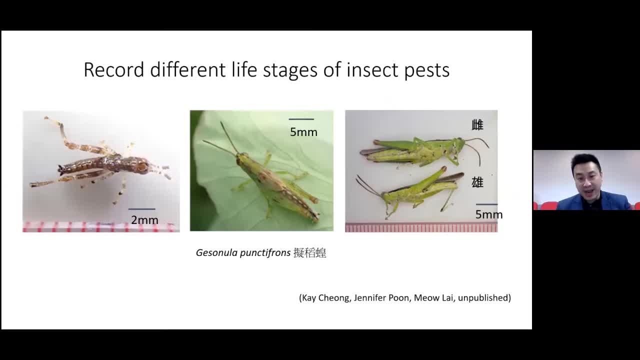 into the bottom of the right-hand side. this has been done by Kay, Jennifer and Mel, I mean in the lab. So after the hand picking they try to go back into the lab and try to raise them, For example a locust I mean they're showing you here. 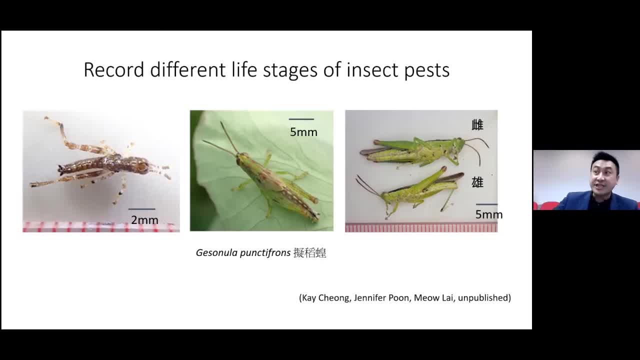 Well, we will be able to document different developmental stages. I mean, rather than people will say, oh, this insect's a juvenile stage, I mean, or a lot of these stages it's very difficult for us to identify. So we have been trying to do that. I mean. 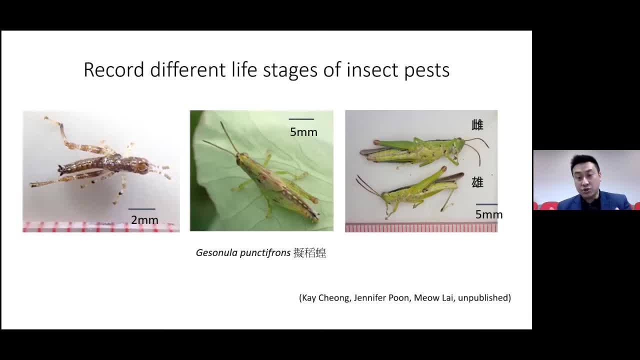 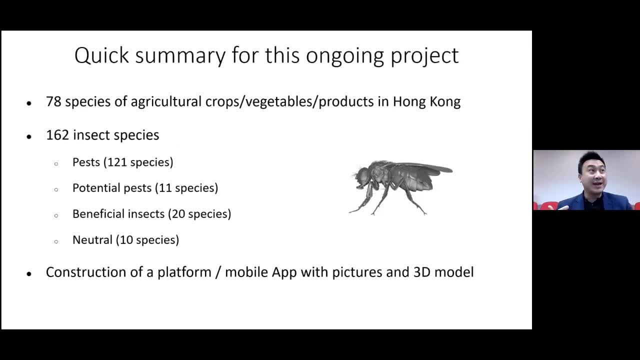 for all the insects that we'll be able to get and obtain in the farmland. So a very quick summary, I mean, which seems to be unfair to their very hard work. We have lots to share today. So, basically, today we have already. 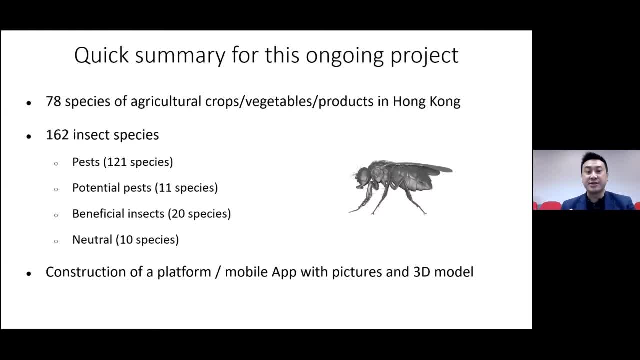 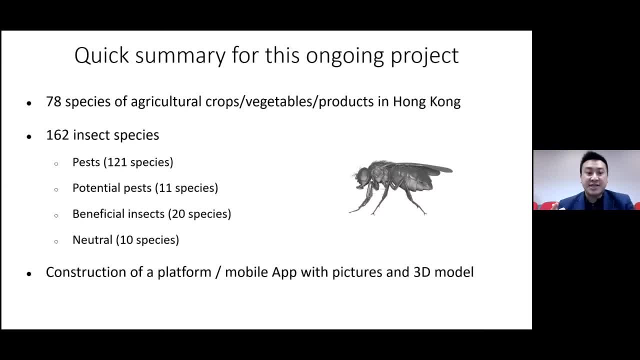 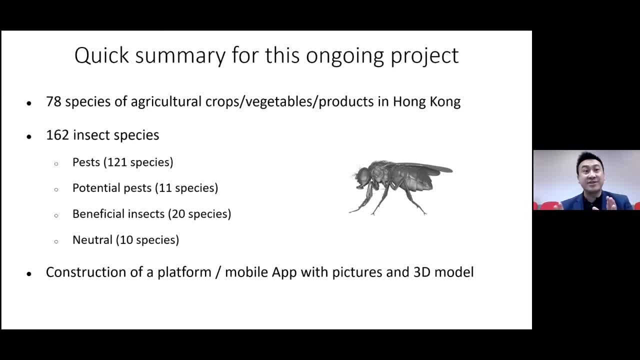 And 10 of them are neutral. So I know you're very interested in those. Don't worry, At the end of the talk I will show your website. You can go and see our ongoing work. But the end of this project funded by the SADF. 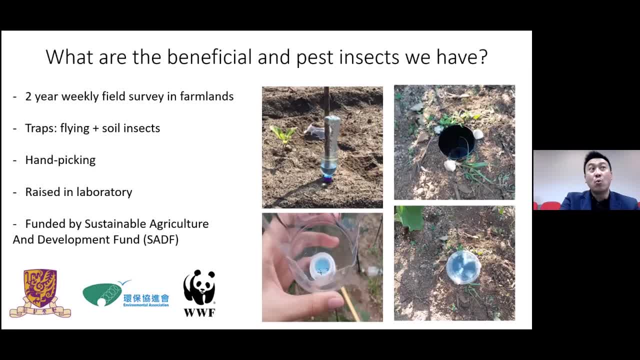 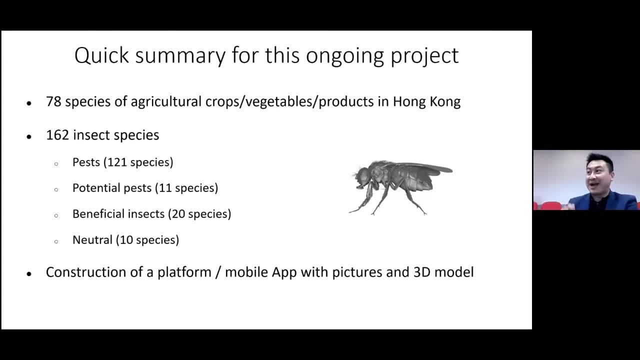 together with WWF, we have an environmental association. We are actually trying to make an app, okay, So there will be a mobile app that is freely available You can download on your mobile phone. So it will be something like we are. it's only a prototype right now. 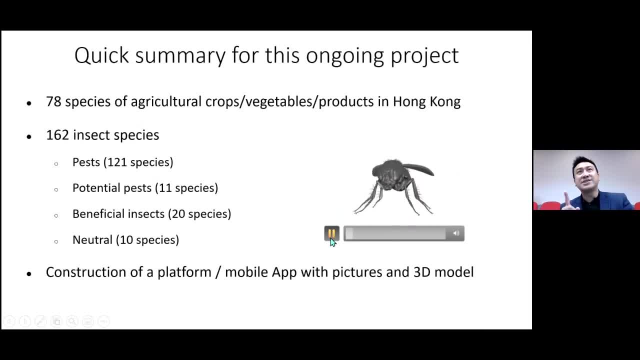 I hope you'll be able to see, and I'm going to show you a video, So it's not going to be like exactly like this, but this is a 3D model for a fruit fly that we get from the field. 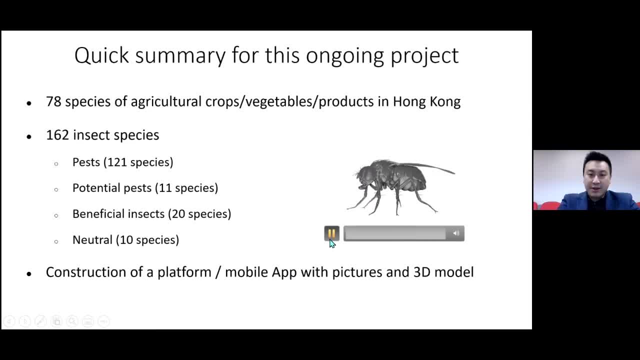 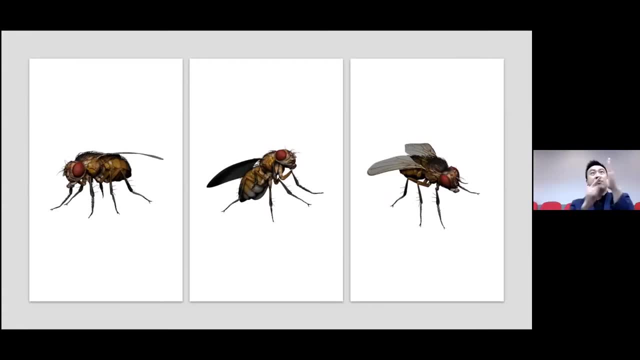 So, of course, when it's properly done. okay, sorry, can I go to the next slide? It will be a 3D model on your mobile phone. You can actually rotate it, okay, So we will be doing that for around. 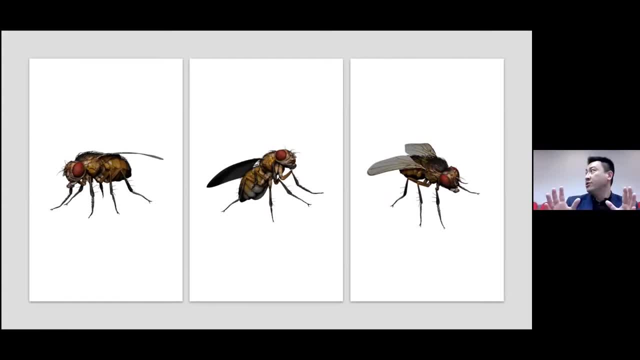 50 common pest species in Hong Kong. So you oh, and then you can say oh, when you're growing a vegetable or maybe a cabbage in Hong Kong, and you say, okay, I see, oh, there's a worm. 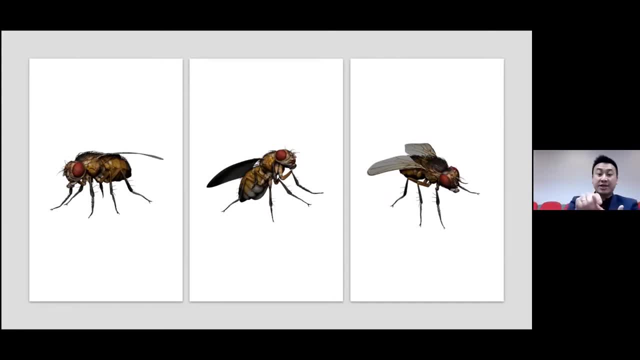 We always call them worm, that what that is- And on your app then you can actually do a 3D model And then you can try to find that. but you say, okay, that's the caterpillar or the cabbage fly. 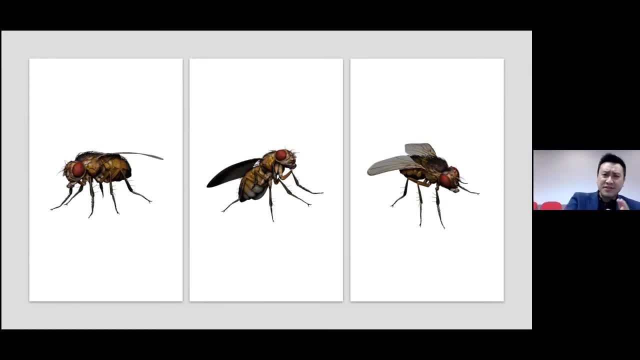 Okay, for example. So this is ongoing and of course, it will be a. it will be a very, very informative app, And also we have a website within that. We will show you the link and give our interest over that. At the end of this year, this app will be available. 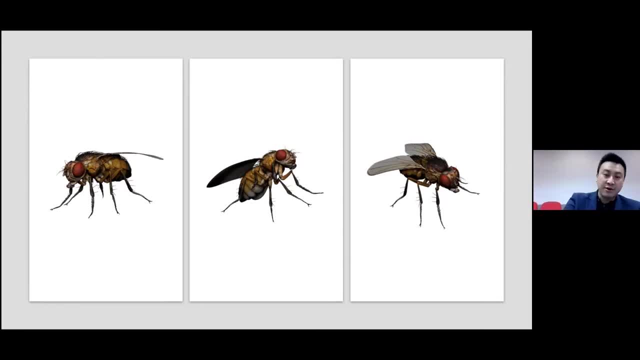 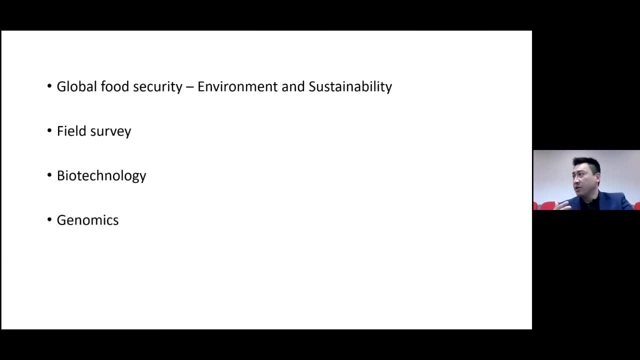 And we will also document all the paths that we will find find in Hong Kong. So now I want to move the gear a little bit, of course. I mean, we now have a better understanding about the past in Hong Kong. What can we do? 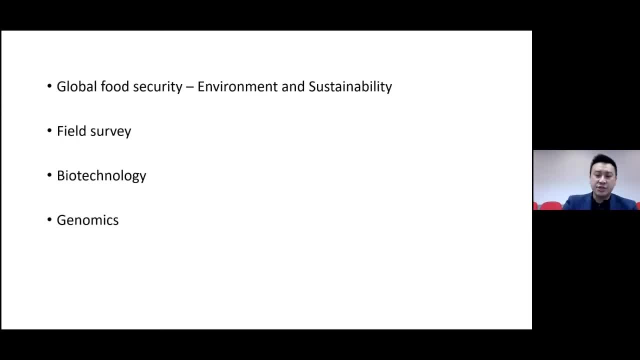 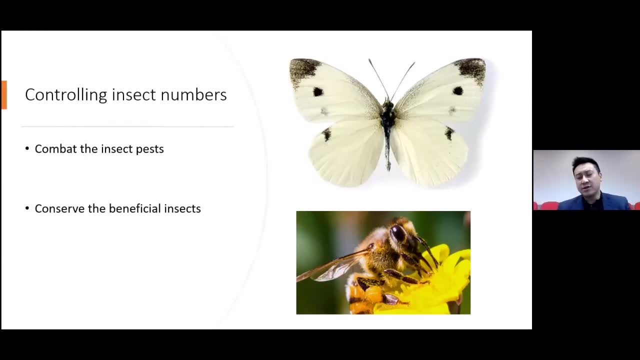 okay as academics in universities. So we try to do something slightly. I mean, we always try to do slightly different things on two aspects. For example, we want to control the insect numbers. On the good side, we want to convey, so we want to attack the insect pest, we want to eliminate that. But I 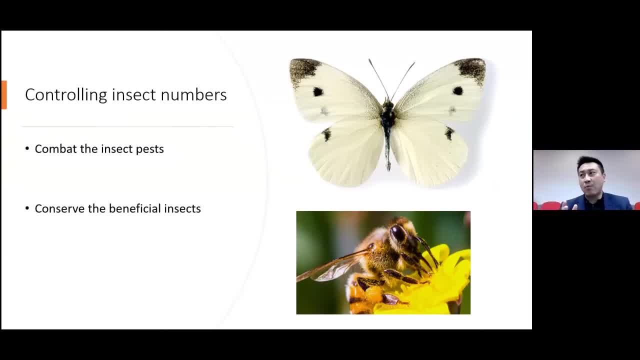 will show you what are the problems that we have right now. I mean, so you say: well, why can't we just use insecticides to do that? There's an issue for that, I will tell you later. But at the same time, we also want to conserve. we also want to. 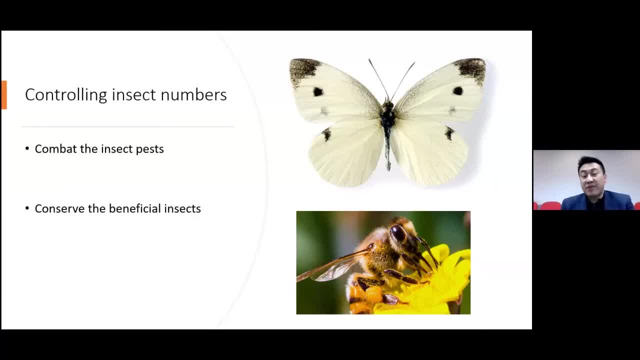 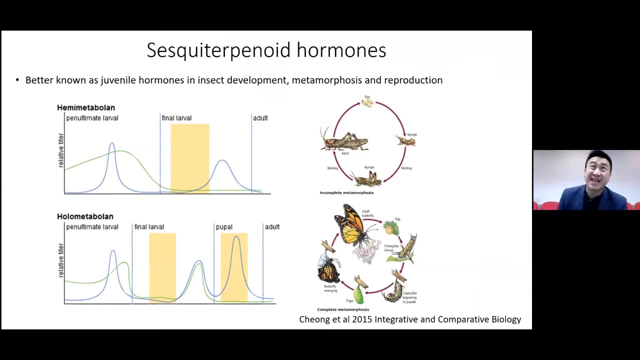 control the insect numbers by, for example, some of the beneficial insects, can we boom their numbers? So we want to increase the number of beneficial insects and we want to decrease the numbers of insect pests. So here I need to begin to introduce a slightly more academics. I hope you're okay. 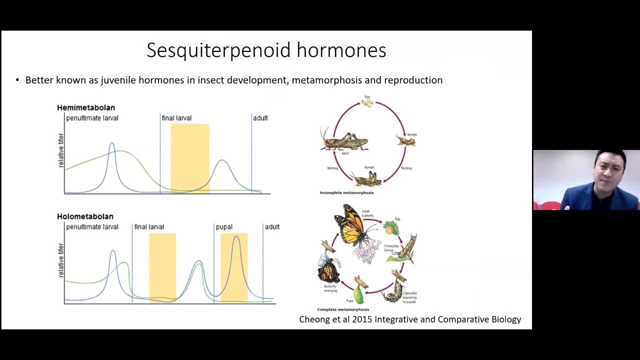 I understand people are coming from very diverse backgrounds, so allow me to go through this slowly. So in insects, of course, if you further divide them biologically, we can mainly divide it into two groups. Of course there are more groups. 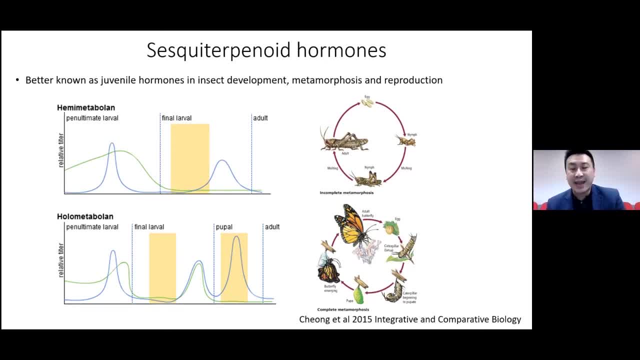 but let's introduce two groups today. They are the hemimetabolins and homometabolins. What are they? You can look into the picture on the right-hand side. okay, So this is the grasshopper, For example. this is incomplete metamorphosis. 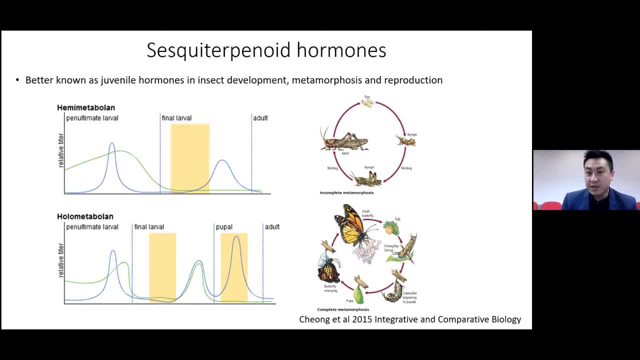 Once they are born from the egg, they hatch out from the egg, they are nymphs, and then they just grow in size- okay, This is what. and then they pretty much look like more or less the same like the adult when they're born. We call them hemimetabolins. that means 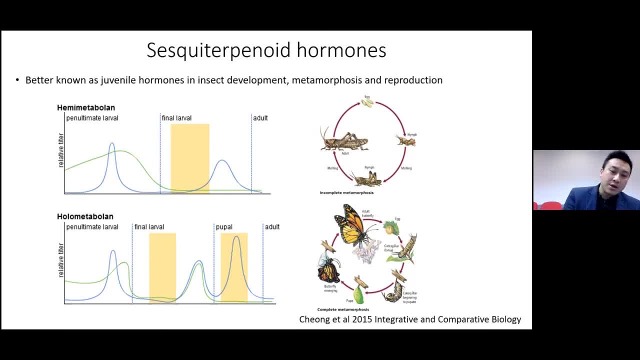 they do incomplete metamorphosis. On the other hand, I think the typical example that they will go through complete metamorphosis are those like butterflies, For example. I mean the picture on the lower panel. when they hatch from the egg, they become the larvae. 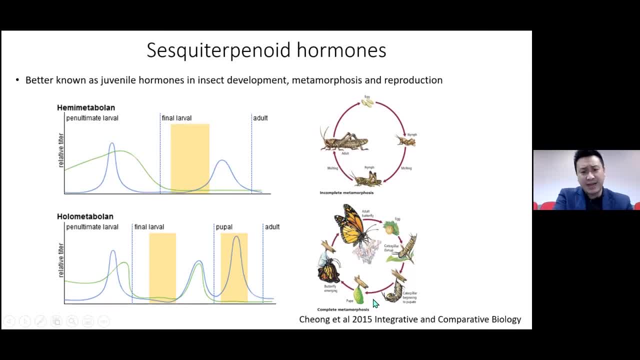 The larvae are feeding on, for example, leaves. They eat enough, then they go into different stages. It will become a pupae For the pupae, then they further develop and then become the adult- Adult in this case have wings, go to another territory and then are mates again, and then 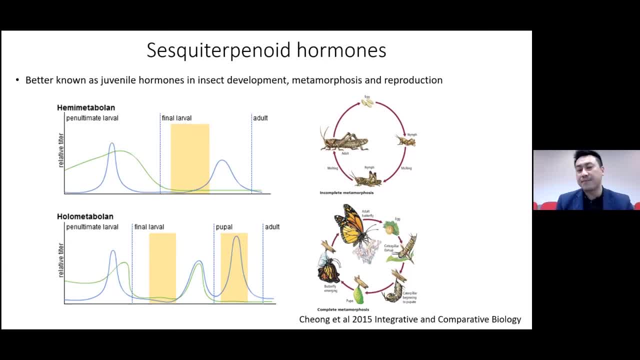 have eggs. This is what we call complete metamorphosis. In either case, no matter the hemimetabolins or the homometabolins, what is actually controlling them for the development? is this green line? okay, It's this green line, no matter on the hemimetabolins or the. 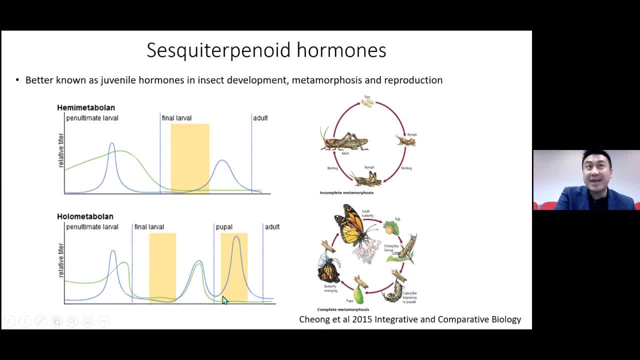 homometabolins is this green line which is actually the hormone, the hormone titer, And it's called juvenile hormone. So they are kind of sesquiterbinoid. don't worry about those, let's call them juvenile hormone first. They're called juvenile hormones because at 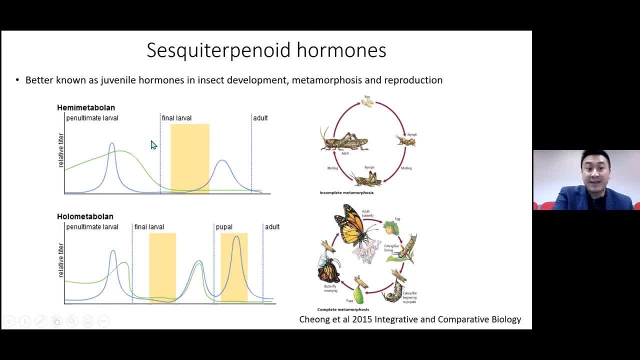 the juvenile stage. they have a lot of juvenile hormone and then suddenly you drop the juvenile hormone And after that then, for example in this case, they will come from nymph and then become adult Metabolins. they will go through different stages of metamorphosis, from larvae, pupae to adults. 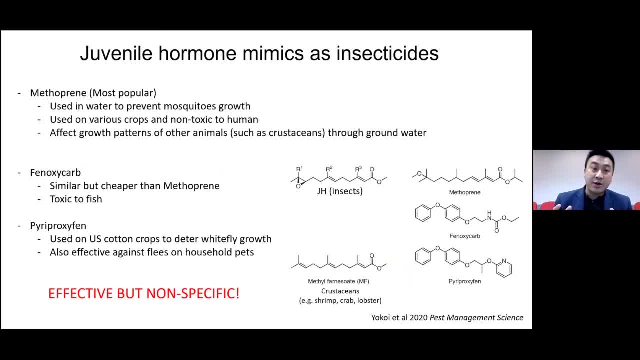 The reasons I want to bring you onto the sesquiterpenoid and typically on the juvenile hormone, is because it is a very, very important hormone for the regulation, for the growth and development of insects And actually because of that people also use this as the drug. 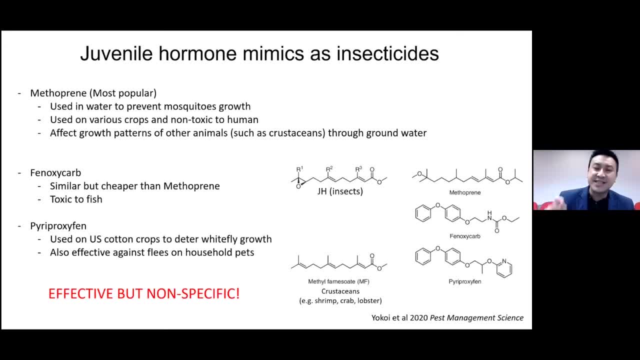 And in this case it's the insecticides. They're so powerful. This is a slightly busy slide, So let me go through the left-hand side first, on the woody bit, before I go into the whole diagram bit. It's very difficult to synthesize chemically juvenile hormones, so you cannot produce a lot of juvenile hormones. 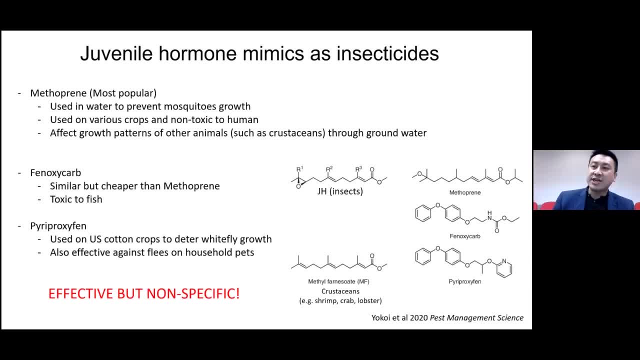 That would be so expensive to do. So what people actually do? they try to synthesize some chemicals, And I in a structure, chemical structure that is very similar to juvenile hormone. So if you look into so, they are called nephropenes. 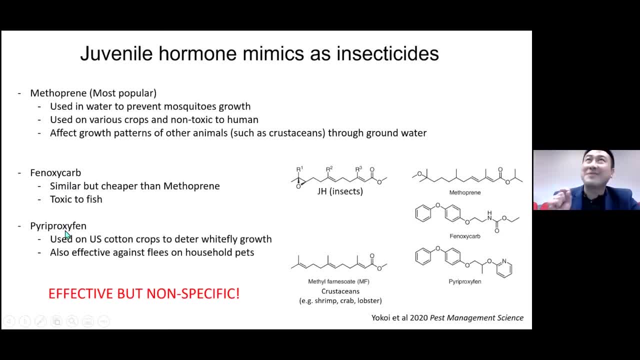 phenoxycarb in cadhexidate and also pyripropylOH. Okay, so in these three cases, if you look into the distractor on the right-hand side, so they- this is the insect juvenile hormone, very difficult to chemically synthesize. 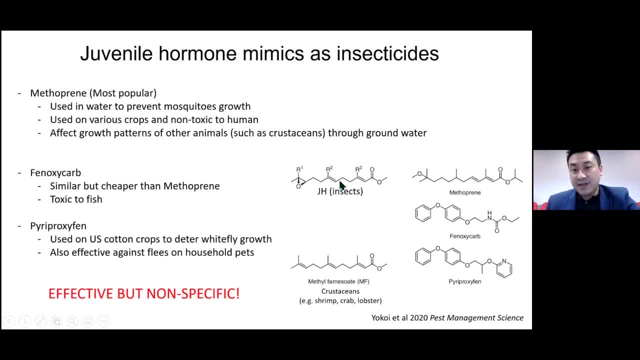 This is the one that is look-like. I mean having backbone, I mean modify a little bit structure So they can be synthesized cheaply, inexpensively, and they actually, for example, mephropene for many of the 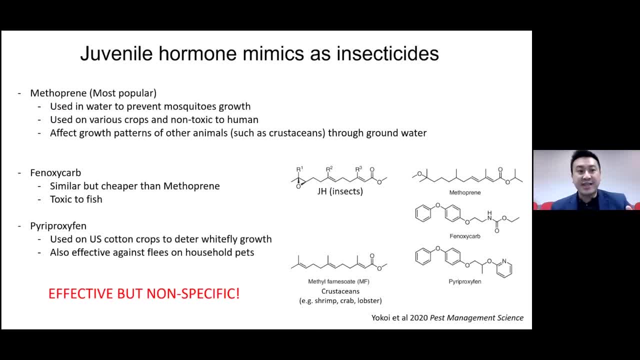 reservoirs. I mean, for example, in the United States. they will put mephropene into the reservoir in this case, because, well, the more squirtle needs to be a little metamorphosis from catching larvae, and then it will become the 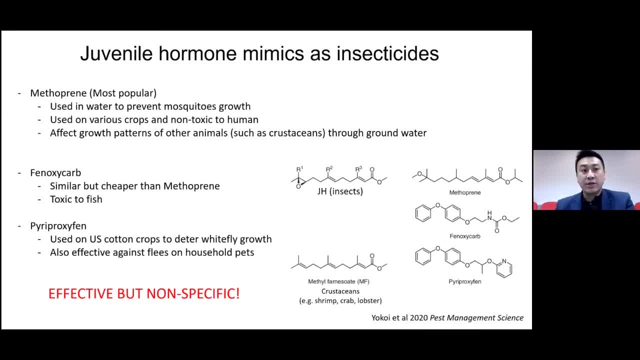 petal mosquito, right? So if you put them in the water, it will prevent mosquito growth. okay, But this is because they are using a chemically synthesized structure. In that case, they're not specific. They're not specific. On the other hand, it also affects other animals. For example, you may have 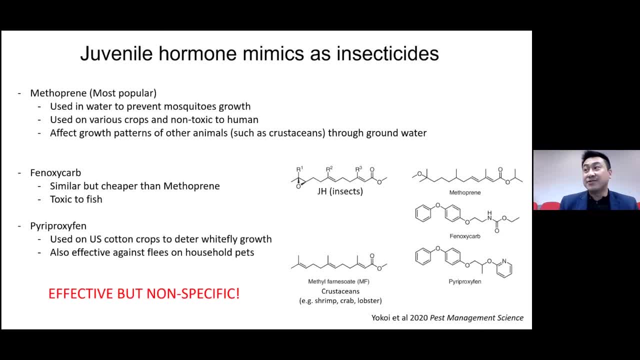 a crustacean. It's like crayfish in the reservoir, so they're also affected because the structure is very similar. On the other hand, you have phenoxycarb. They're even cheaper than mephropene- also useful, but if you put it in the 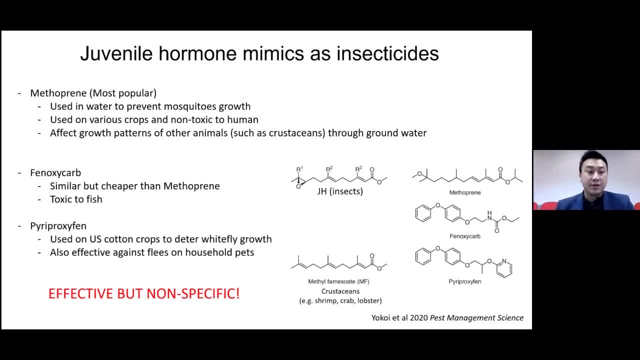 reservoir, etc. they're also toxic to the fish. The other drug is used to be using- actually used on the cotton crops to control the whitefly growth, but it's also useful for the fleas. I mean household pests. A major problem is that they look like juvenile. 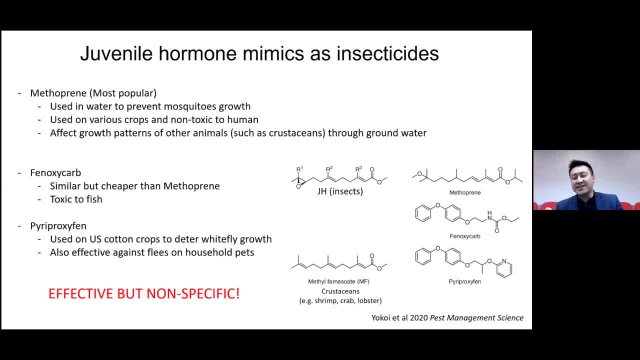 hormone. if they are specific, They are not specific to sets, but they can also be needing to be toxic to other groups, Even though they seems to be more specific to insects. you have an issue. The issue is that you will be indiscriminate Either. if you remember, I was saying they are pests, of course. 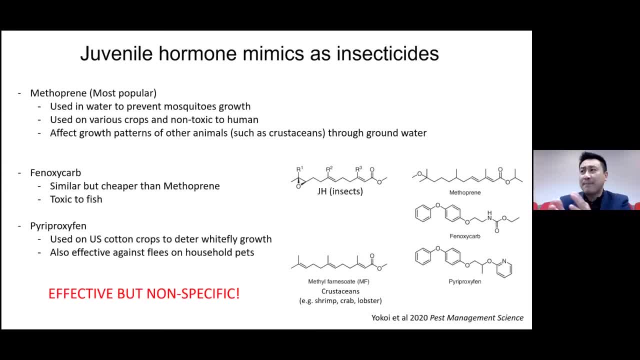 you eliminate them. But if they're beneficial insects, for example bees, they will. Koreans, because you execute the sollten sciences. when you can't control them, They in another way. it will also affect the bees. so yeah, you're affecting all the insects, or even 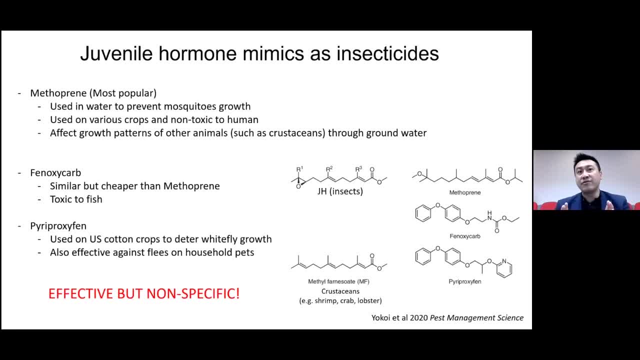 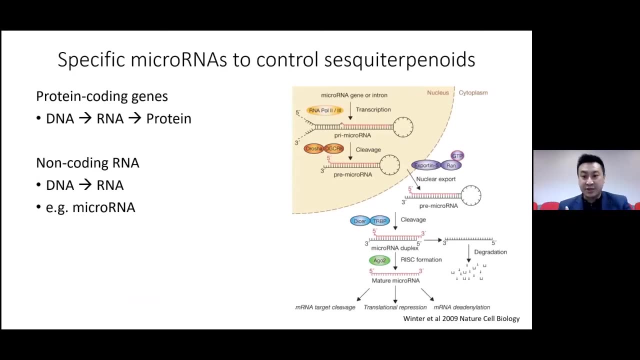 non-related groups. okay, so this is the problem of using juvenile hormone mimics as intact insecticides: very effective but not specific. so my lab has been trying to do this. i've been almost in cu for nine years, so we have been trying to do almost a decade trying. 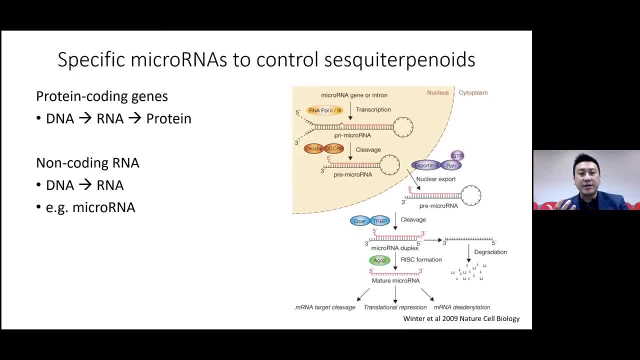 to understand this question. so we want to develop something that can be specifically also control the juvenile hormone, but at the same time that would be specific to that particular animal rather than to all insects. you see what i mean. so here i understand. people are also coming from. 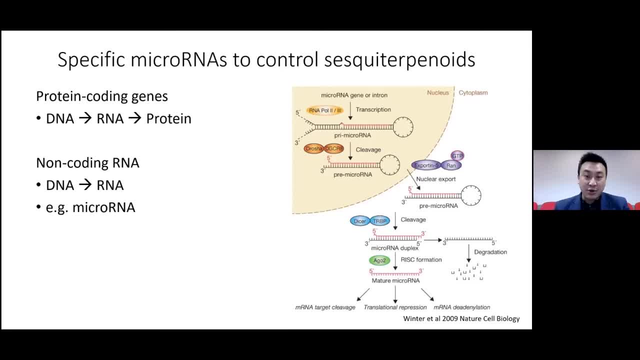 very, very diverse background. so what i need to do is i need to go through this, uh, briefly, very, very briefly, okay. so, uh, for example, if you understand the central doma, that we, we are protein coding dean, we, we have a dna transcribed for an rna. 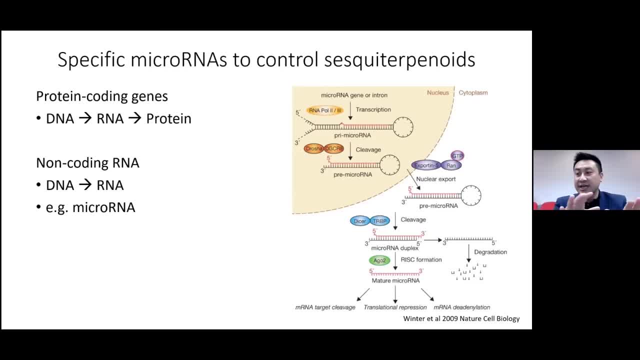 rna translated protein. you know that insulin gene rna and then we produce insulin. okay, so juvenile hormone genes produce juvenile hormone, i mean, etc. so non-coding rna are are kind of rna to which they will be encode from dna to become rna. they will not be translated into protein. 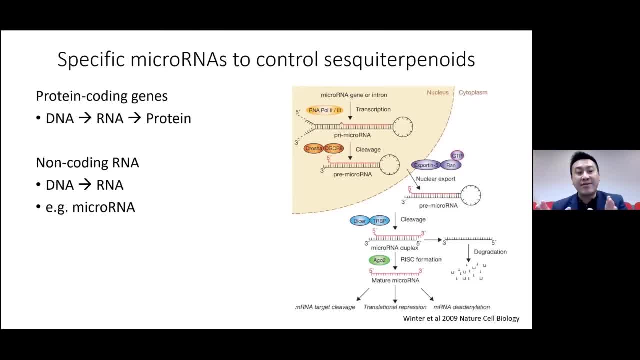 but this kind of rna and now, for example, micro rna, okay, one type of, uh, small rna, which i'm not going to go into the detail else, but because of the diverse background that we have here they will be, actually will be able to target, for example- if you felt sorry, follow my mouse cursor- the micro. 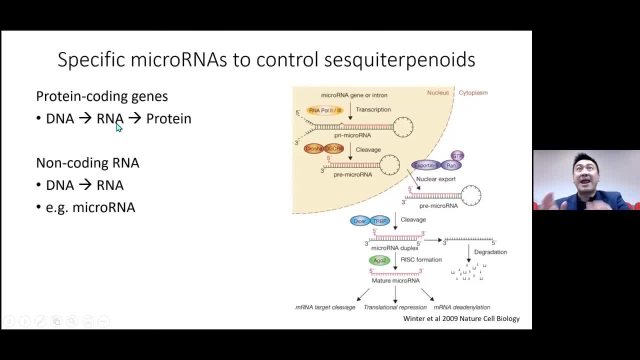 rna will target back into the rna and affect the protein expression. so in that case, for example, if you have a micro rna being present, they will target the juvenile hormone. synthetic pathogens, an enzyme, for example, then you theoretically you will affect the juvenile hormone. that's the whole idea. uh, long story short. yes, uh, it's possible. 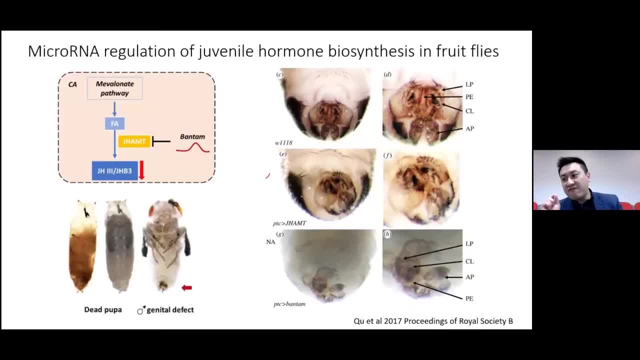 so we found the first micro rna that is actually targeting juvenile hormone biosynthesis and fruit flies, a few years ago. so, um, if you, if you see what i'm showing you here- i mean this is the summary- we find a micro rna called pentam. this pentam is going to target a 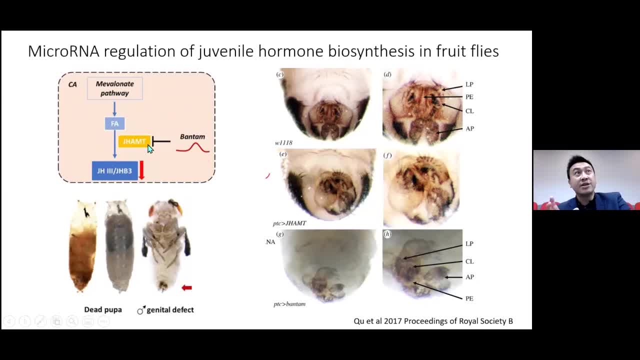 gene for during how juvenile hormone acid mufa transference. don't worry, because we know that the hmt- this is an enzyme that is going to- is the last and most crucial step for the synthesized for juvenile hormone. so once you have a micro rna, 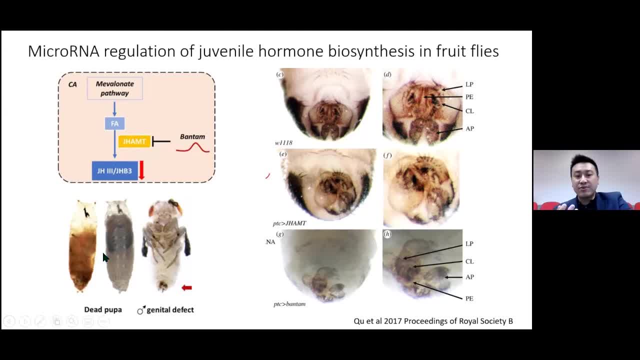 targeting here. we put them into the fruit fly, you will either result in epupy- okay- or those that may be able to escape- eventually they can't- you will have a genital effect. what is the genital effect? follow my mouse cursor over here. this is the w11x, which is 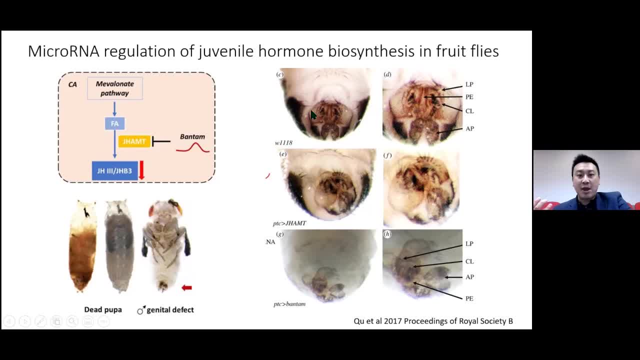 close the wild type: this is a male, okay. this is a male penis, okay. so the male genital organ is supposed to be a straight orientation. so when you have the female you, you insert your penis into your vagina doing fertilization, but in this case, when you actually modulate, 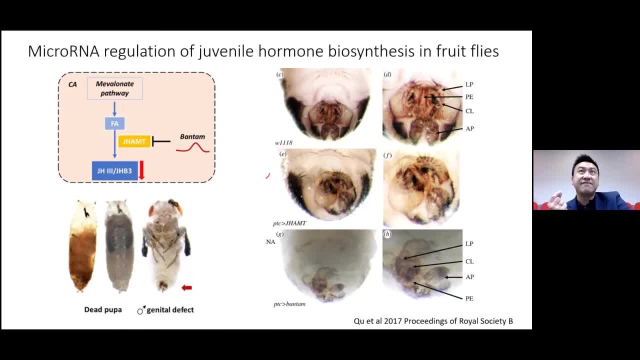 the activity for for the juvenile hormone gene gene first, okay, what you're resulting is the misorientation. your, not your, sorry, the fly penis that's going to get this orientation okay, and when it's misorientation, what is actually? they cannot actually cross and you're right, those flies become 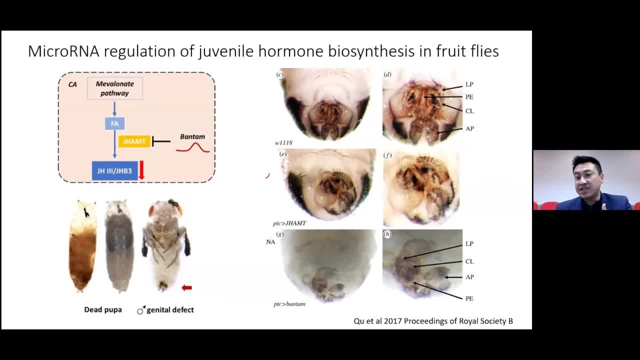 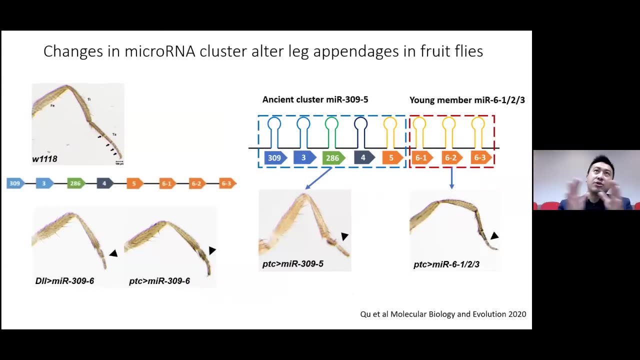 sterile, okay, so they're not able to produce the next generation. and of course, if you use the micro rna, bent time in this case, you cause the death and also genital misorientation. so and recently we also begin to look into other microorganisms inside the the, the fly genome. 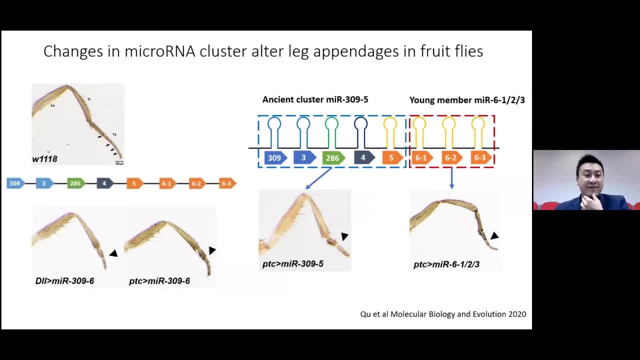 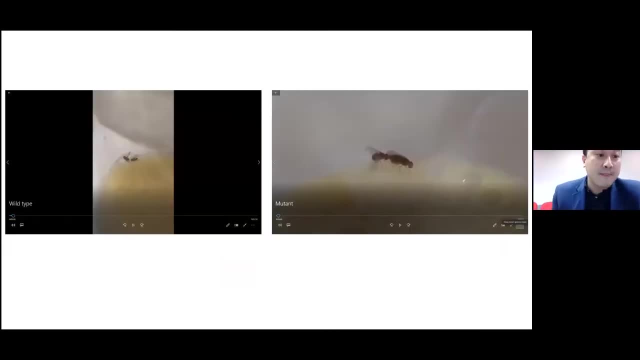 and see how they can actually relate to the regulation of the development. So this is a microRNA cluster, So they have many microRNAs. I'm not going to go into the details. I want to show you one very interesting thing, I mean, which is the video over here. 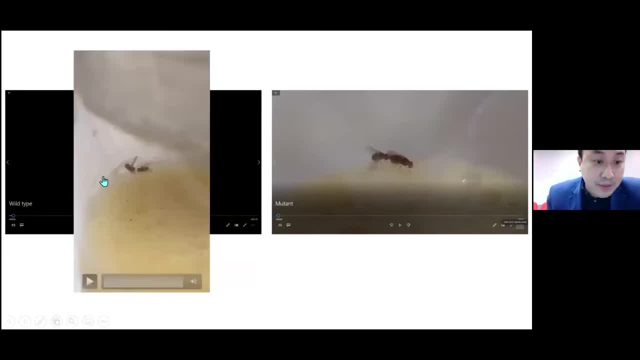 So let me try. I just click it right. So, if you? if yeah, so what you see? so follow my mouse cursor. this is the one with the back abdomen, it's the male and this is a female, okay. 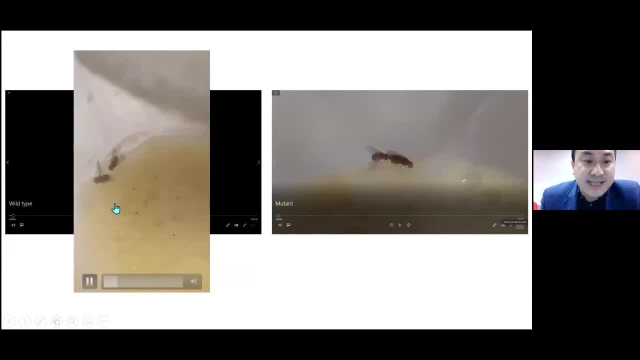 So usually the male chasing the female and try to ask for caution behavior. So of course it keep chasing. And what is it using? It's actually using the front pairs of appendages, the legs, to grab the abdomen of the female. 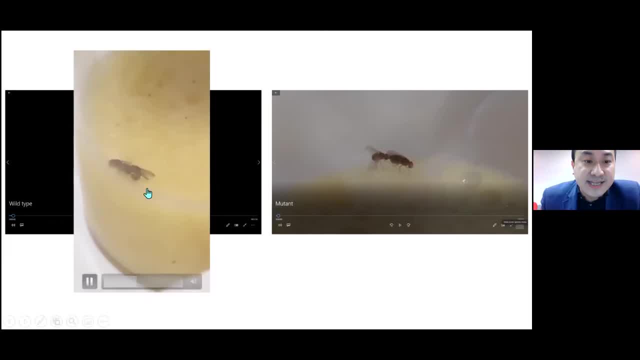 so that they can. you see they're beginning to touch and then you see they're going to do a copulation. So I'm not going to show too long, But when we have the microRNA, in this case we have the mutant. 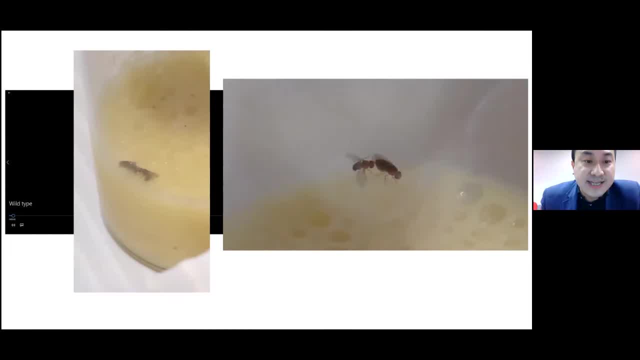 So the appendages, the legs of the flies, are getting shortened, And once they get shortened, you see this, they cannot actually hold their legs and grab the abdomen efficiently. You see, this poor guy, I mean, I just wanted to show you a very long movie. 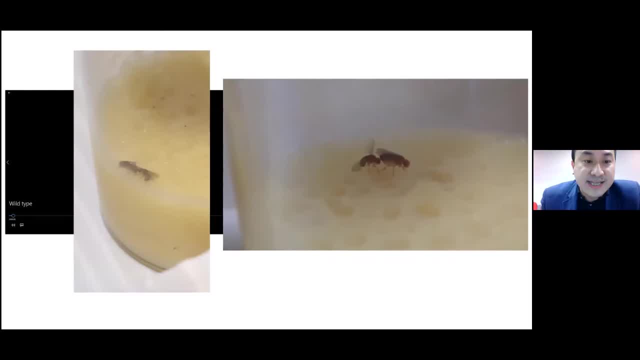 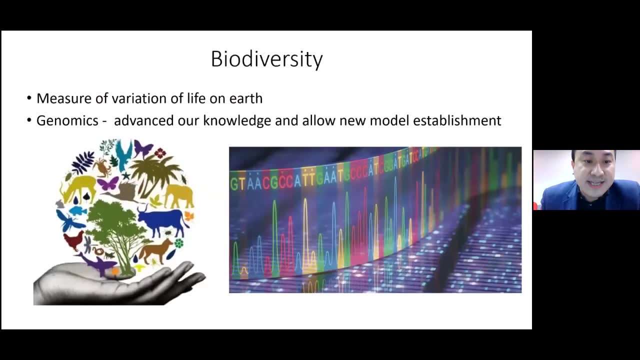 They try to touch. you see, it's not going to be efficient in this case. So what I was showing you is that, in the biotechnology side, what we are trying to do is to we also want to control the insect numbers. 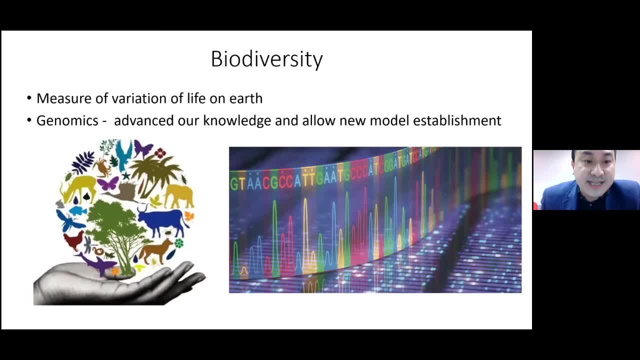 We also try to develop new generation of insecticides, But this kind of- you know- insecticide is. so the way that we try to do is to look for developing new type or new generation of insecticides. to watch, the insecticides will be targeting specific species. 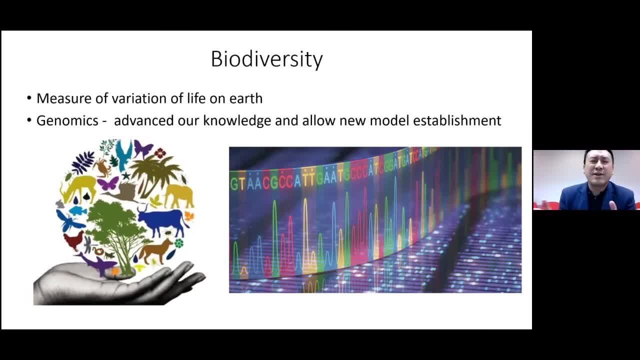 rather than discriminate all the insects or even anything, something not even including insects or fish, et cetera. So we have been using a typical model for fly, because it is very good, genetics model Foot fly. only only it fruits, right. 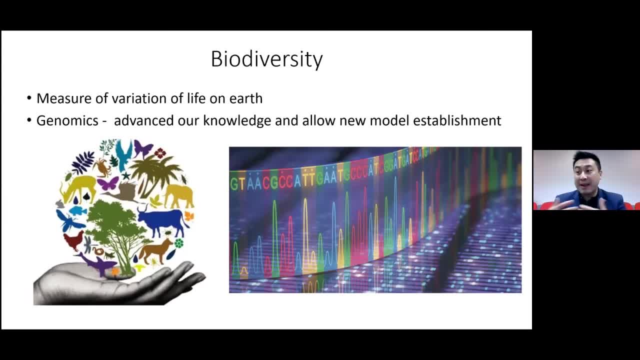 I mean so it damages fruit. Some people think they also damages of wine, for example. But but talking about biodiversity, there's so many variation of life on earth, So can we actually use our techniques to also do them on other types of insects or crops? 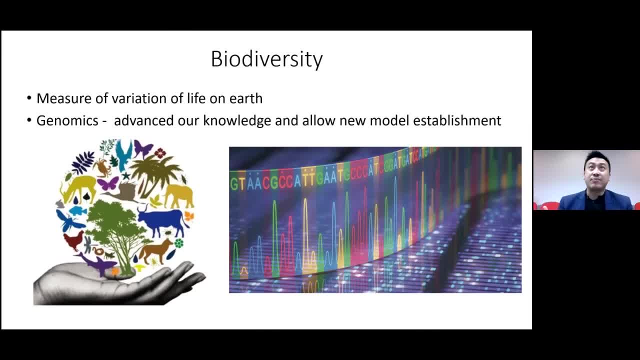 or other things that we will be able to do. Well, we're fortunate. we are in an era of genomics, to which previously it's so difficult that the whole world need to focus on fish, to which previously it's so difficult that the whole world need to focus on fish. 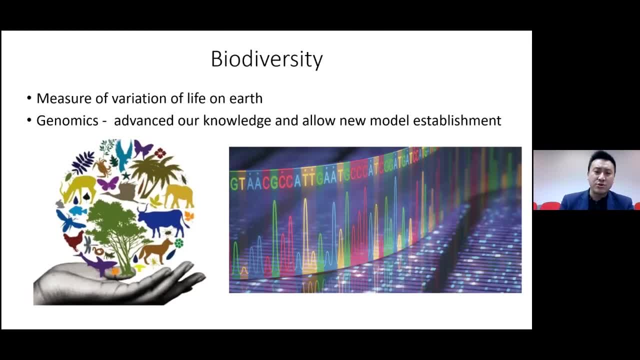 Because we do not have enough people, We do not have enough power. We need the whole world to solve one or two questions together. I think that is reasonable. But now is a time that we can expand a little bit with the advancement of genomics. 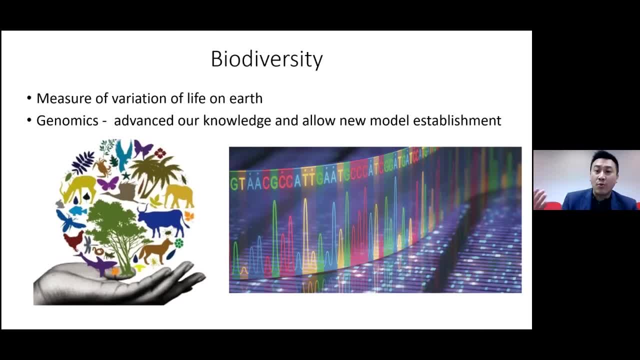 Now we'll be able to get genomes, We'll be able to understand more, We can establish new models, And I'm trying to tell you some of the things that we have been doing in the lab. Of course, I mean because of the man sitting next to me here, okay, 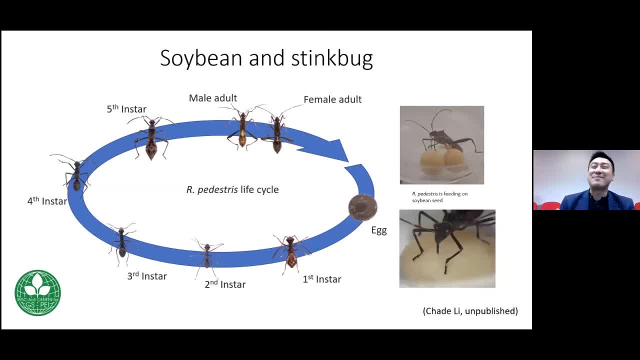 Professor Lam, I mean. So I think, okay, if we want to develop a model, what shall we do? okay, We have someone keep on persuading. you say, oh, soybean is the best, okay, So well, okay, yeah, it's very good. 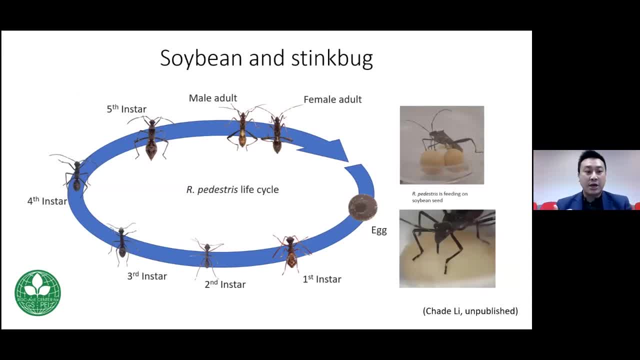 Of course it's a good model. We spent several years together. Of course, I mean we're very lucky- with the support of his area of excellence center. So we have been trying to develop a new model on the stink bug. 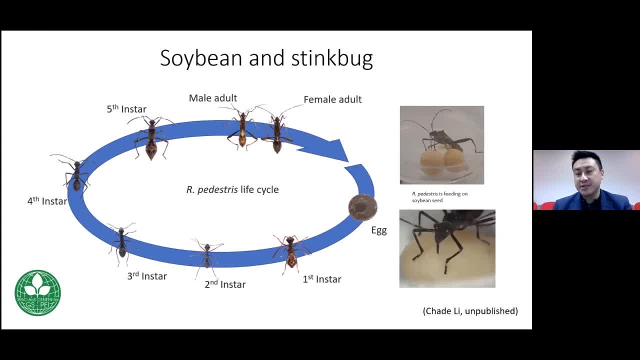 When many people think about soybean, I mean many people think about, you know, soy beans Atheists. of course, atheists are important, But, as I've said, when, under the climate change, what people are seeing right now seems to be: 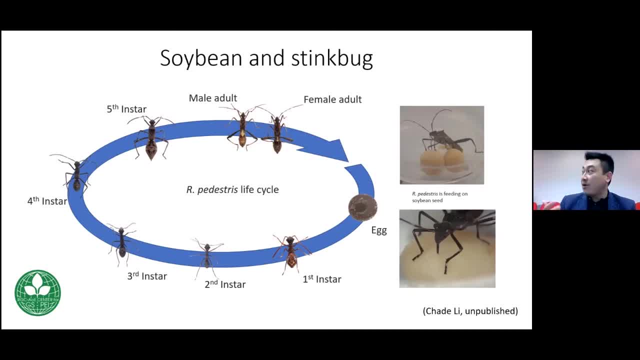 an increasing numbers of stink bug, Our collaborators and friends elsewhere, for example in Korea. what they've been thinking is that traditionally, when you try to target stink bug, it's easy, because you spray insecticides. They're usually very, very dumb okay. 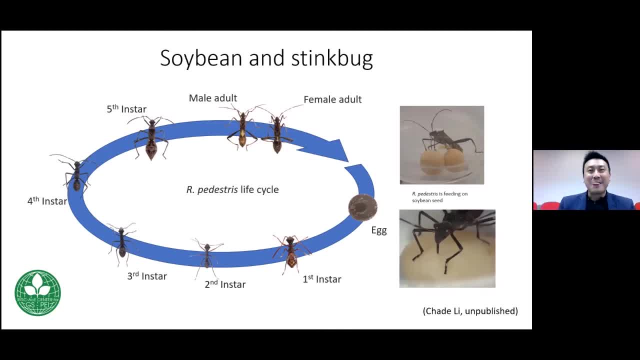 They are there, get the insecticides in eye- okay. But you begin to see this kind of thing by coming in, which is, when you spray the insecticides they fly away, okay. After the insecticides they come back, okay. 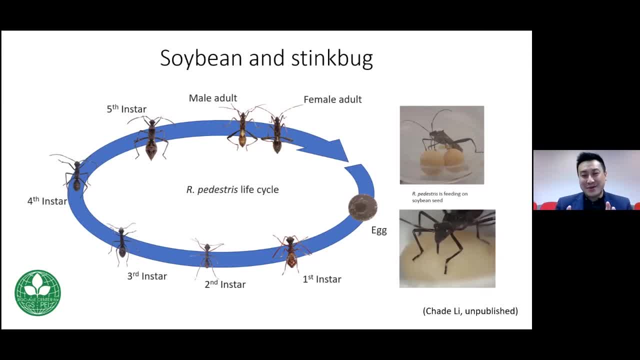 So this has been a new issue that we, or the soybean field, has been facing, especially in Asia. So we need clever ways to do that. I of course I won't speak more. I mean, I want to leave the room. 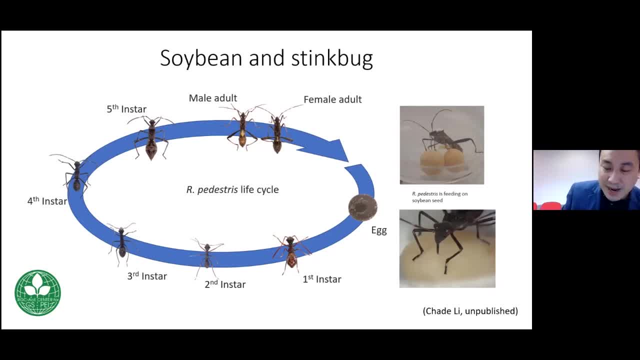 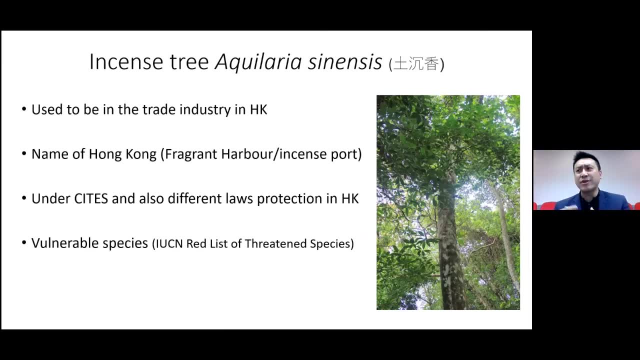 So I'll stop it here. That's my, That's what we're doing by our student, Richard Cha-Dong, So I want to show you something else, which is something we're doing In addition to agricultural crops. can we also think about something else in plants? 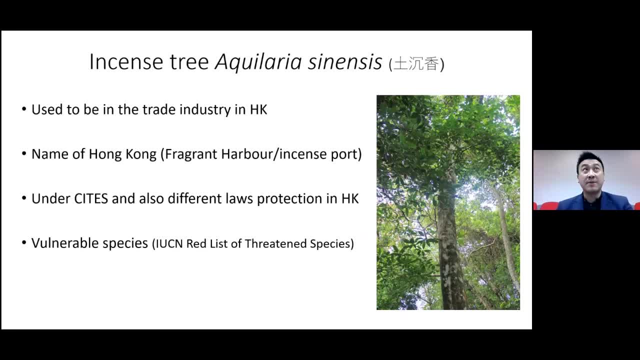 that we'll be able to do under genomics, And I want to typically bring out this species, which is incest tree, echolaria sinensis. That is very, very related to Hong Kong, because that is the name of Hong Kong come from. 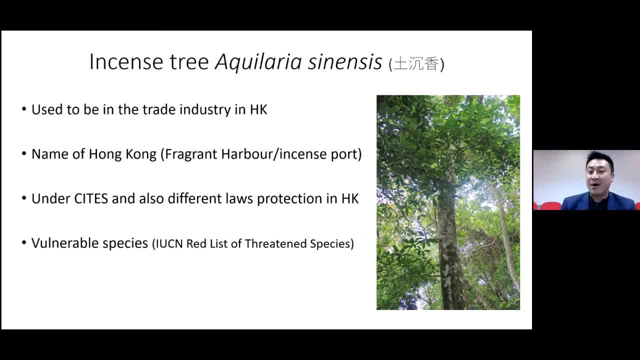 Many people believe Hong Kong we call fragment harbour or incense port, because Hong Kong used to be in an industry or trading incest tree throughout the world or at least in Asia. So it's now. this tree is now under cities and also under different laws protection in Hong Kong. 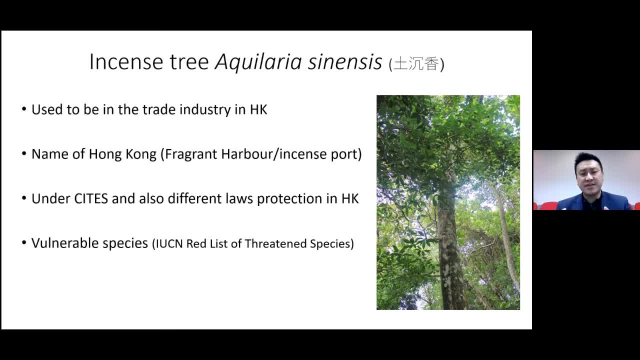 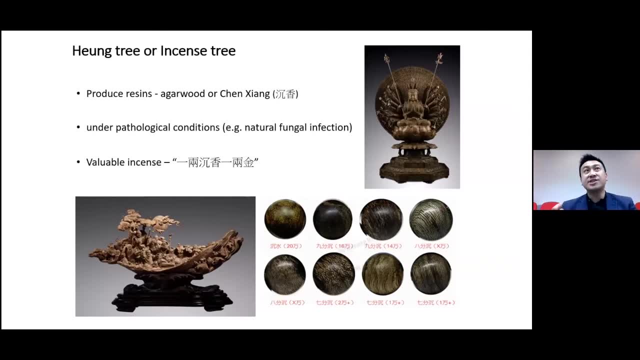 So it's a fraction to unibold species either. the IUCN red list And one major reason that incest tree has been getting a lot of attention and people actually do illegal fouling of those- has been because incest tree can actually, when they get wounded, they will produce vaccines. 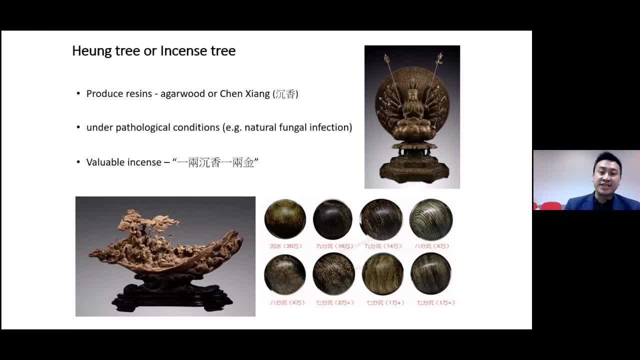 And those vaccines are actually what we call in English, agarwood, but in Chinese they call some, So those are actually very, very expensive. Okay, wood products and what people would like to have is actually natural fungal infection. That is fine, because that is actually a natural process. 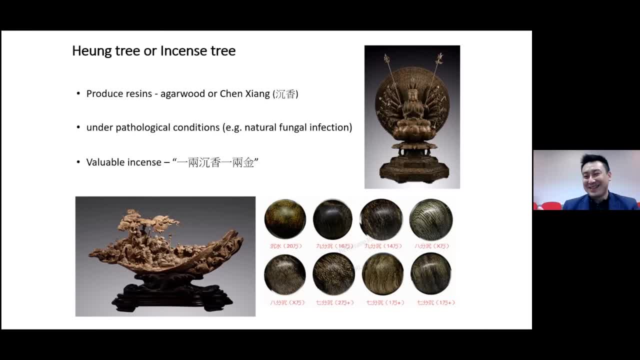 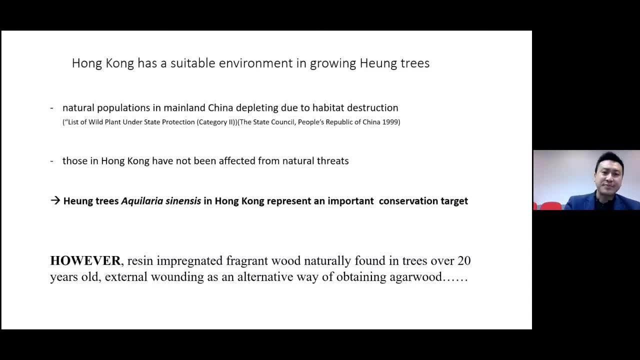 But well, I mean there, of course, I mean people they want to do fast-weights, which they fail to treat the wound, so that has been very, very dangerous Under climate change. what you'll be seeing is that. 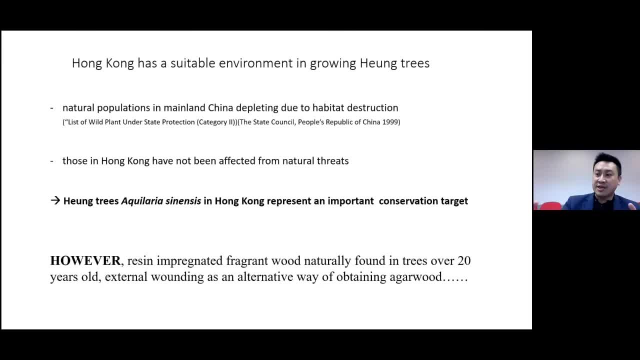 well, the southern part of China seems to be. of course, they're trying to grow a lot of incense tree, but at the same time, well, the habitat seems to be shifting. Hong Kong remains a very, very suitable environment in growing incense tree. so the natural populations. 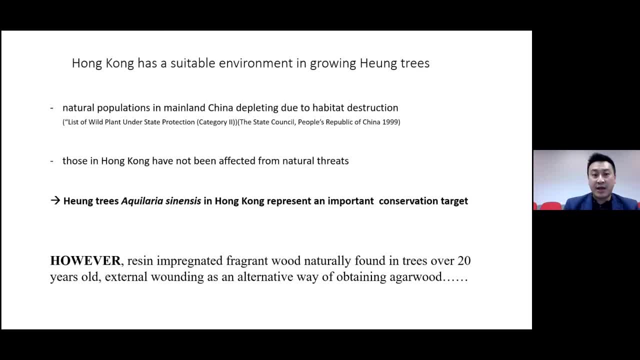 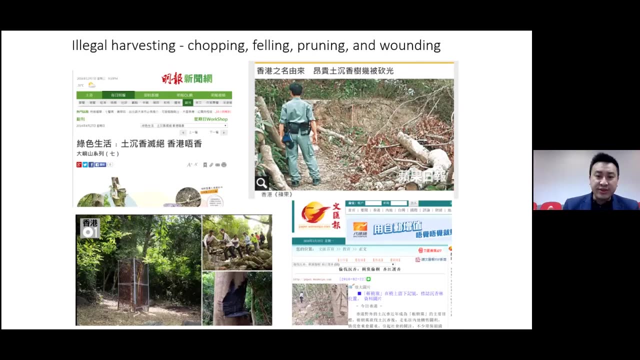 in mainland China have been depleting due to habitat destruction. So the one in Hong Kong has been a very, very important conservation group. But we have been seeing news from illegal harvesting in Hong Kong as well, like chopping, felling, pruning, wounding et cetera. 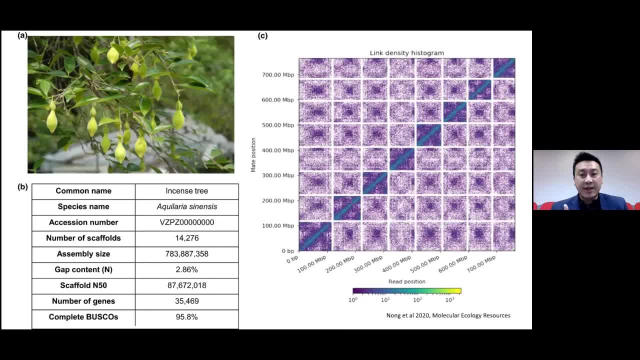 So this is the work that have been done by, and also Sean Law, in the lab, I mean. so, of course, this is also a collaboration together with our herbarium at the Chinese University of Hong Kong. So what we are trying to do is we want to use genomics. 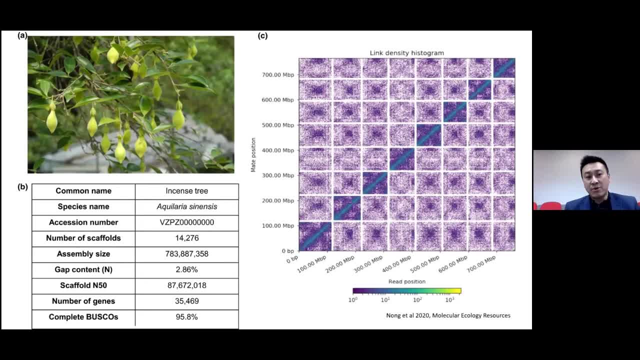 to see whether we can actually help. For example, I mean now we have published the genome coming from Hong Kong and what we're trying to do is to look for. can we actually identify every single tree, For example, when people cover, and we actually see? 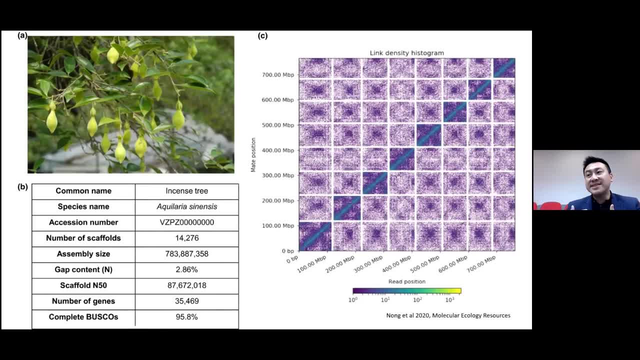 oh, this is actually coming from this area. or when we do compensatory planting, which is we want to plant trees, I mean, in a similar geographical area, can we be planting trees that are with similar habitat types, so that that will be causing less destruction? 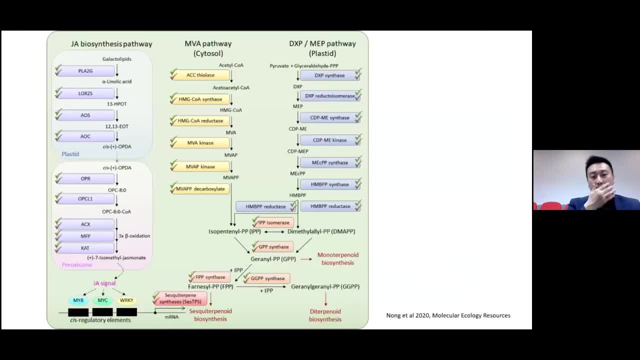 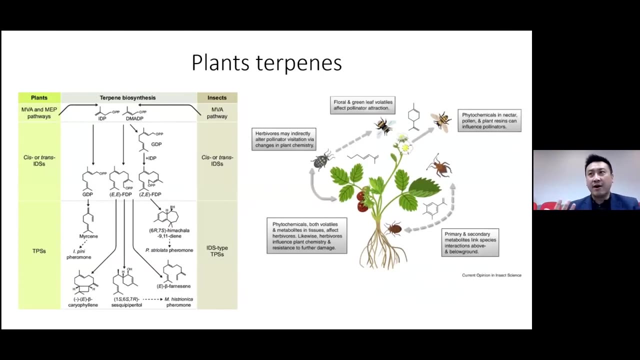 to that particular ecosystem, for example, And of course, we have also identified the pathways so that they will be able to produce terpenes relating to the incense. But, as I've said earlier, I won't. we are a group of zoologists, etymologists. 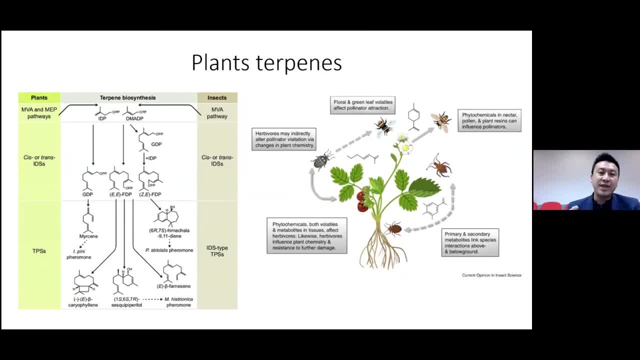 so we're working on plants. We of course need experts in plants to work together, But actually there's one interesting thing. we would also like to mention plant terpenes, And I mentioned that insects produce sesquiterpenols, right. 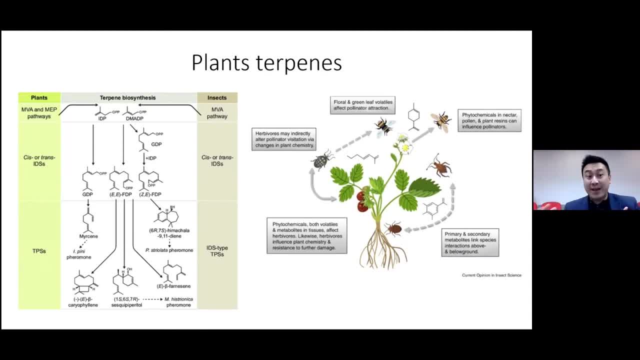 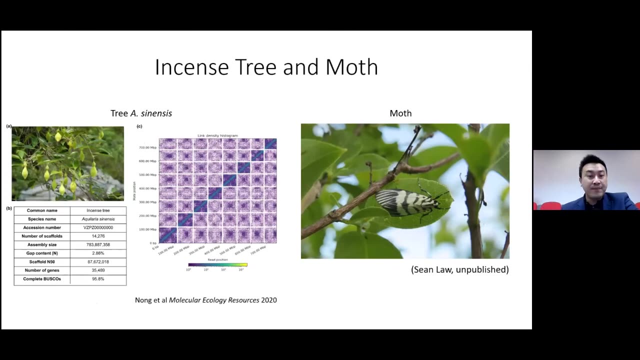 Juvenile hormone Plants also use a very similar pathway and produce terpenes to attract the insects. So this is actually a talking point, a sharing point in between the two, And we have been actually looking. this is unpublished data from a PhD student, Sean Law. 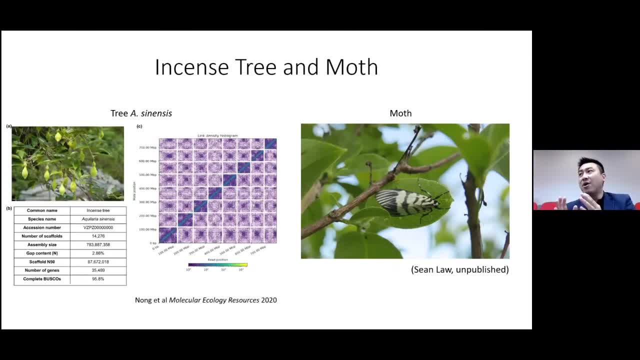 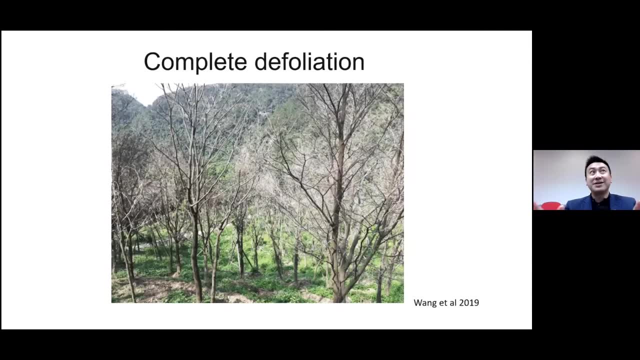 So we've been looking into a moth. okay, This moth is a specialist to which they only target the incense tree And when they're present, you have complete deflotation. okay, You have complete removal, taking all the leaves off your incense tree. 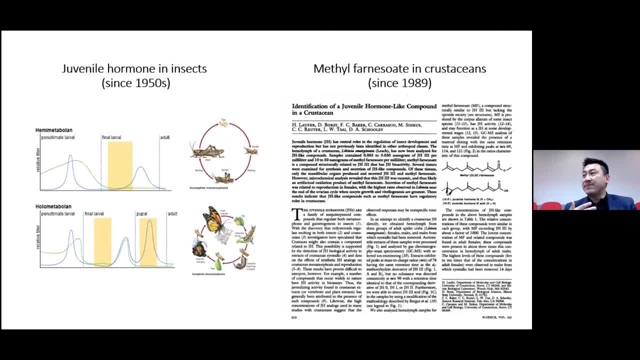 So what I've been telling you from biotechnology we've been doing on new insecticides. I've been using genomics to establish the new model, like together with the soybean, and also we're trying to do conservation, understanding the interactions of other insects. 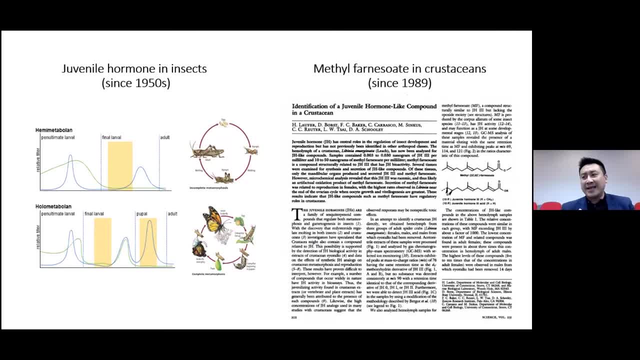 for the incense tree And, as you can see in my topic I said insects and other arthropods. okay, Can we actually develop some new models for agriculture? So come back into the. I only want to share juvenile hormone today. 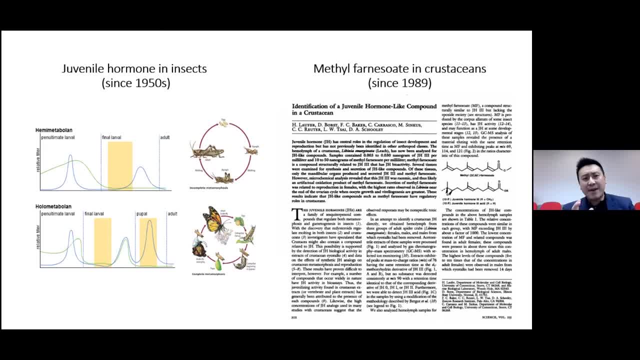 coming back into here, Juvenile hormone has been described in insects since the 1950s- okay, In crustaceans in other groups, mainly in water, maybe not be too related to agriculture back into late 1980s. 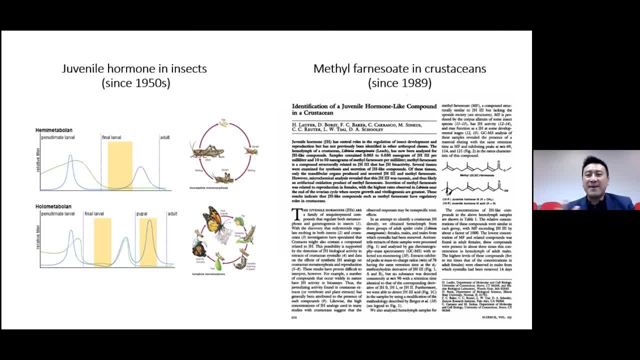 they discovered they do not have juvenile hormone. They have something called newfound, very similar structure. I'm not going to go through that, but I want to tell you what our lab has been doing In 2014,- I think very luckily. 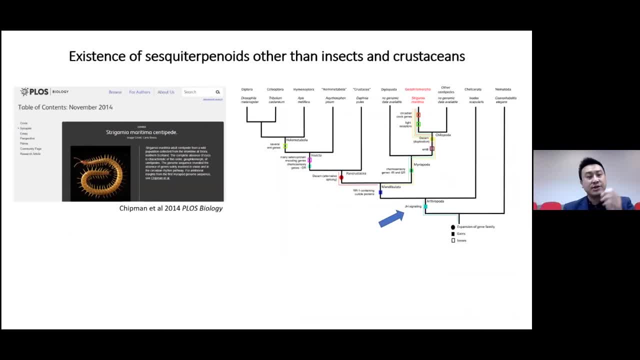 if you understand the relationships for different arthropods- insects- the closest group is the crustaceans like crabs, lobsters et cetera, And the immediate closest out group is called myriopods, That is, arthropods, I mean. 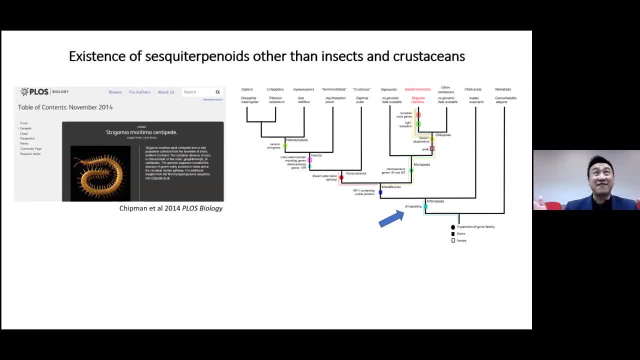 are jointed leg animals. They have lots of legs like centipedes. okay. So the whole world has been doing together. I mean at that time we need the whole world to do one centipede genome. I mean our group has been very, very fortunate. 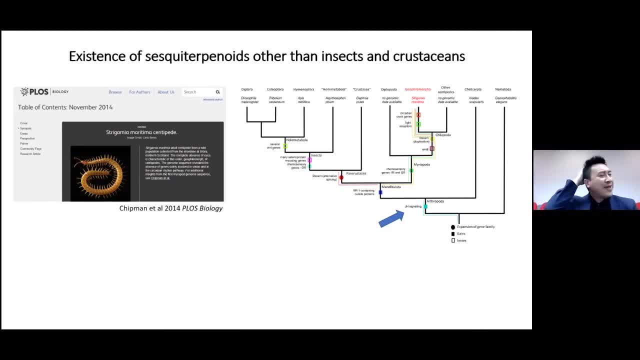 to be involved in this annotation. So when people ask us to do- okay, well, Jerome, you can do- juvenile hormone, I say, come on, juvenile hormone has only been known in insects. I say, come on, juvenile hormone has only been known. 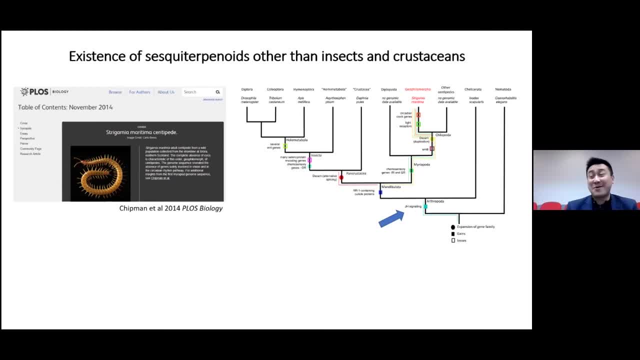 in insects, Maybe also in crustaceans? We never would be able to think that you'd be in centipede. They'll say, okay, it's a global effort. We try it, To our big surprise, which also become a major point of that genome paper. 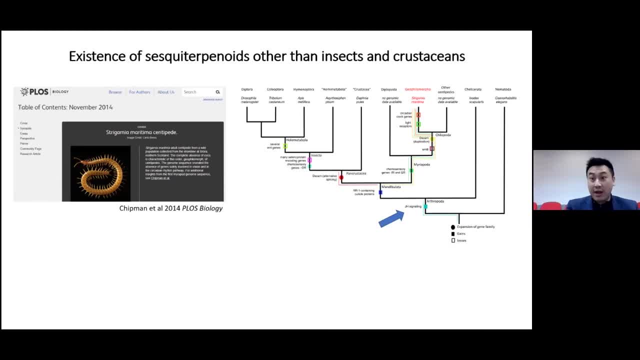 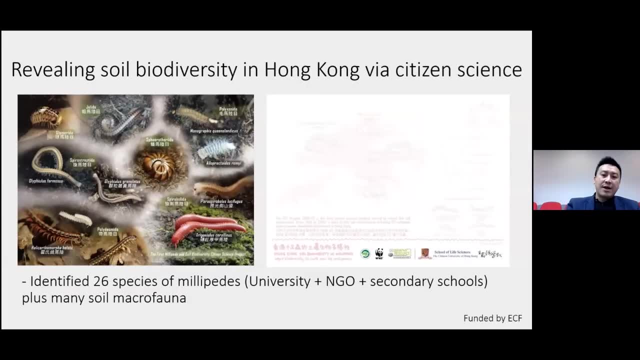 we found that, yeah, actually this kind of system seems to be also found outside in such a crustacean, in centipede, for the first time So recently. I mean, I'm not sure if you're familiar with this. 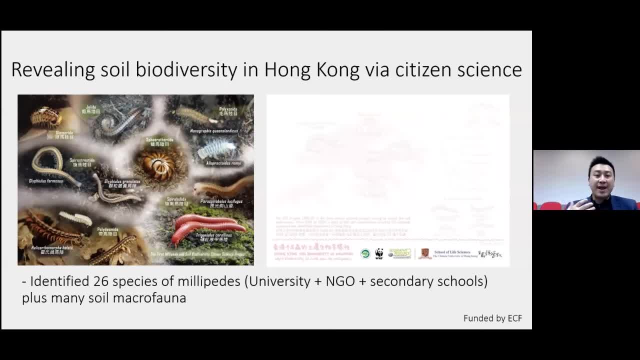 but we have been working with the ECF, I mean of our Hong Kong SEL government, So we have been asking together- I mean, if you can see- sorry, the logo is a little bit small- funded by the government. We do get in together with WWF Hong Kong. 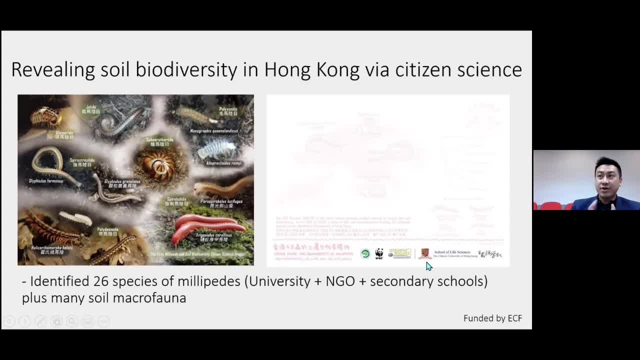 together with the DRM and also our School of Life Sciences and also around 20 secondary schools in Hong Kong. We do not understand how many species we have in Hong Kong. That project that has been finished project we asked the students- I mean together with our staff. 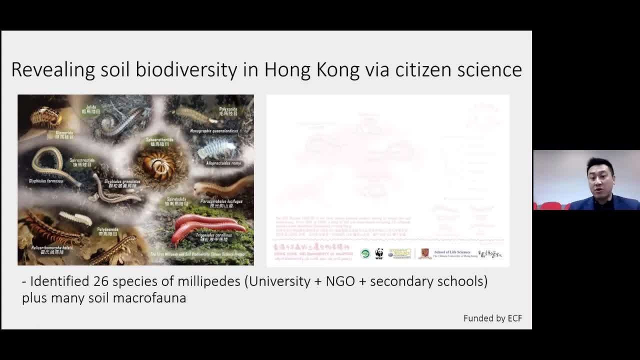 go to the field and try to take out and see what are the millipedes that we have. We have found not only millipedes but the soil macro fauna, all the soil animals. you're able to find Just millipedes alone. 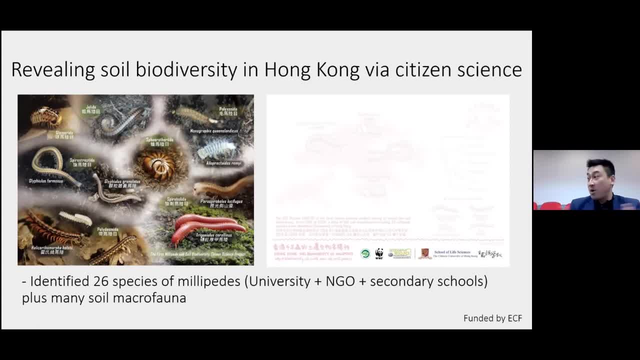 we found about 26 species from Hong Kong. I mean we make a postcard showing you over here. These are the one that we'll be able to find in Hong Kong. Of course, some of them are also shared together with in other places in mainland China or Asia. 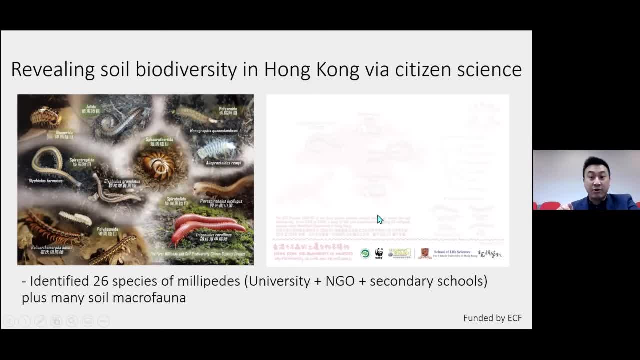 But we seem to find that one, of course, for now it seems to be unique in Hong Kong so far. We also find many, many other many soil macro fauna. I mean about roughly about 200 species, 180, I don't remember the exact numbers. 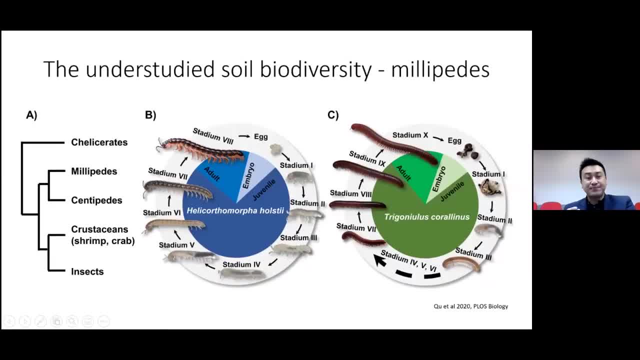 And after we do that, together with the citizen science to do that, we go back, of course, to academics. We want to understand more. So this has been done by Kevin Nong Henry, so in the lab, So we sequence the first two millipede genomes. 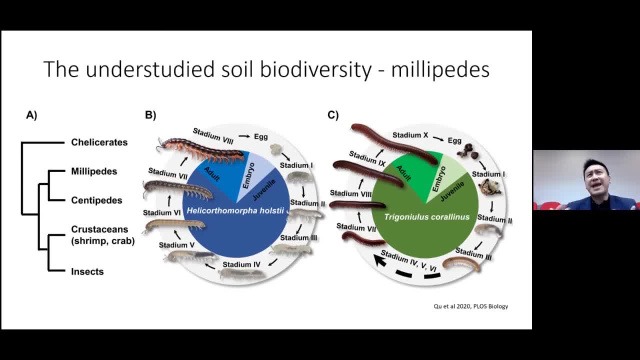 to understand what are actually happening. Can we actually use them as a model? Because when people think about soil animals in agriculture, many people think about earthworm. Earthworm are, of course, important, but many people have neglected millipedes. 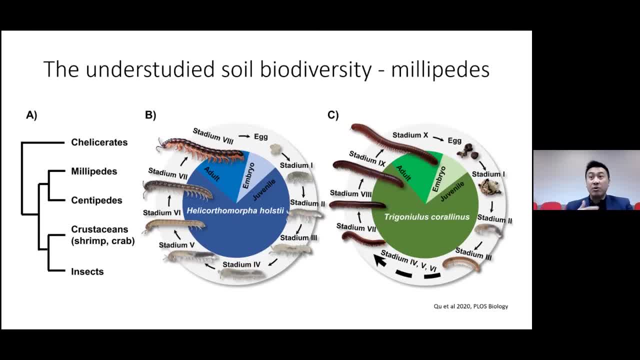 which are actually. if you go to a forest, for example, they are very efficient nutrient cyclists. All the leaf and litter, they are the nutrient recyclers I mean in the system. that has been overlooked, So I'm not going to talk about all the findings. 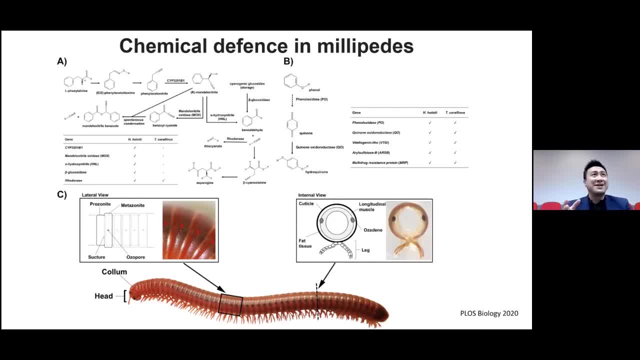 that we have in the millipedes, For example, we are able to find- well, I call a job like a chemical defense. this is random and this thing will produce a lot of like how to cyanide gas and we're able to identify. what are the genes actually? 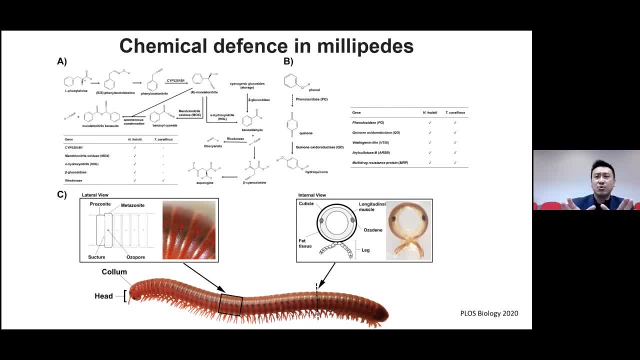 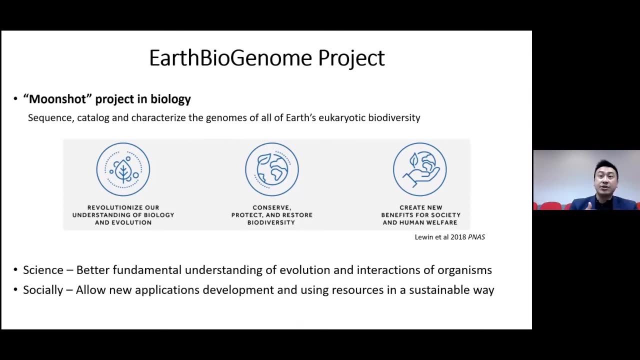 in water, for example. Having a genome allows us to recover and discover what actually the underlying biology and also allow us to wow, to develop new models. Why am I saying that Not only my lab have been trying to do from insects to trying to look for a new generation of insecticide through the regulation of juvenile? 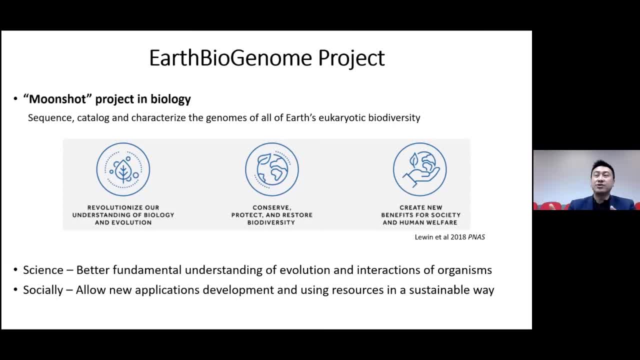 hormone and microRNAs, et cetera, and the development, and also we try to look for new models. I mean plant and insect interactions and also new models like millipedes. Now, in the era of genomics, we for example in UK the Darwin Tree of Life is now proposing. 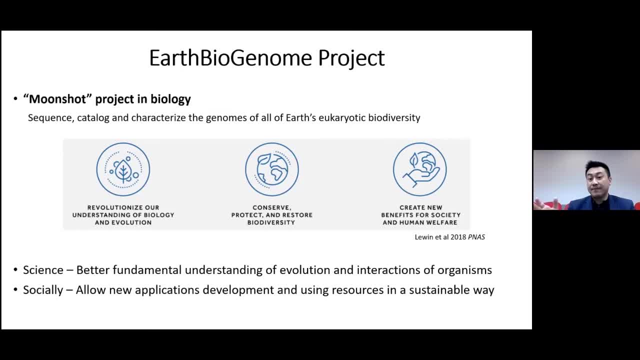 to sequence every single species in UK. United States are thinking of sequencing every single species in the United States. That's been called a moonshot project in biology, So it's like trying to do a very difficult task. I mean in this region, in Asia: EarthBioGenome project. 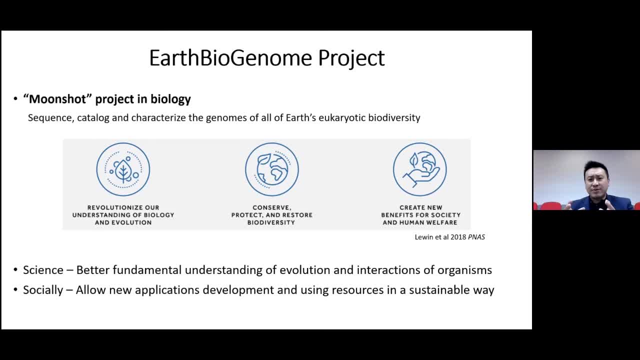 many people have been proposing. I mean, I need to tell you this is not just scientifically important- Science-wise, this allow us to have a better understanding of evolution, interaction of organisms and also the biology- But socially this also allow new applications. 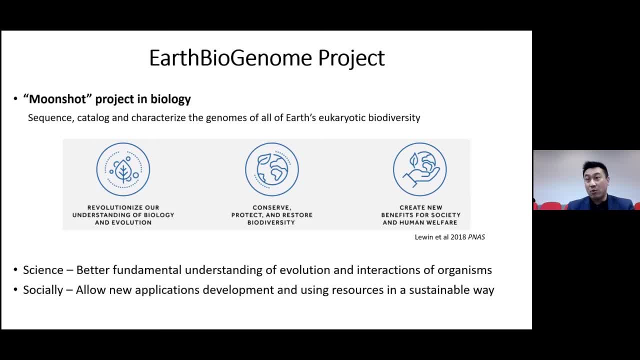 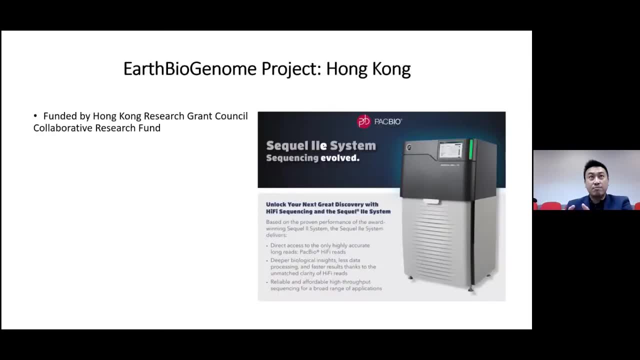 development and also using resources in a sustainable way. So, for example, we'll be able to look: oh, could this be a certain type of population in certain area we need to preserve, et cetera. So, the EarthBioGenome project: we are trying to launch a project of EarthBioGenome project. 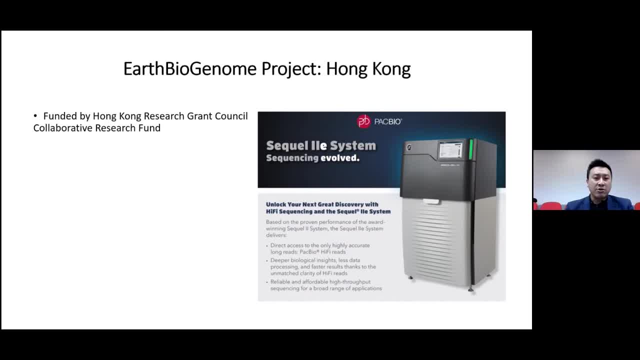 in Hong Kong And we are very, very grateful to the Hong Kong Research Grant Council Collaborative Research Fund. We are going to get the first system of our SQL2E system. Don't worry about the name. This is the system that will allow you to do genome sequencing in a very, very 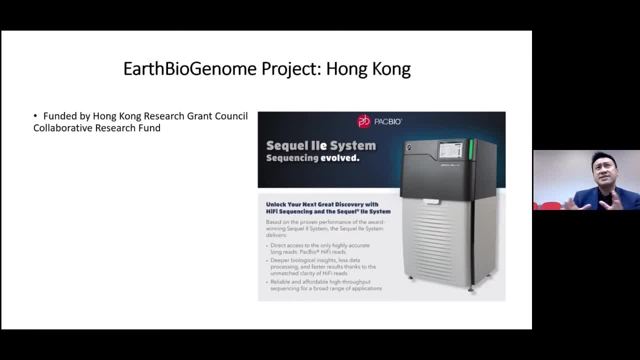 efficient and massive way. So we want to sequence the genomes in this region And we are going to launch a campaign later and also ask the citizens to give us suggestions. What would you like to know? Genomes, maybe will be useful for you to know. okay, This is something. 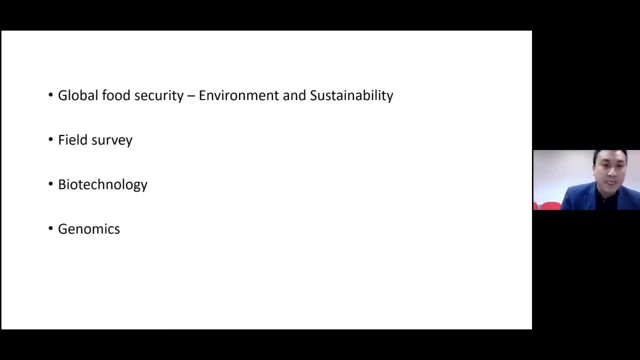 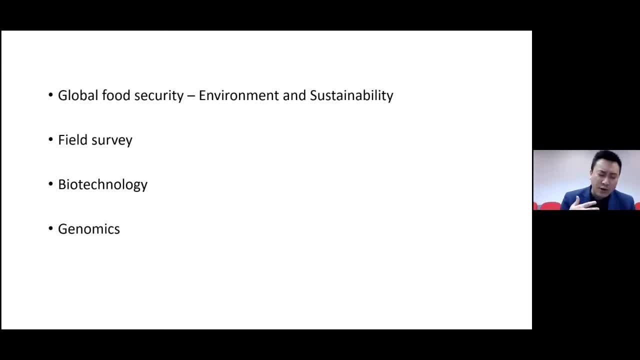 environment and sustainability, And I hope you agree or get convinced that insects and other arthropods actually play a very important role in addition to the plants itself, And their interactions are very important. I've shown you about a field survey that we have done in Hong Kong. 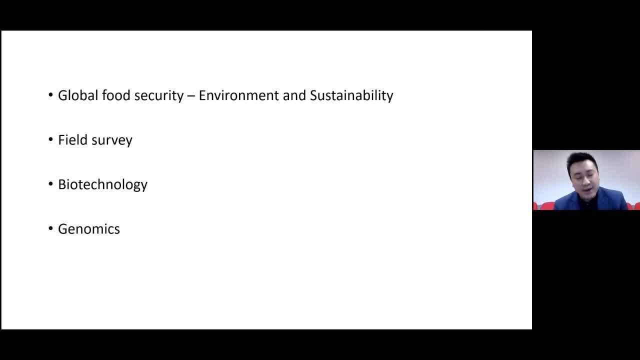 to better understand the insects and also other micro fauna, no matter in the soil, the insects, the pests and the beneficial insects. I've been showing you the studies in my lab going through the biotechnology from using microRNAs, genomics, et cetera. 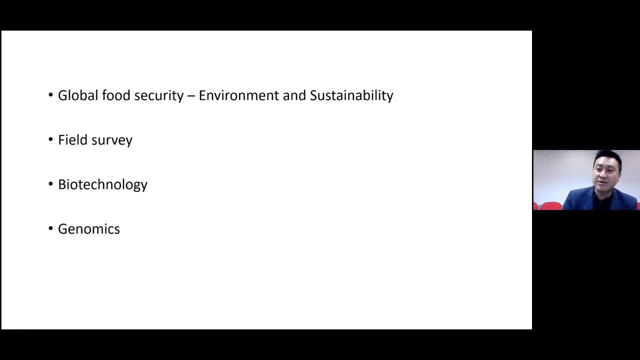 to better understand their interaction, to develop new generation of insecticides, how we can do together with the plants, And also we are trying to see if we can understand more from this region by sequencing more genomes. But that of course I need to thank. 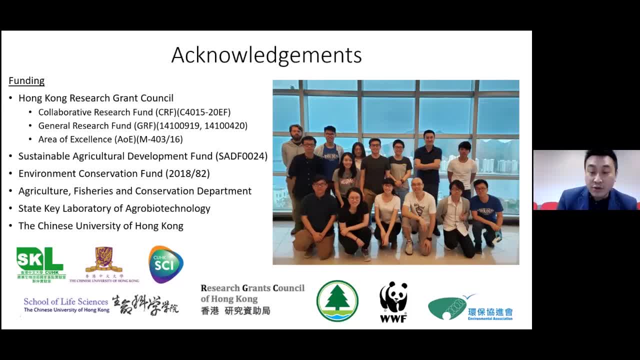 I mean this. I cannot do this by myself. I need to have very good collaborators. I mean, including the one sitting next to me, Professor Lam, and also many good friends. I mean TF Chan, many people in the AOE, et cetera. 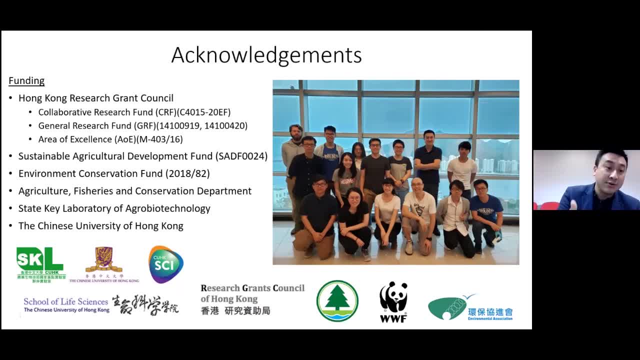 You know, I also need to thank our Grand Council, Hong Kong Research Grand Council, Sustainable Agricultural Development Fund, ECF, AFCD, our Stakey Lab at the Chinese U and also, of course, my university and our School of Life Sciences. 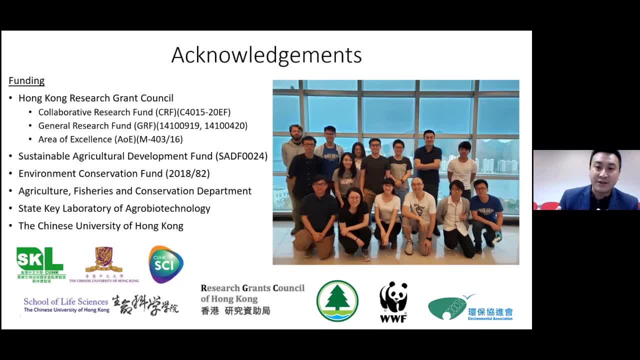 Now, mainly, of course, I personally. I really need to thank the group members that I have in my lab to do this fantastic work. I mean, if that's good, it's because of that. If something is bad, it's because of that. 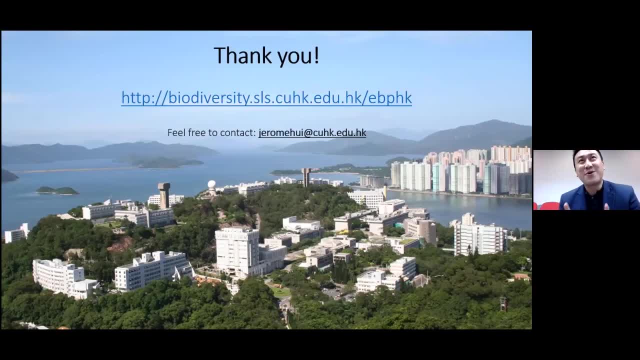 Because it's me okay. So that's all what I want to say today. If you're interested and find out more about what we have been doing, we have set up a new website. I mean this link. There are many different projects. 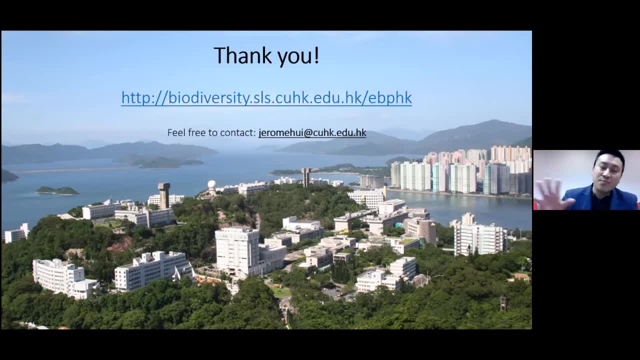 There are more introductions on that website. You can look into more details. Of course, if there are questions that you may not be able to answer today and you want to ask me, feel free to contact me at this email. And this is, of course, our beautiful campus. 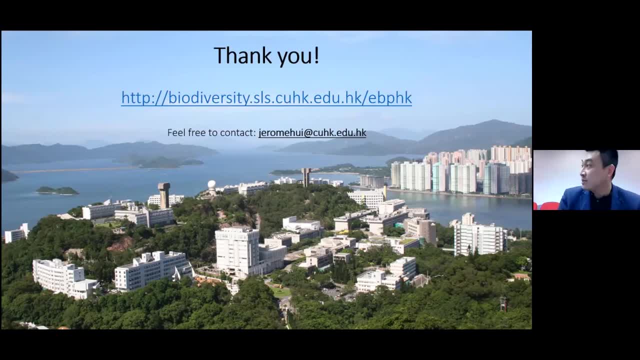 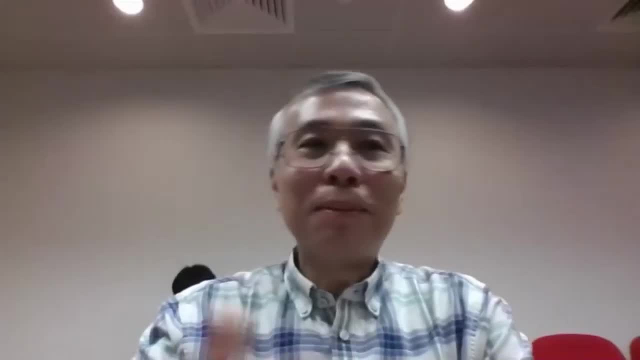 And again I thank you for the time for listening. So if you have questions, you're welcome to ask. Okay, Thank you. Thank you, Jerome, Before we take any questions, so I suggest us to take a group photo. 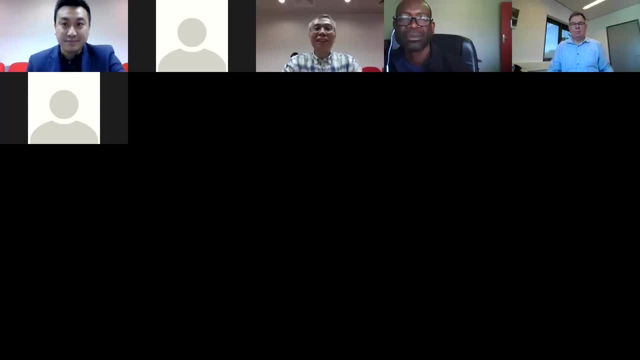 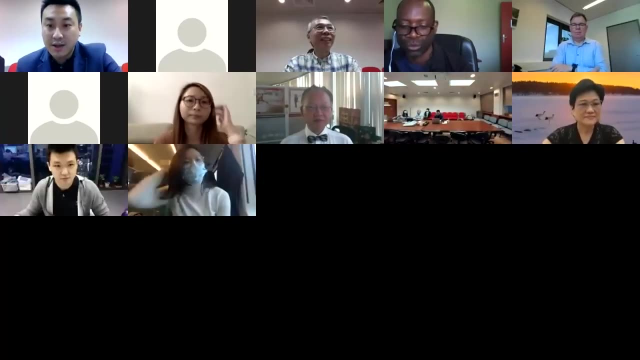 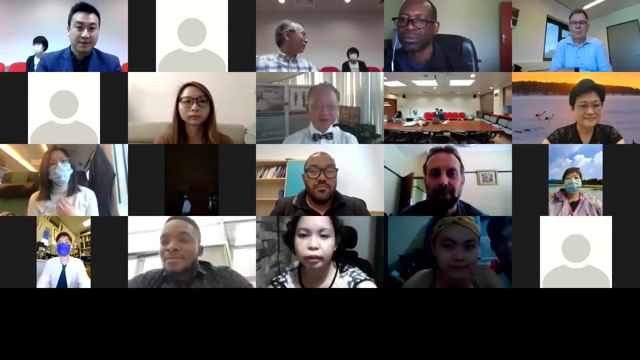 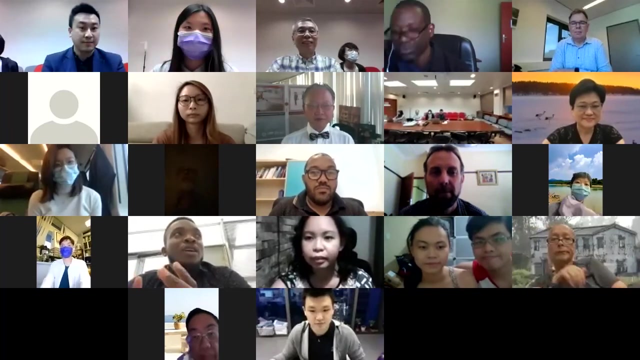 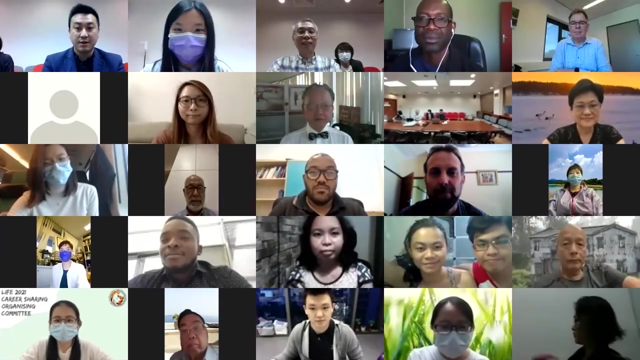 So could everybody turn on your camera and, if possible, remove your mask so that we can take a photo together? So let's just sit here, yeah, Okay. so, Joanna, please help to take the photo. Okay, we look at the camera and look at the field. 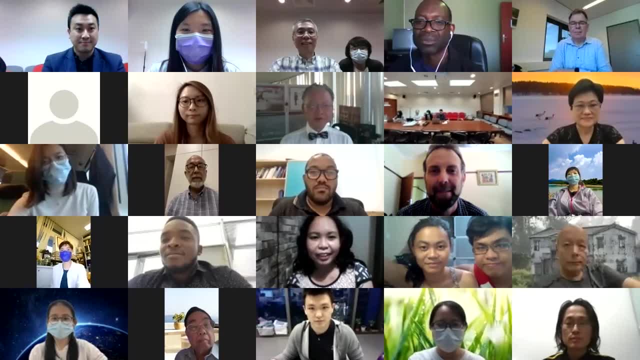 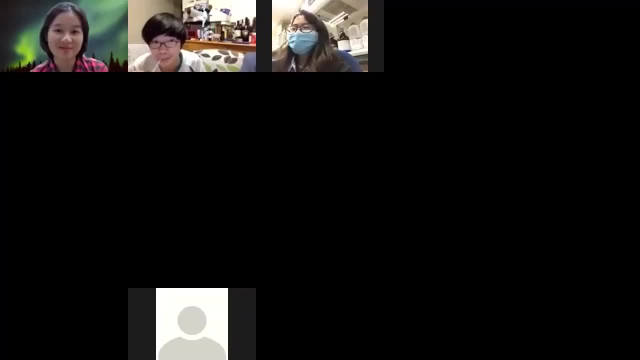 First: one, two, three, Okay, we'll take one more. One, two, three, Okay. one more One, two, three, Okay. great, Thank you, Okay, Okay, so well, I guess the biodiversity of insects. 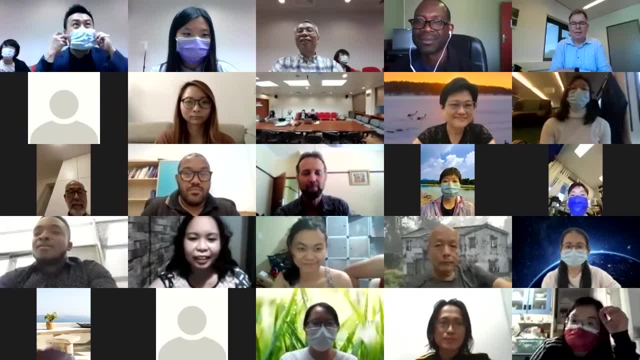 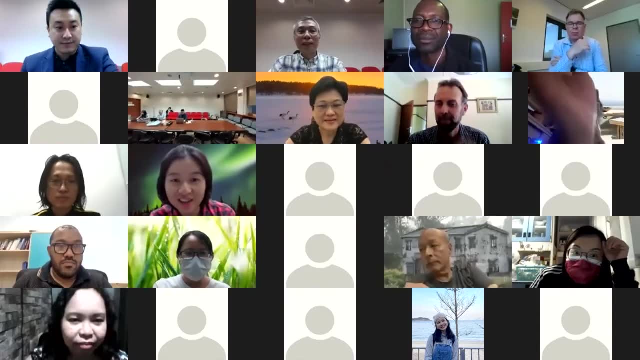 play an important role in sustainable environments. Of course, we have worked in agriculture. We always think about pests that will destroy our crops, But insects could do a lot of good things to us. So I think it's important for us to think about. 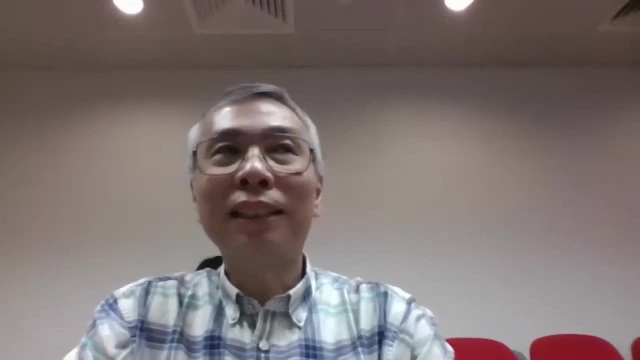 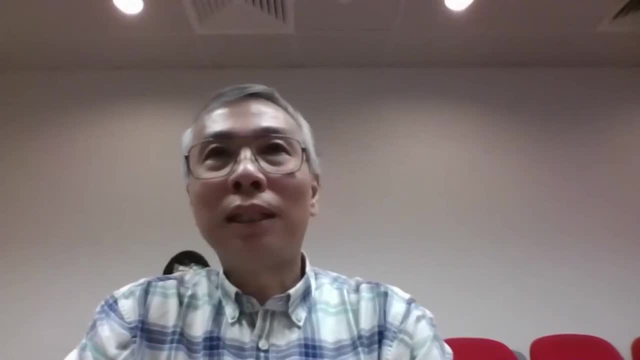 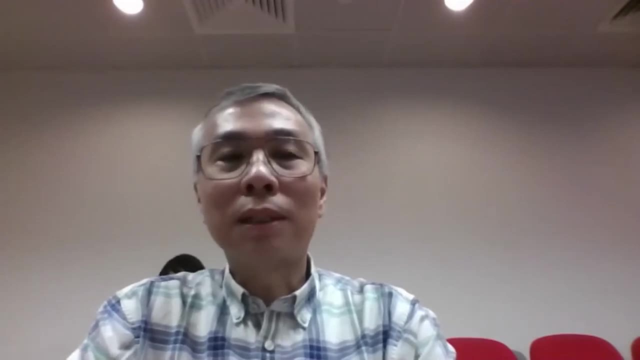 we do know that an effect of an insect's pollination. it's very important to maintain a healthy population of insects and understand how it interacts with plants and crops, And Jerome used the state of the art genomic technology to investigate such a system, as well as doing some mechanistic studies, including the development and the juvenile hormone, et cetera. 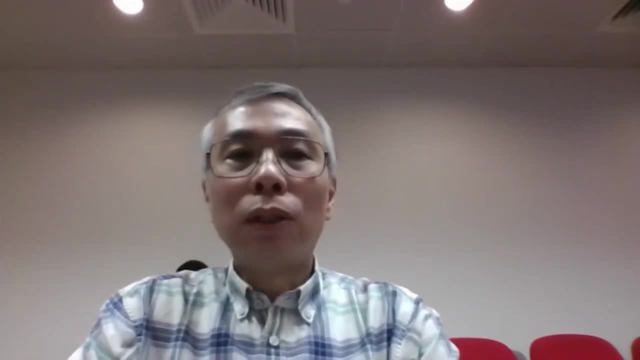 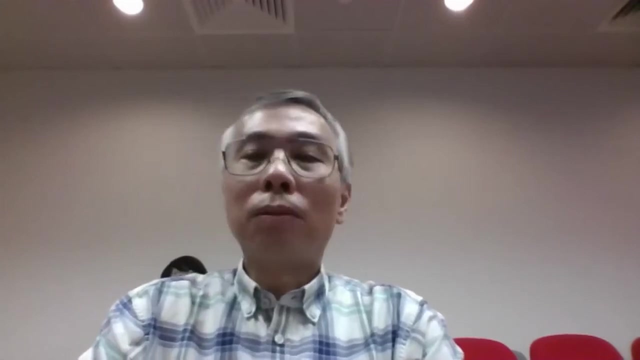 So I think that's very important. it will give us a tool for agricultural biologists to think of how we can plan a sustainable agriculture. So now the floor is open for questions and discussions. so whoever would like to ask a question, please unmute yourself or you can type. 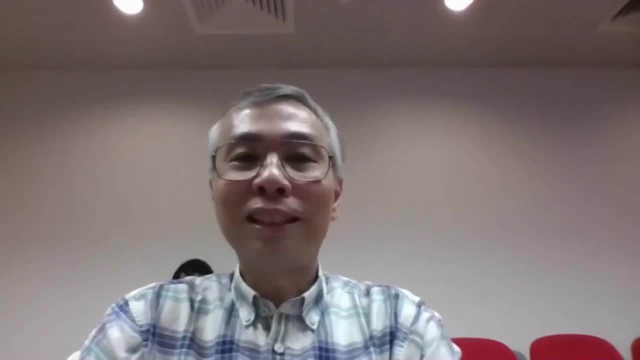 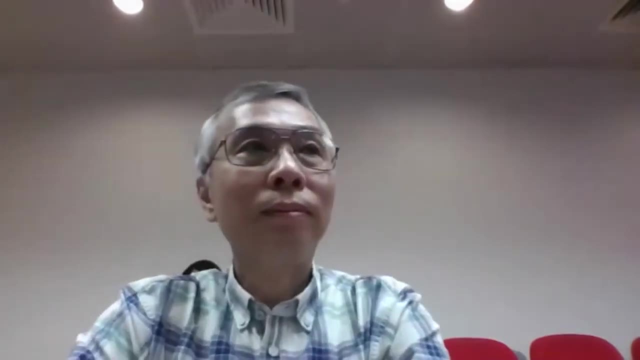 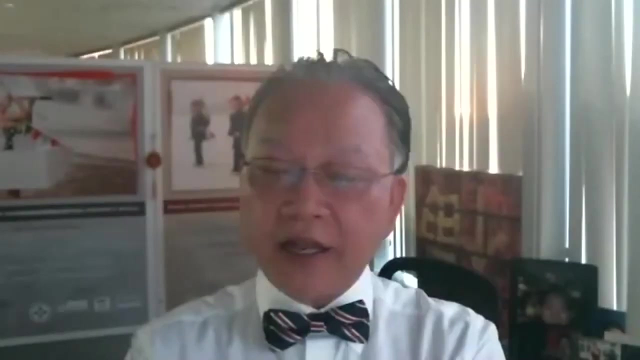 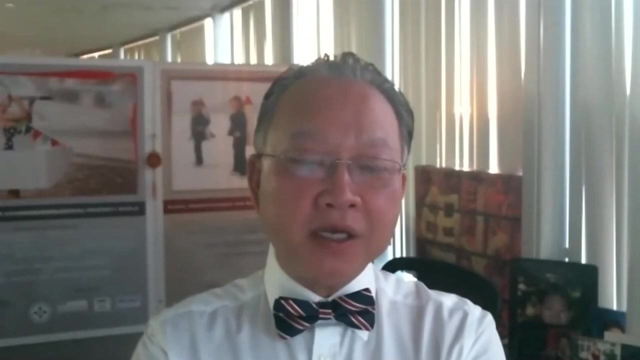 it in in the chat box, so it's now open for Q&A, please. So this is Kit Chan, right? so in 1984, I was being sent by my mentor to go to Texas A&M. So what we what we see is that I follow the professor MD Summer. 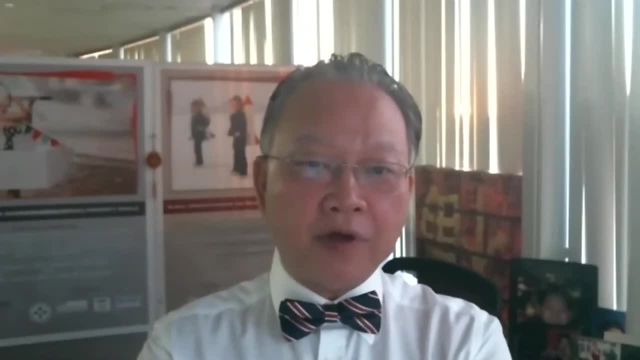 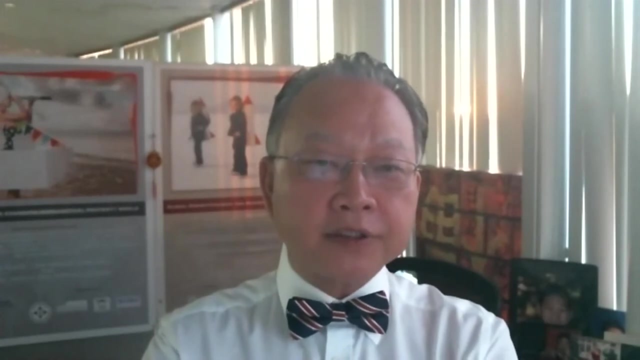 He said, actually at A&M they have a department of entomology, So at CUHK I learned all these insects from Chong Shui Zhang. so, Professor Zhang, But anyway, I guess my question is that at that time baculovirus is a polyhedron gene. What? 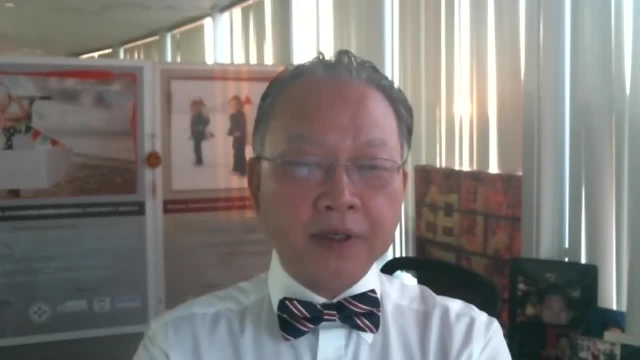 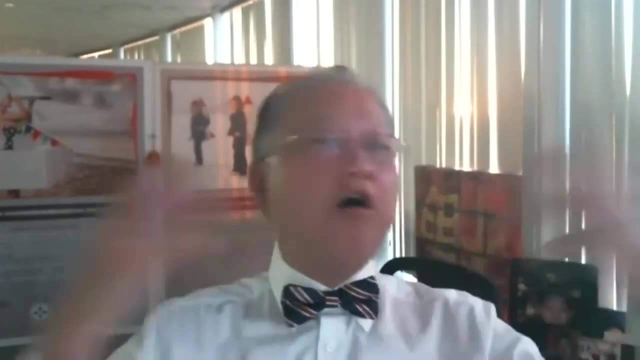 do you really see in the global landscape how all these wonderful insect study would have a major impact in the agriculture? And now of all these studies? what do you see in the global landscape how all these wonderful insect study would have a major impact in the agriculture? And now of all these? 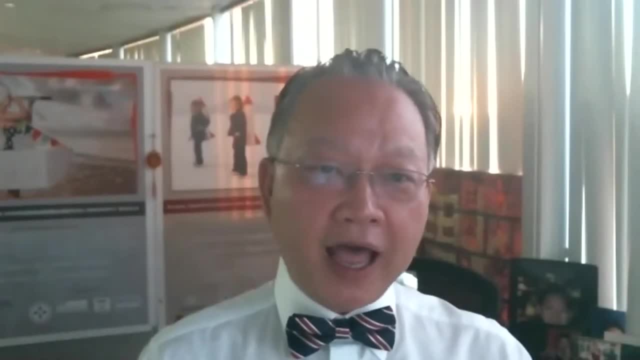 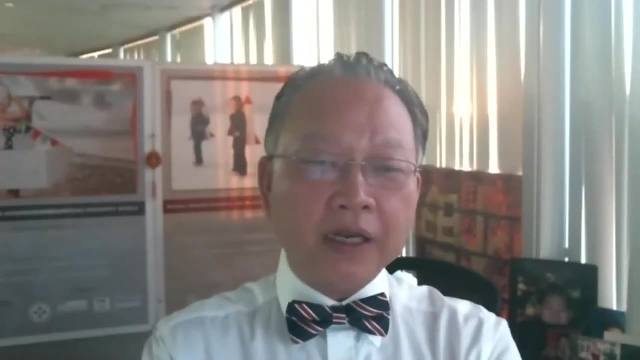 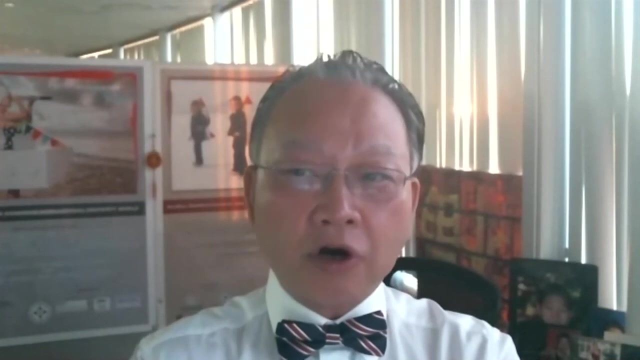 different insects. which one would you pick have the highest potential? So that's what a global perspective From the locality. it's very admirable when I see your slides about all these like worm and you motivate the high school kids. So I was growing up in new territory and I'm fortunate enough and 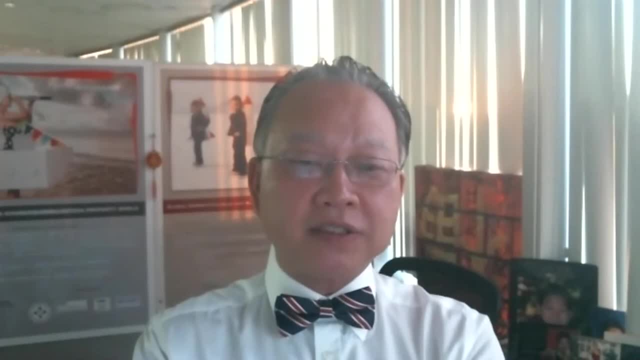 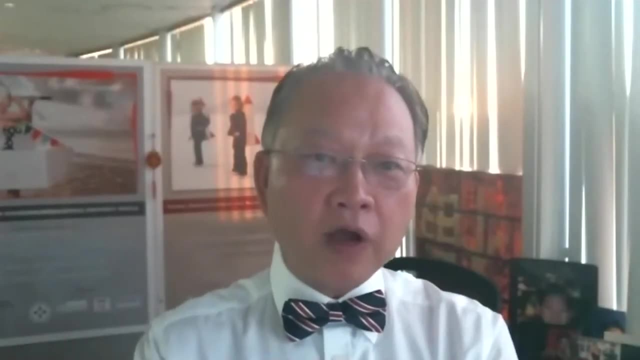 go to my backyard, I take up the soil, I see the earthworm, I see all these different stuff is, to me, is fascinating. One word is fascinating: habitat and in the local environment. what would you really propose and how do you promote it? and how do we really popularize and make sure that our kids, our next generation, 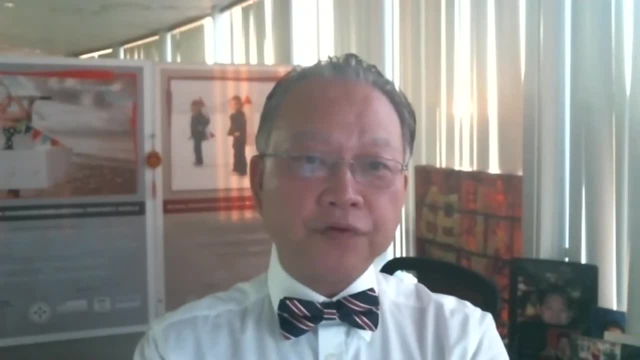 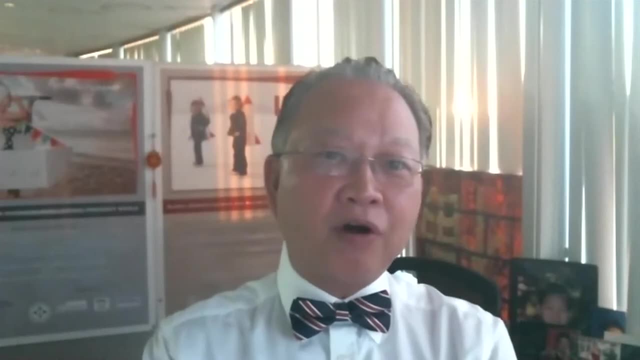 would learn how to appreciate the importance of insect study. When I was in CUHK- I was I was focusing on the microbiology. I was really for the people work on Chong Shui. I would say that it's a low cost science, but as I gradually 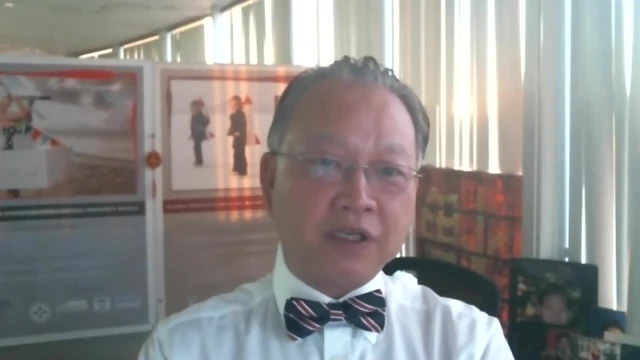 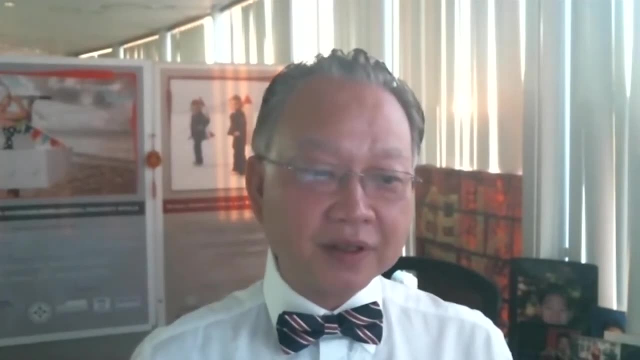 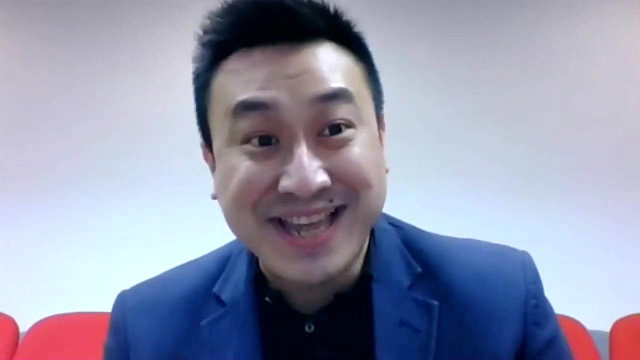 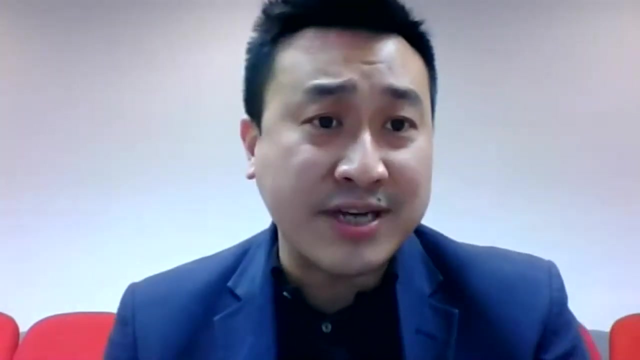 growing up I just really know that, how wonderful, wonderful this living organism and its impact of human to mankind. So thank you. I mean, of course, I couldn't agree more that they're very important and they're fascinating and they are going to bring a new enlightenment for our new generation. So I answer your second. 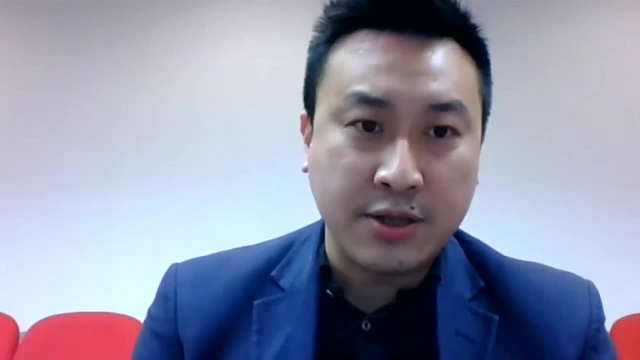 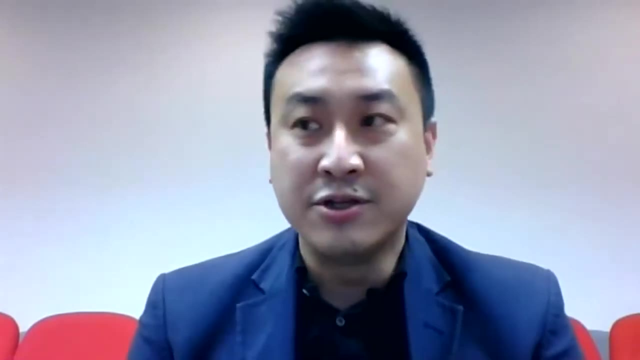 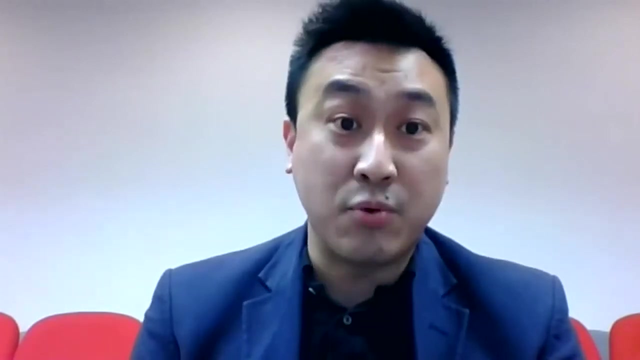 question first, which is how we are going to provide, how we can arouse the interest of the- of the students- I mean themselves, I think- throughout the survey that we have. I mean, I think, get them engaged. it's actually very important because, well, I actually we need to write a report, right, because we have 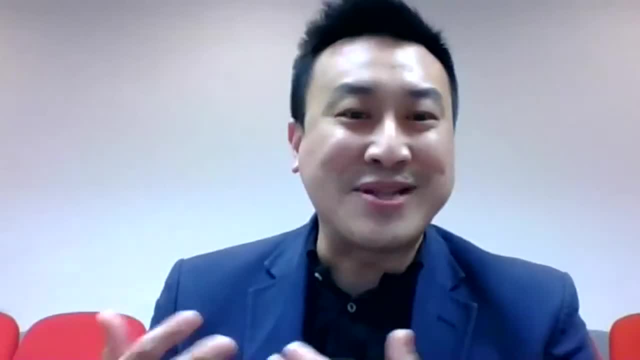 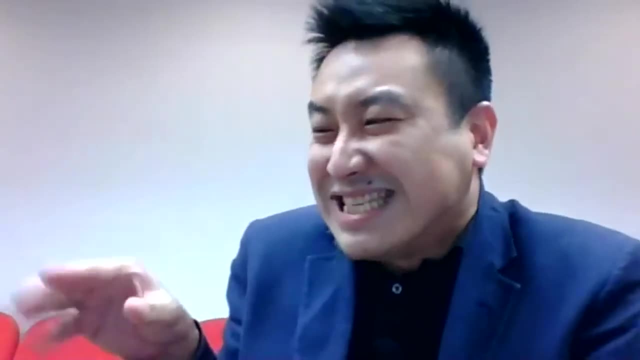 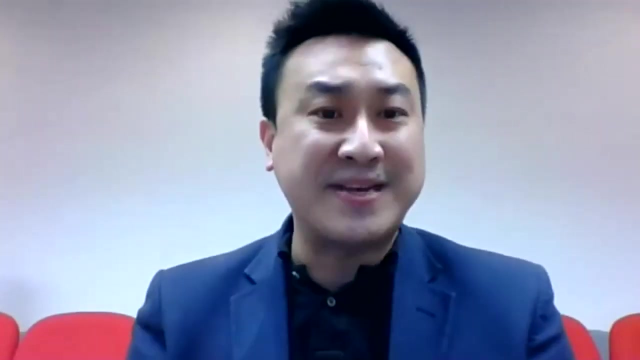 been funded by the UCR. so actually, well, some students told us that when they go to the field at the beginning, well, we were very excited. but they go to the field and say maybe I don't want to touch it, and eventually they think okay, I can do it, and they can actually identify. 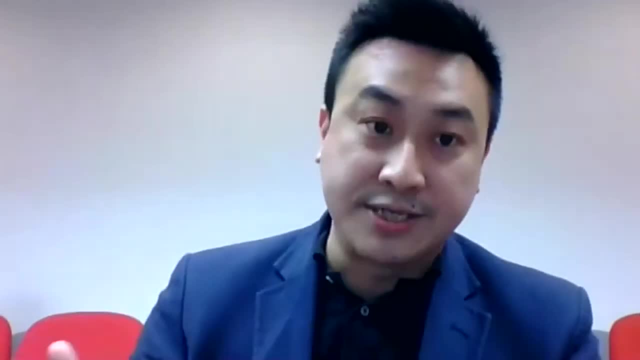 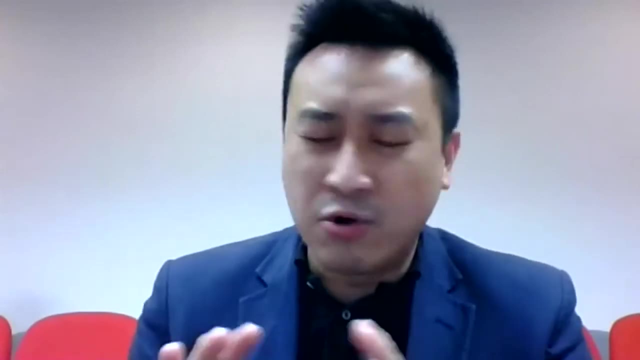 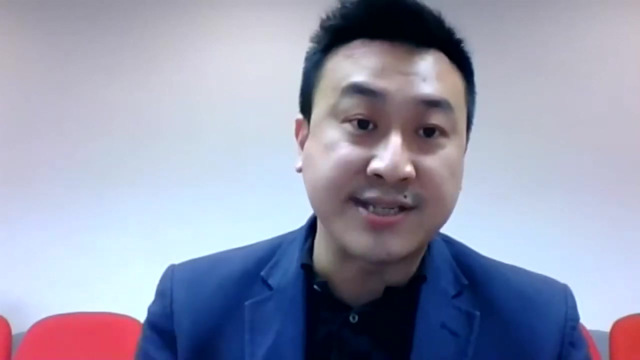 it. So that kind of learning and experience is the best way for them to to actually get into. So, of course, if you say documentary, okay, I think, of course, on, multiple channels are fine, but hands-on experience, I believe, is always the key to to to answer your second question, 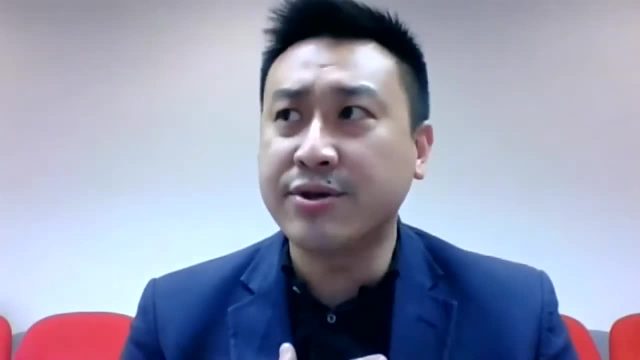 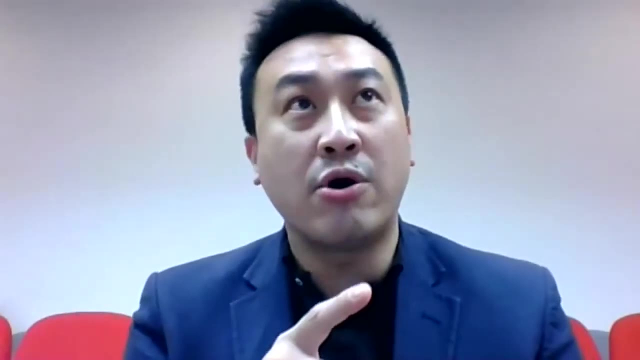 and of course I mean at Chinese University of Hong Kong, how we can do that, can we actually open some spaces or can we also actually do as you, if you remember the talk that I've been showing? I mean, which we are going to do is we're going to use an app, because we, we have been 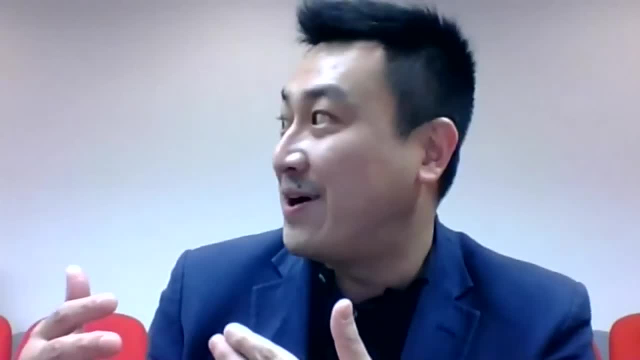 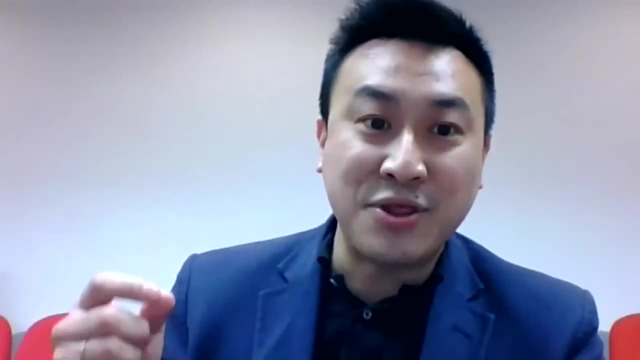 seeing that people, actually new generation of our- not only students, youngsters or teenagers- they want to learn a little bit of farming, lecture farming so, and the way that if you ask them to grow they'll say: oh, so sometimes I see something. what should I pay in? 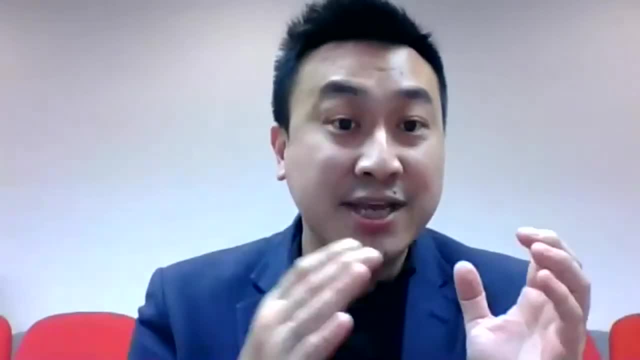 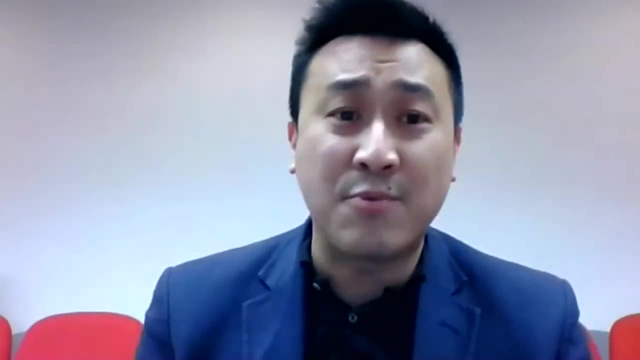 So we're using, trying to use a free model to also get their senses. once they feel engaged, I think that's the best way- then they will begin to try to find and learn more about it. So when you're talking about how I will, how diversity and sex, etc. 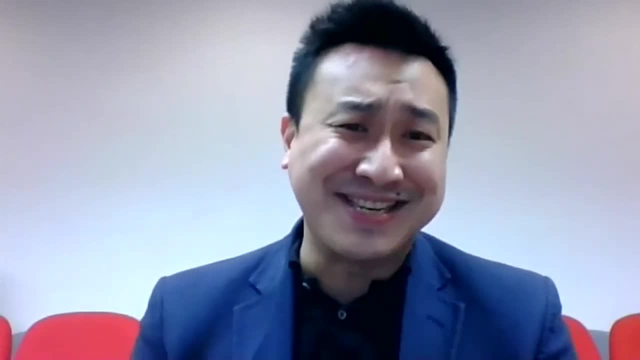 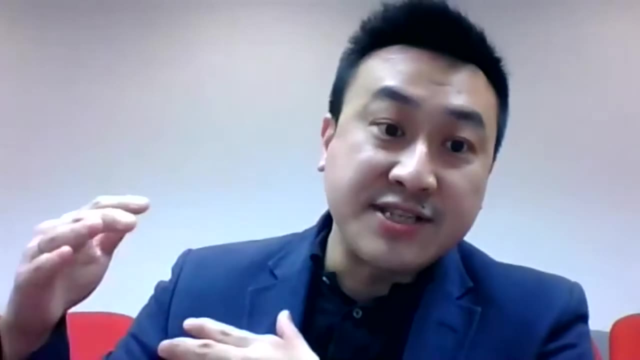 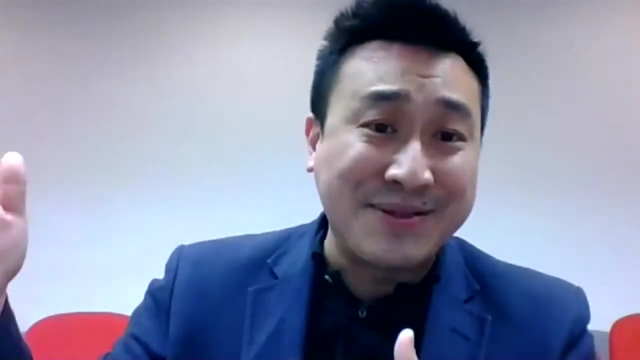 Your first question is difficult to answer, I mean, I'm afraid. well, the reason is because, for example, an under climate change, well, this kind of insights may be growing in this area, but they may also do like: well, you know, you study entomology, you know they were doing migration, so the other places they may be. 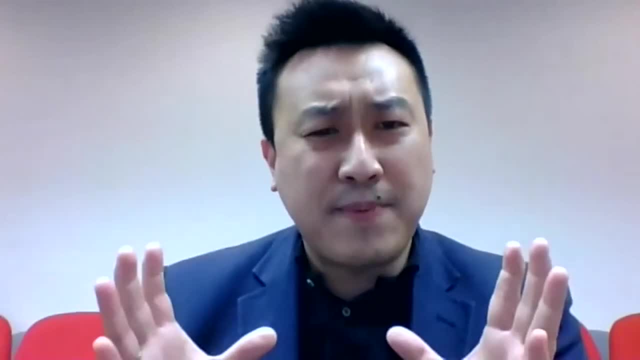 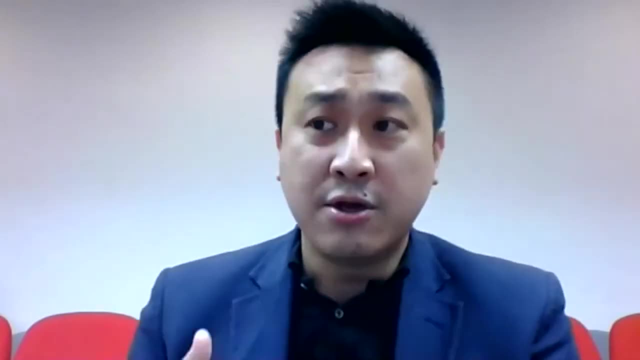 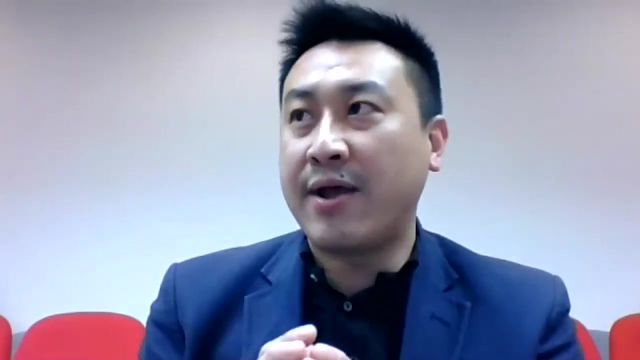 bad. they may be good so are. I don't want to pick particular one. I think that should be regional-specific. you need also to look into the consideration of the crops or the associated or the surrounding plants that are having is. I would say that should be. 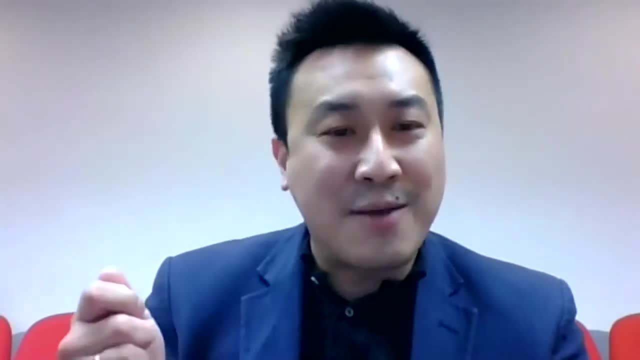 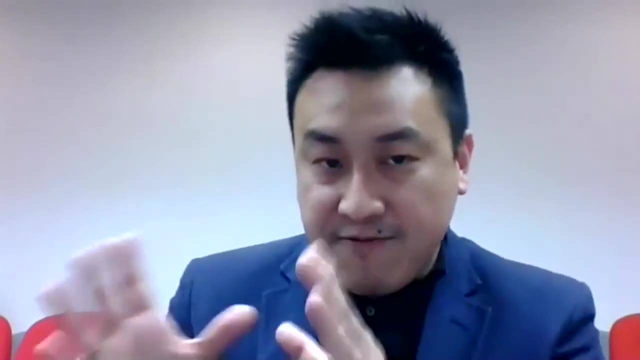 like a holistic way of rather picking. I think I will be very, very biased and say this one is important because I'm working on it. I don't know. I think every different question, every different scenario and every different geographical location they will have different. 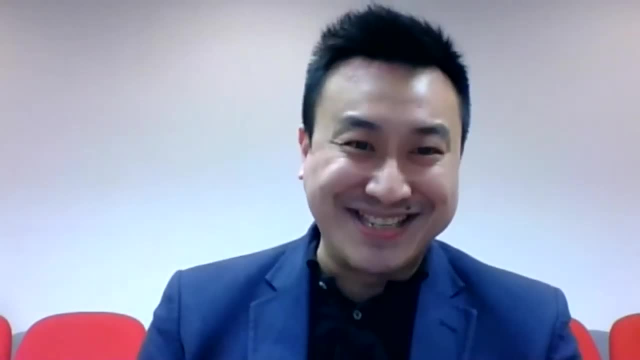 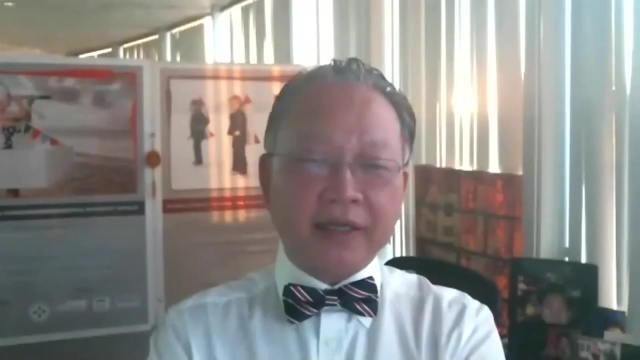 they will have a different question, So I hope that is fair in that case. Well, this is a follow-up and also a comment. So for our new president, so to him: Biden, President Biden, really look at the green technology and green environment. 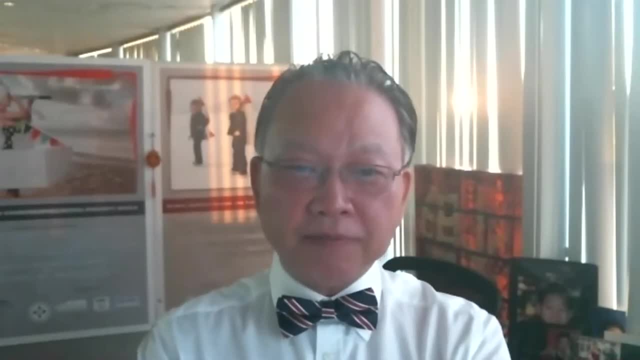 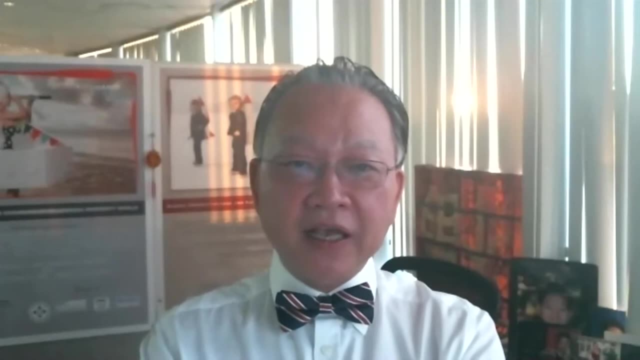 I think I don't think that he's really more focused in this, like microflora or what we can do in our soil and everything. I think this is a very important body of science And I think that you know the new president. 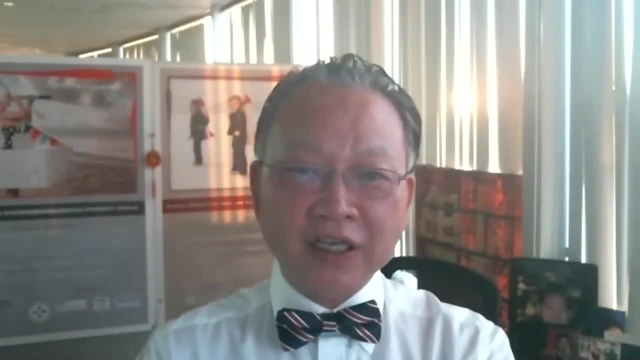 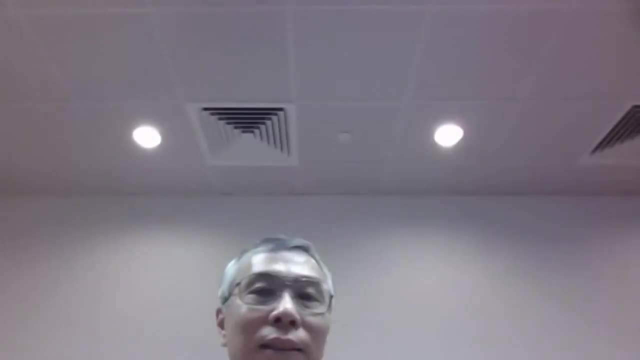 particularly in the United States, when he keep talking. he keep talking about green technology, And so I probably would use your email and ask you more questions. Okay, thank you. Thank you very much. I'm very happy to assist in whatever scenarios. 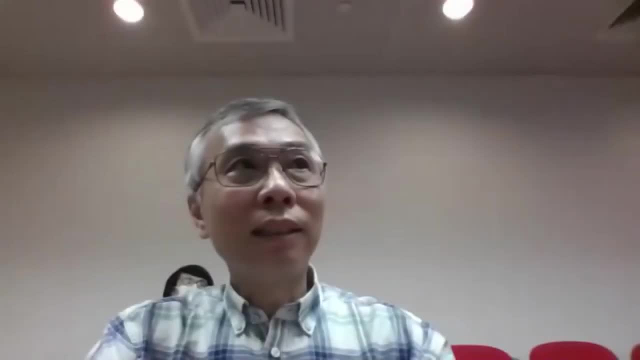 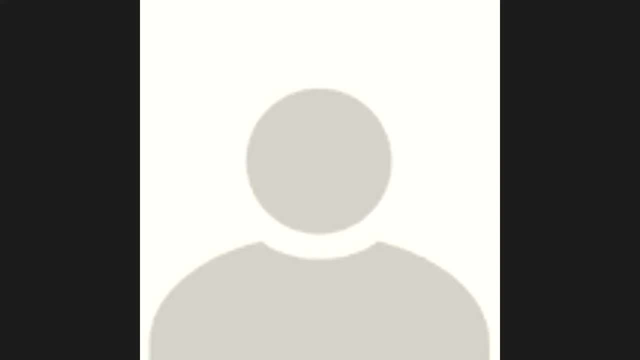 All right, thank you. I think Marcia has raised your hand right, Thank you. Thank you, Prof Lam. I have a question for Jerome. So I know you saw the latest publication about the discovery that a white fly uses a stolen plant gene. 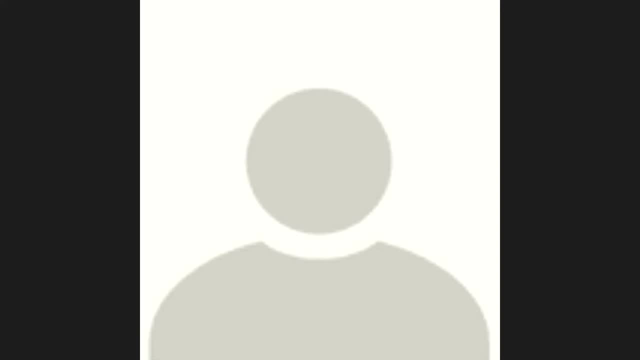 to elude its host defense. It was published in. recently a short paper was published in Nature, but I think the main paper was published in Shell. Did you ever see this in your screens or are you only looking at from an animal perspective and you didn't look at both? 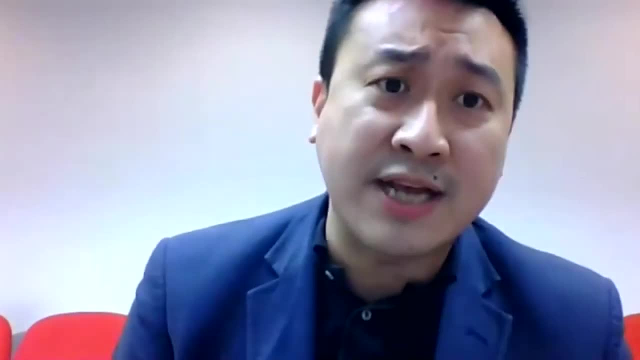 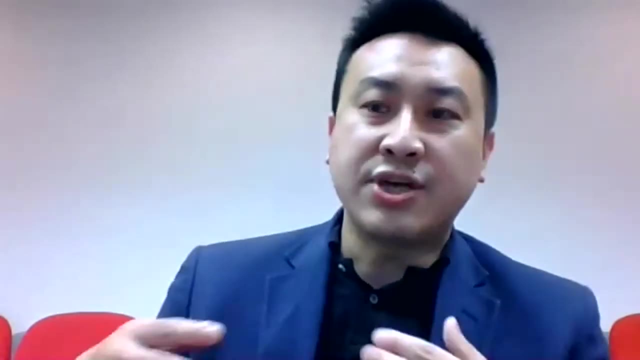 Thank you, Marcia. So yeah, I'm aware of that study. I mean the study for those in the audience may not know. well, I mean, this is a very interesting case. What it's showing is actually the white fly in the plant. 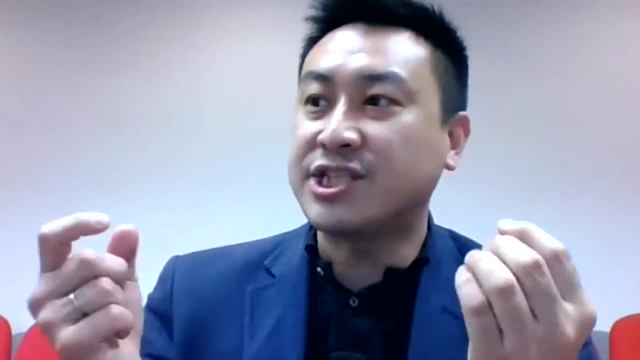 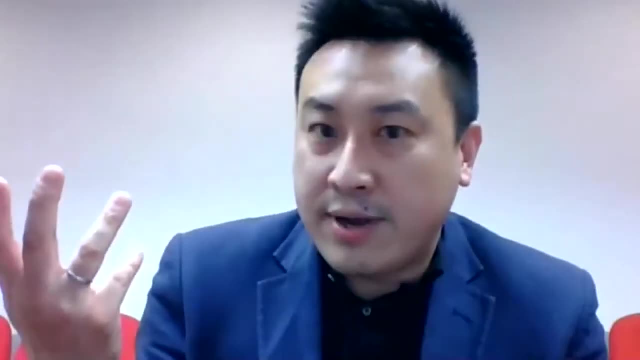 Okay, So this is the first case showing that there's actually horizontal gene transfer coming in between the two. okay, While it's published in Shell or Nature, I mean. I think that is reasonable. So that means actually something that is actually coming from one organism. 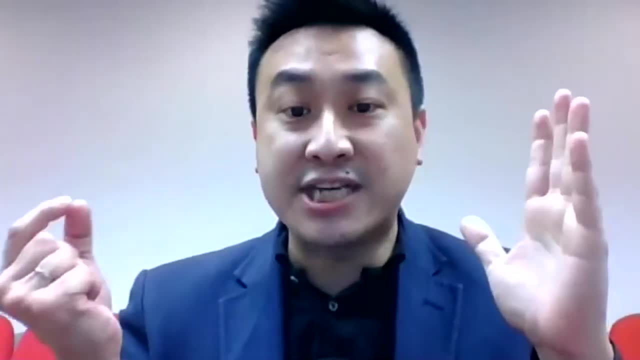 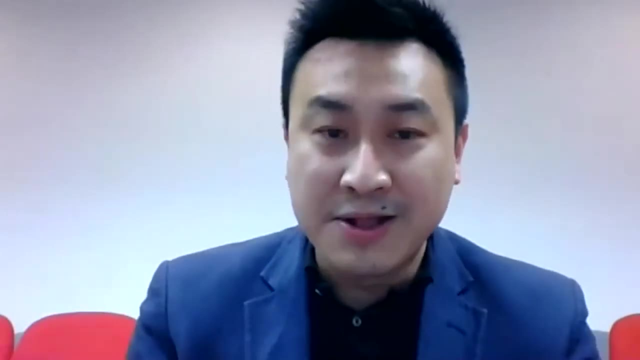 You know, think they have interaction all the time, but the gene can actually be transferred into the other species' genome. I think this is something that hasn't been looked very carefully before. Actually, we look into it, but I don't want to say that now. 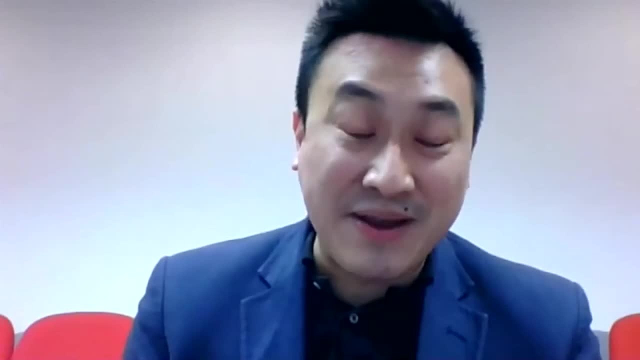 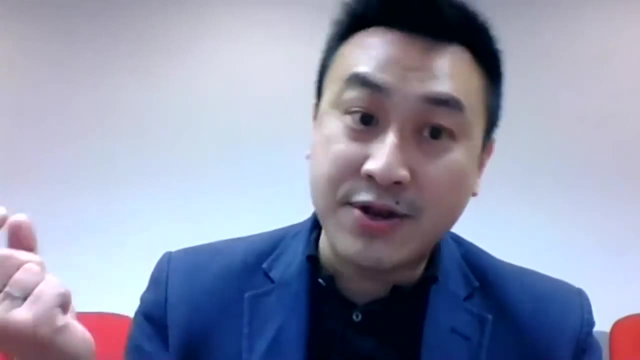 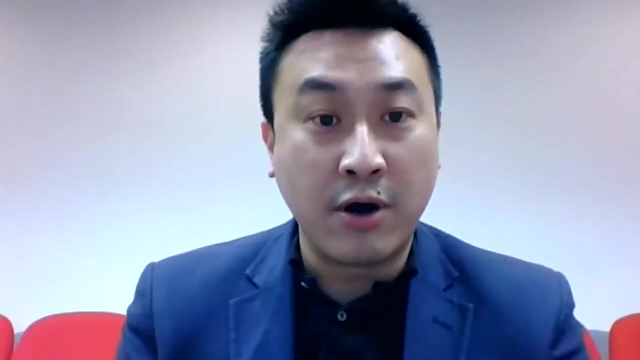 But yeah, I mean, I think this is going to be a very, very, becoming a very hot area. So, and how are we going to utilize those information when you're actually coming from the other gene? So what are they actually happening? Yeah, they are going to be very important, for no matter. 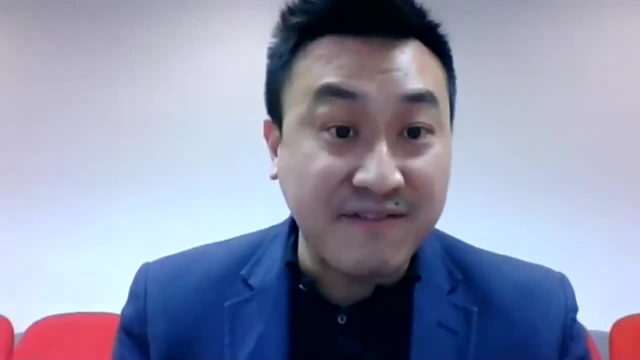 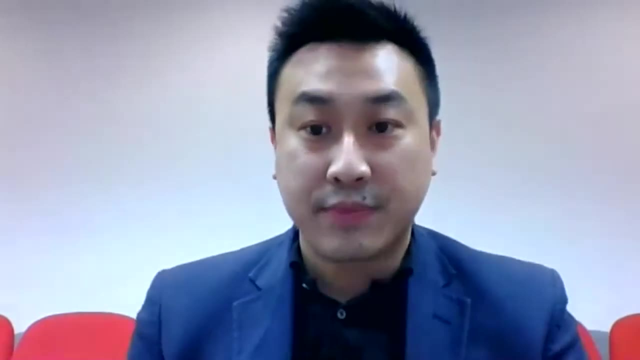 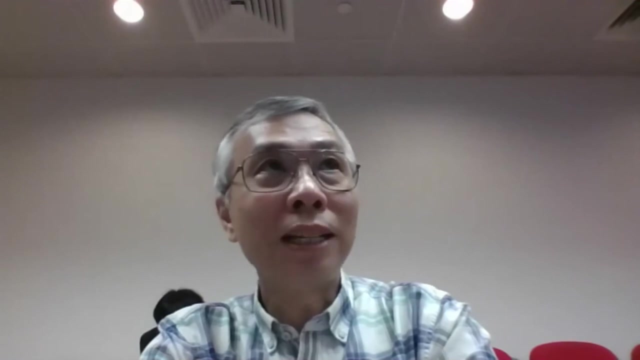 controlling the numbers for insects or actually benefit the crops itself. Yeah, so thank you, Maslow. So that's the question in the chat box by Xi Yundi. So he would like to know how to introduce RNA-bentham into fruit flies to inhibit juvenile hormone. 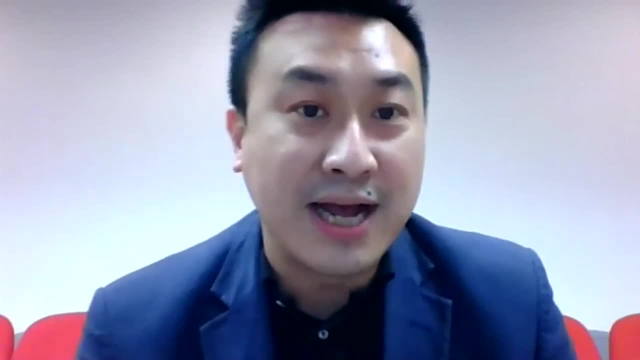 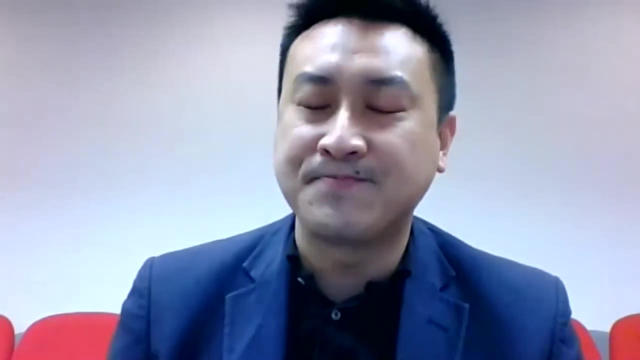 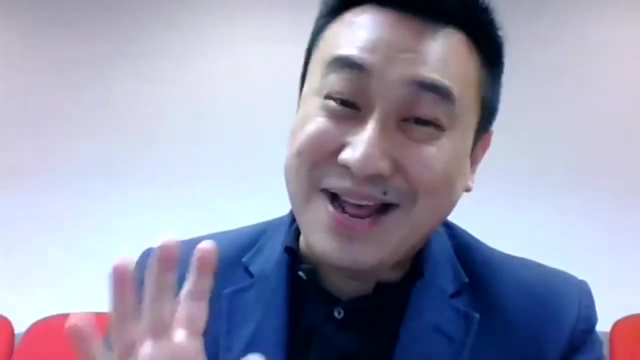 Okay, so thank you for the question, That's, I hope you're having a background in molecular biology. If not, you're trying to get some DNA. okay, You put in in a very simple term, you put in the DNA together with the bentham, for example, with your microRNA. 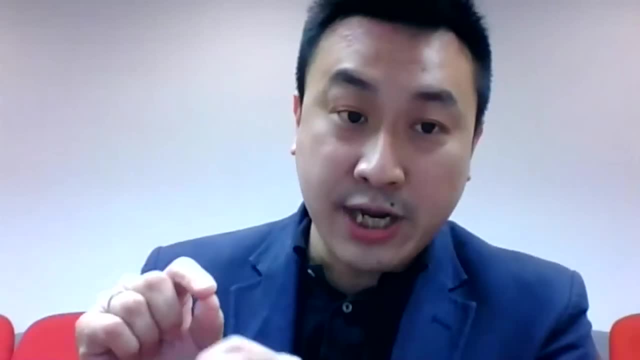 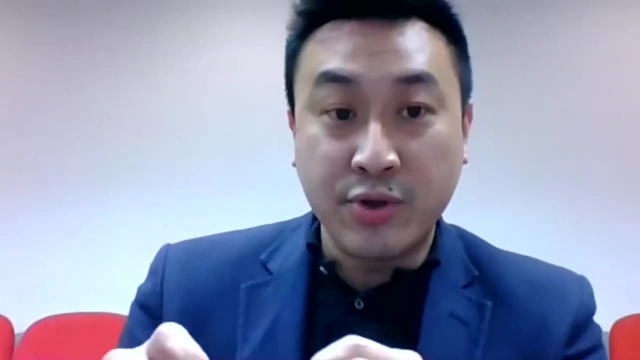 You inject them into the embryos. okay, Fertilized embryos, you inject them. So of course we can put in some selection marker so we know that, oh, they're actually mutants. So after, after, then we cross the flies, then you'll be able to make mutants like that. 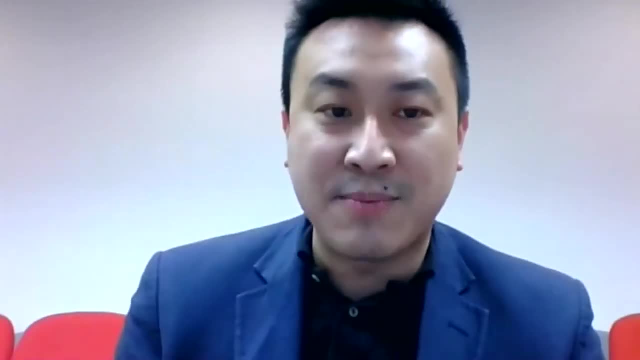 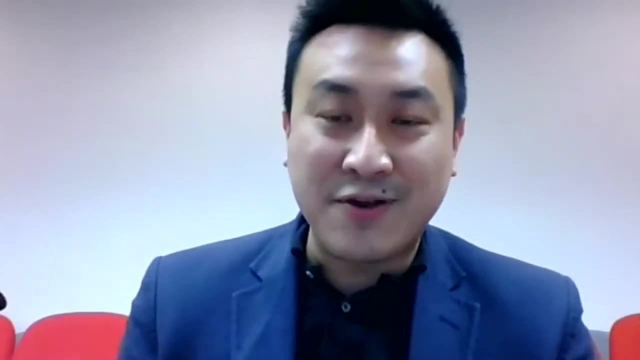 But I understand the question that you're asking is actually more than that. If you want to do that in the field, how are you going to do it right? So this is also an area that we have been trying to develop. It's: how can we actually massively produce a lot of microRNAs in the field? 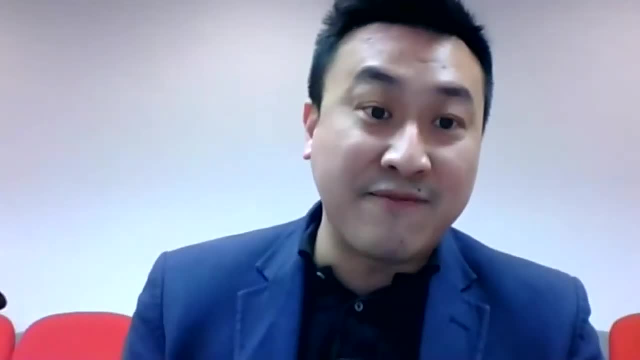 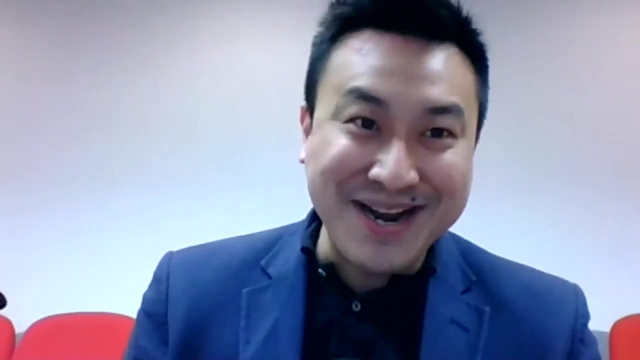 Of course, this has been the idea that we have been talking with Professor Lam for many years ago. You don't think? no, RNA won't work, okay. Okay, Take a look at what is happening with our vaccine now. right, 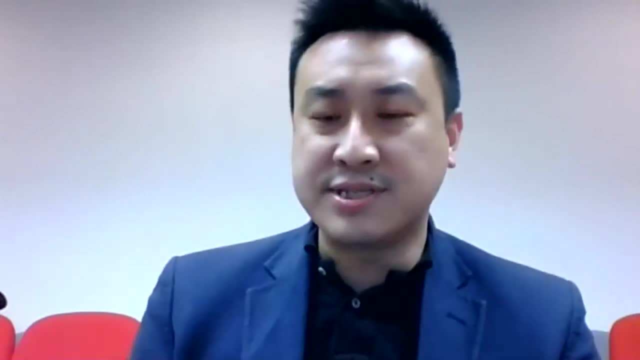 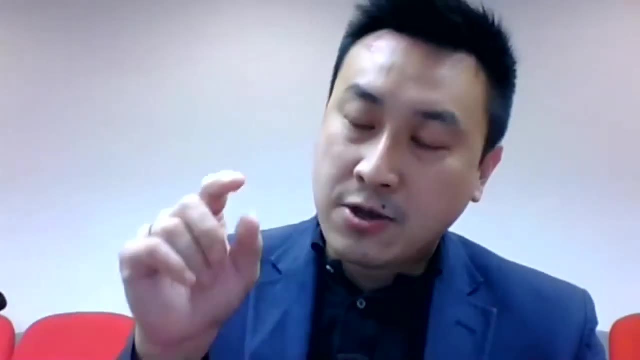 Okay, So it it works. I mean it works, But how we can? but before we try to do that- in insects I'm talking about in this case- we need to make sure that they will be specific to that particular insect. 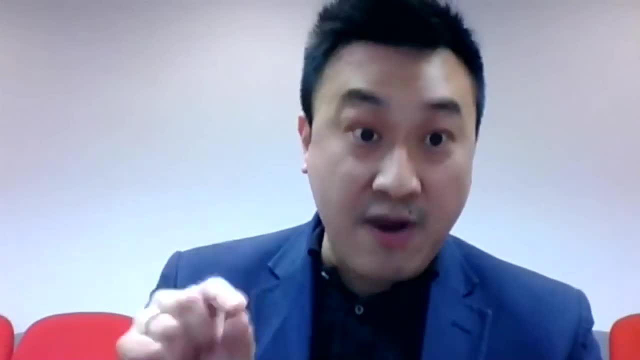 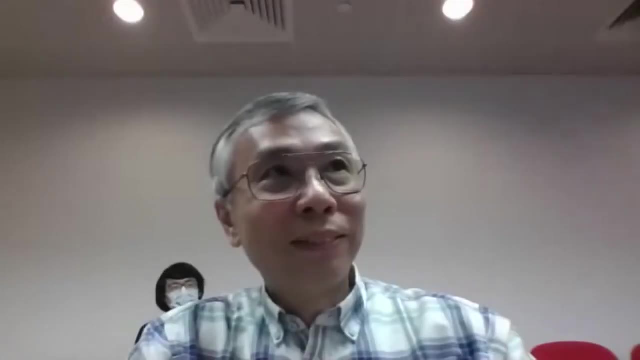 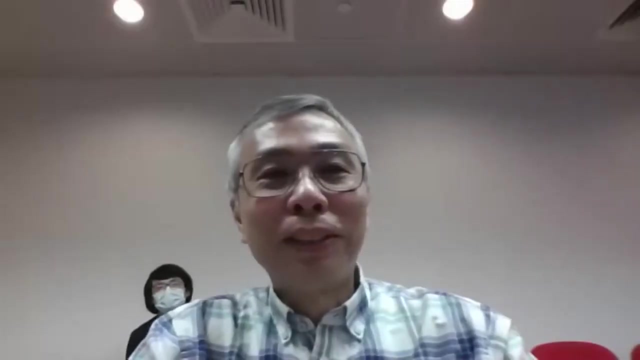 So to that particular group, otherwise they will be very, very disastrous event. Yeah, So I hope I can answer your question. Okay, So maybe I ask a question, Okay, So well, I guess I just have some imagination. So food security is also. it's always a problem. 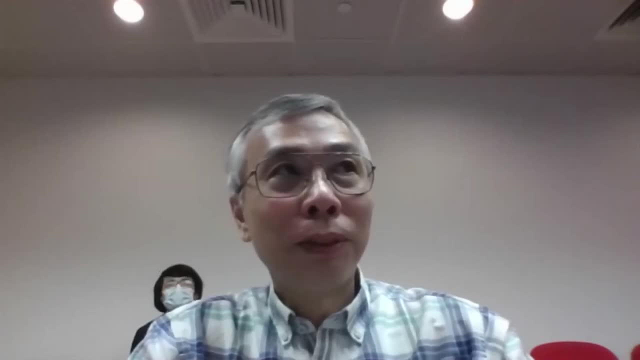 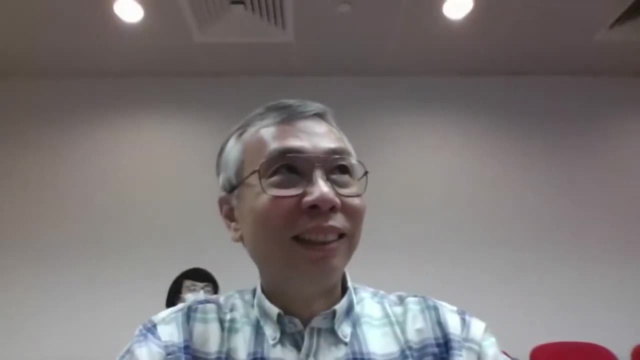 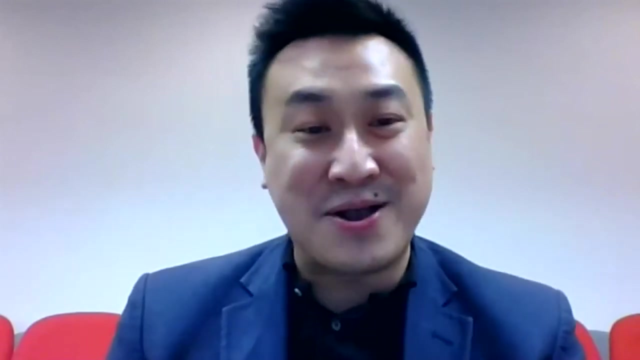 So could some insects be developed to become food of human? Huh, Um, you know I was joking. I mean I I was asking whether whether I watched a Korean movie which is very interesting because they are using cockroaches and they're trying to make food. 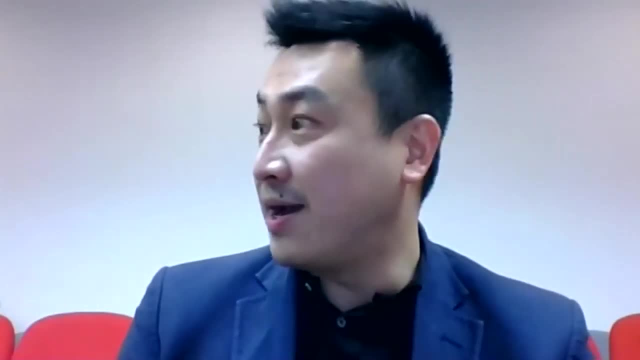 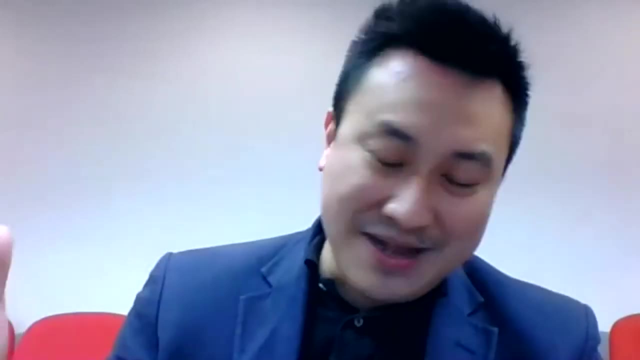 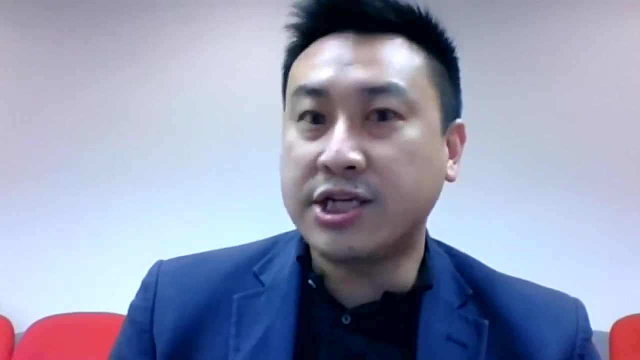 I mean, actually, I've been approached by a biotech company. They have been thinking about those. of course not feeding human, okay Feeding, feeding other other animals, et cetera. I think, well, actually using insects, you know, or even the, the products, the food waste have also been. 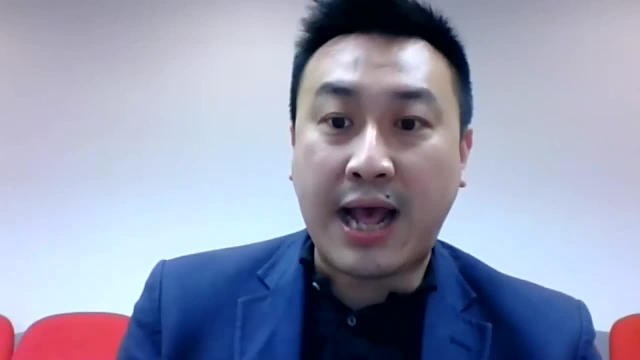 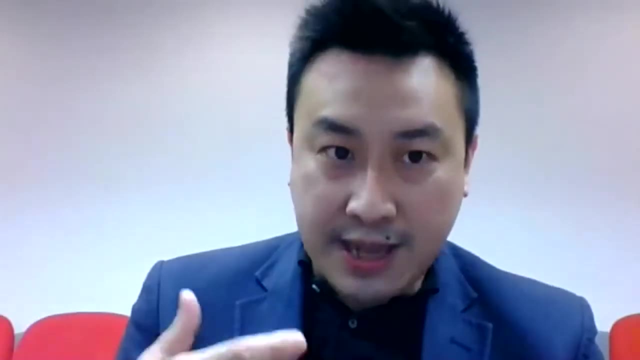 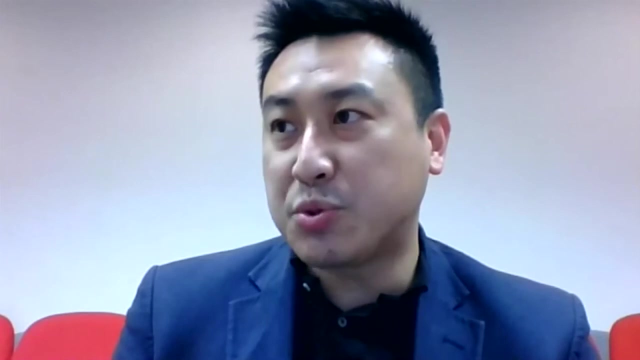 have also been doing okay. I, I it has not been doing very properly in Hong Kong. Many people only focus on like beetles I mean, but I think there are many things that can be done, Um, uh. so I again I don't want to, um, you know, I don't want to. I always want to get more minded. 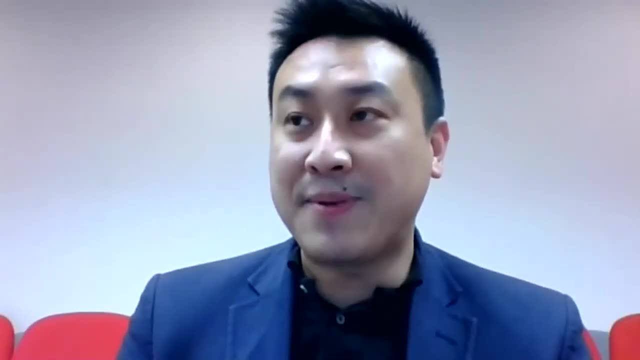 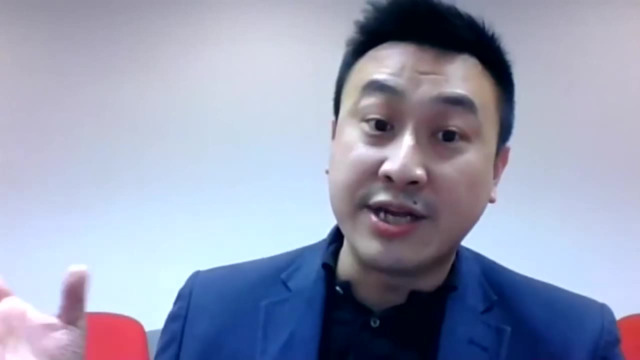 So I don't want to propose a specific one. It also depends on scenario. For example, right We, it's not my PhD student, I, I, I. one of my colleagues has retired and now I'm the co-supervisor. 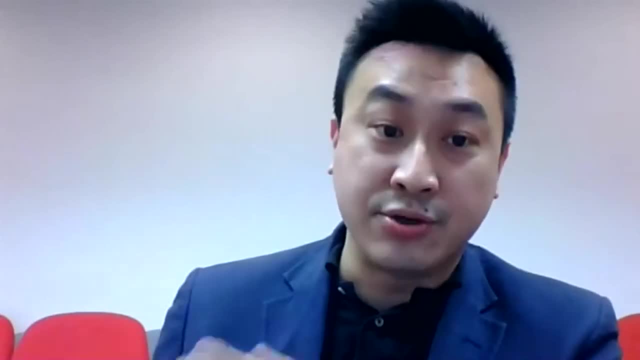 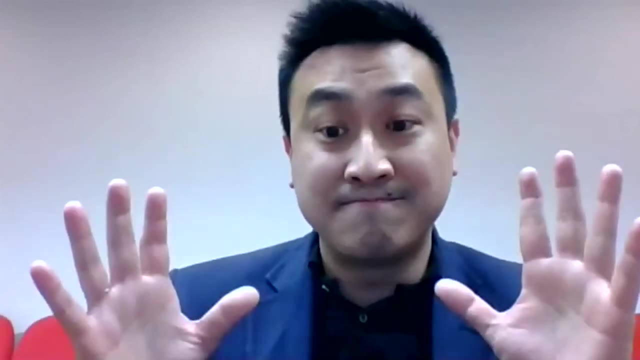 And she's actually working on food waste, using insects to to do uh uh, using different kinds of insects. you know different ways and different food products and et cetera. So, uh, yes, they can be done, et cetera. 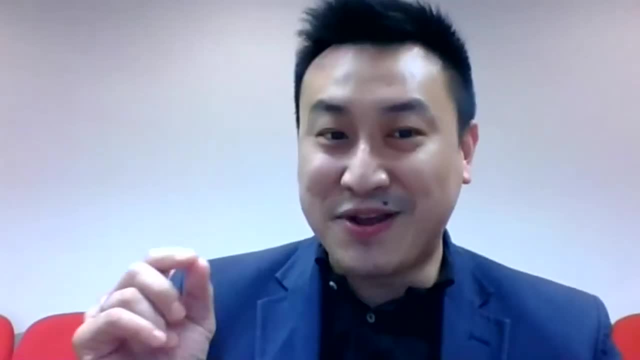 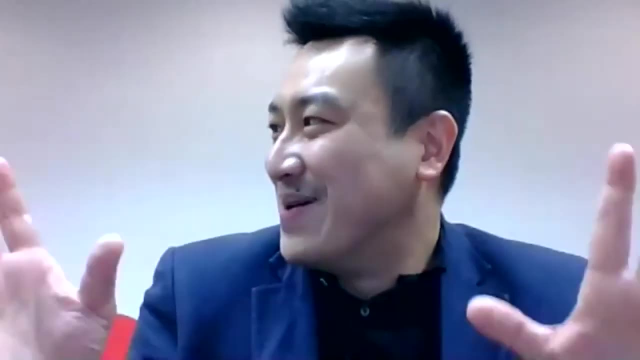 But uh, I think human always has a concern of eating insects, So it should be insects And it's just go one. I mean maybe feeding a fish or whatever. Okay, Then we eat a fish. That would be better. 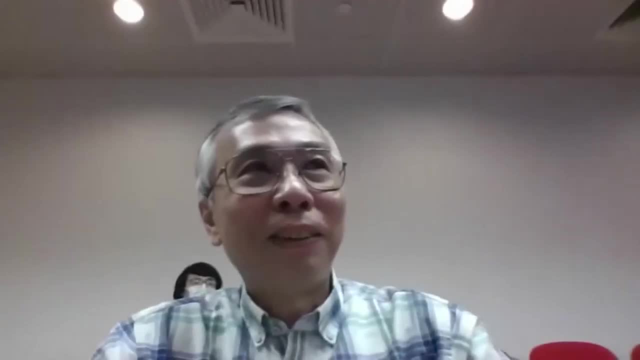 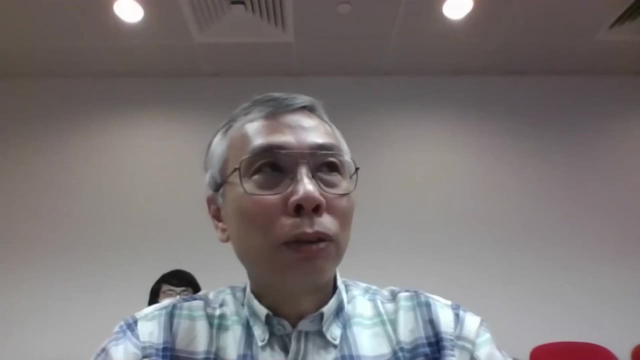 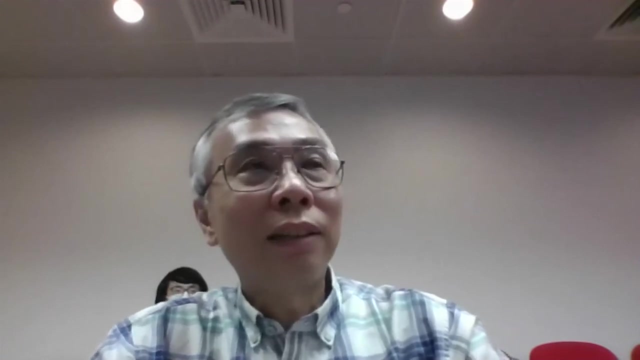 That would be more acceptable. Okay, Yeah, Because I always think that, uh, insects high in protein and it is a recycler of nutrients, So it should be very energy efficient if we can make use of it in the food chain. So, but anyway. so that's another question by Coleman. 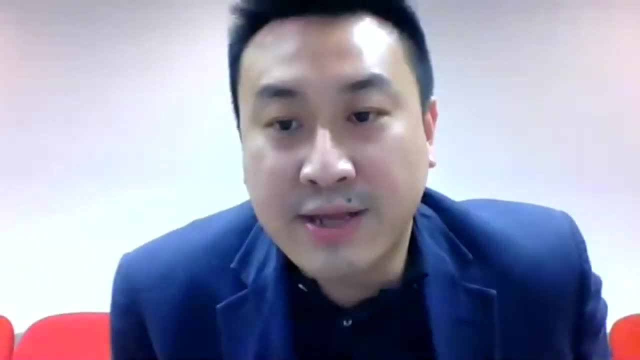 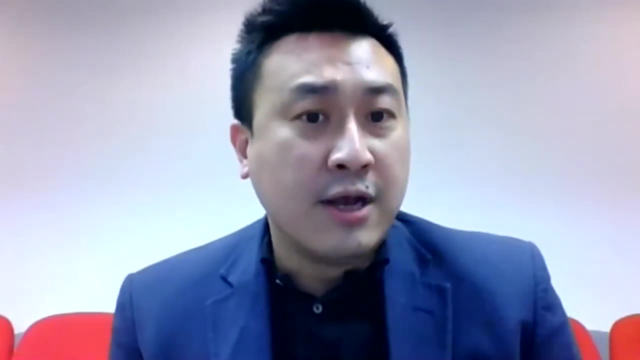 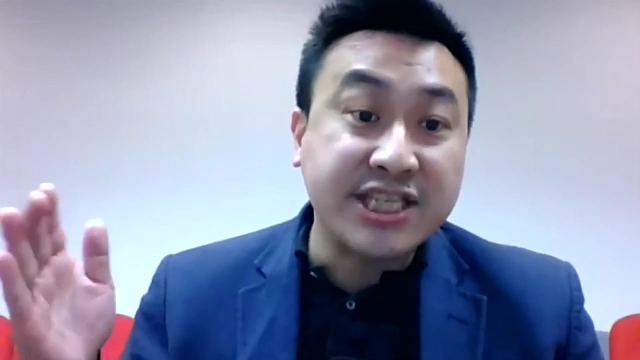 Yeah, Yeah So. So Coleman is asking whether we can uh, create artificial juvenile homes to increase the population of beneficial insects for agriculture. I think this hasn't, hasn't been tried, And I think that should be, for example, bees, or even those insects that are actually taking away the pests. 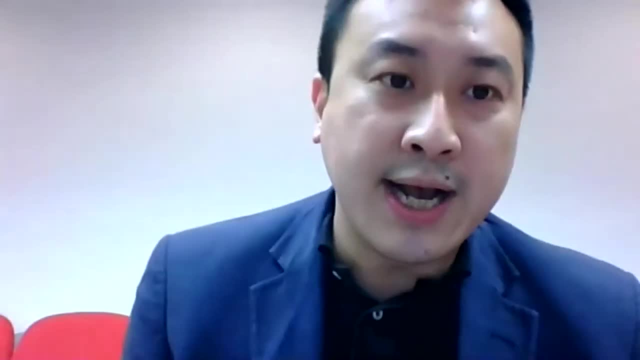 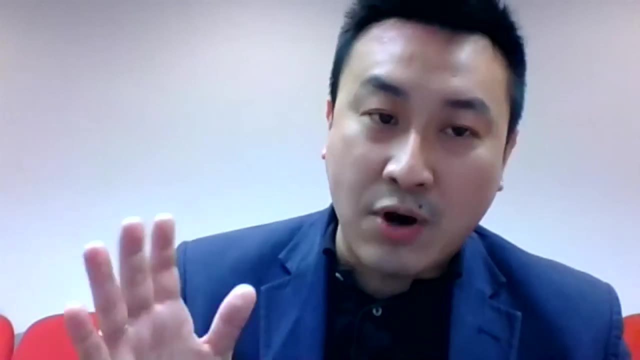 So they are. we also regard them as beneficial insects, right? Uh, yes, that is possible, And um and uh, as I've said, uh, artificial juvenile home is very difficult to to make. Okay, The reason is because, uh, it's very difficult to synthesize that step. 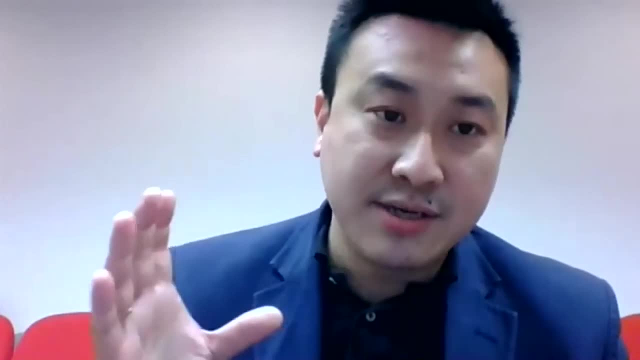 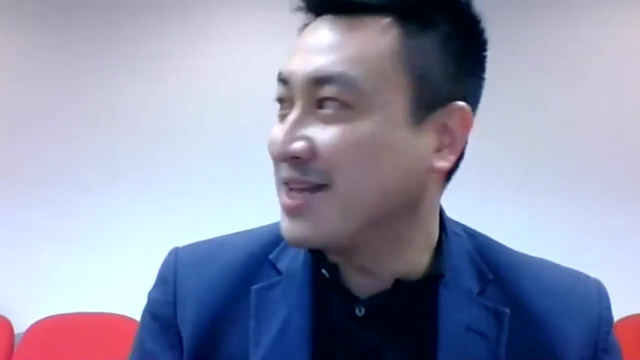 So what you can make, um, uh, mimics, uh to those. uh, I think that is possible. Uh, just haven't been tried, And you need a, a partner that is willing to try, Because, uh, when I first uh collaborating with Professor Lam, I said, oh, why not? 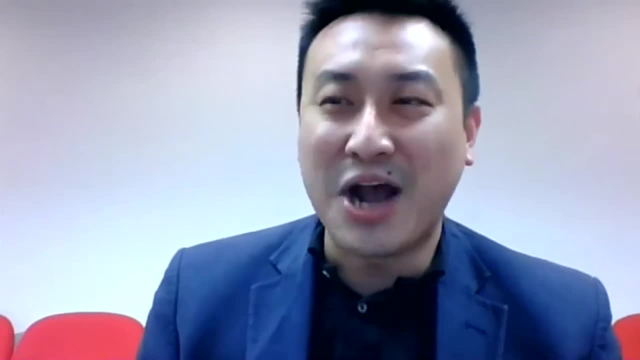 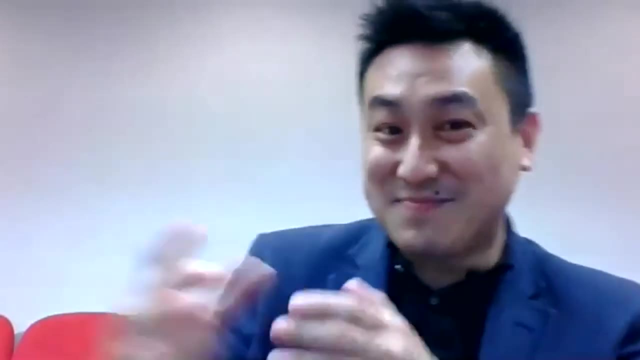 You should try to do something on soybean together. And then he said, okay, you can do it there, not here, Because you will eat all my soybean. So you need to find a partner with a space that you can do the crops on. 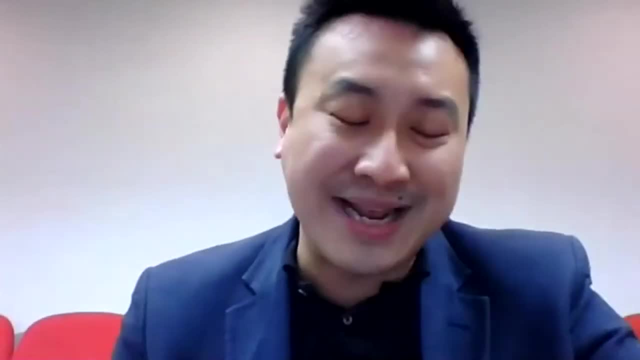 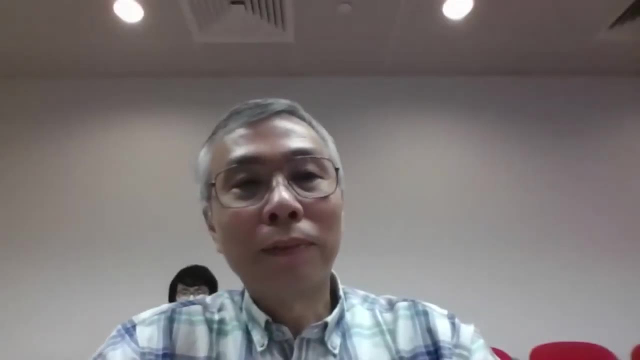 Or et cetera. So I I was tempted. Yeah Well, I want to follow up on this right. If you synthesize a compact um molecule from by the local process, of course it takes a long time. 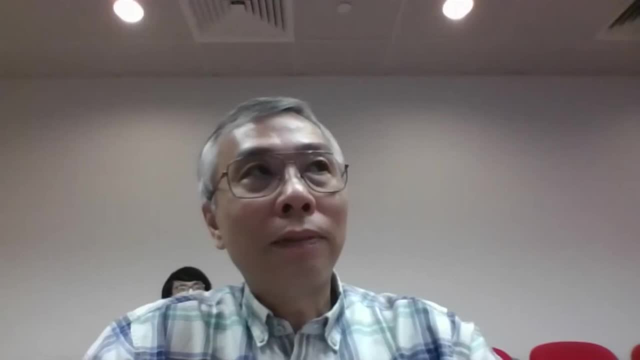 Yeah, But how about, uh, if you have identified similar compounds, from plants, for example, then you made a few steps. is enough to convert it into bioactive compound that can be used? Is it a possibility? Uh, that's a super question. 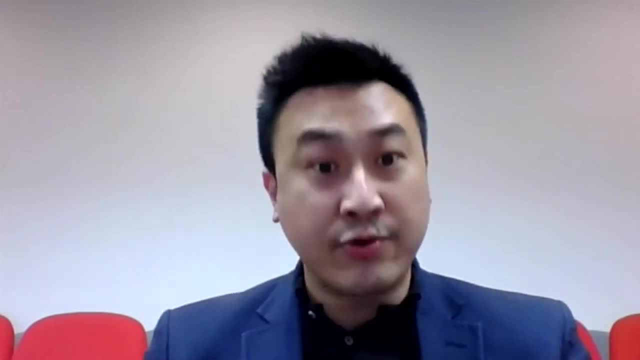 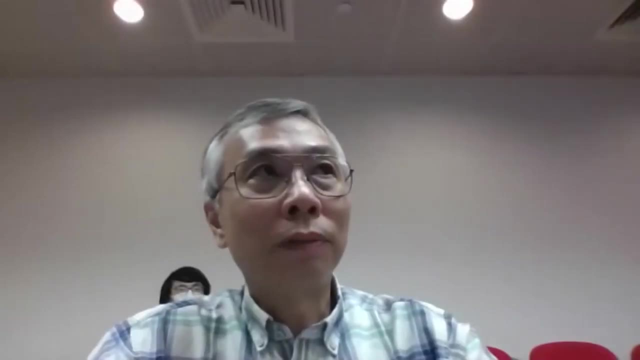 Super clever idea. I don't think that has been thought before, But it's a very good idea. You can try. Yeah, Because I I believe that uh, for example, terpenes is quite similar to the structure of silver knife hormone. 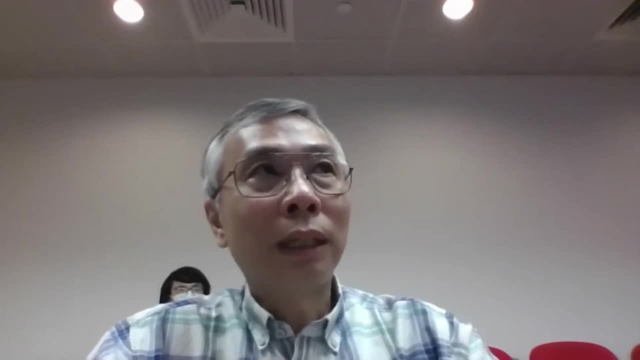 Maybe some side change changes. So if we can just target to a few steps, that could be much easier than you synthesize from carbon and nitrogen. Yeah, That is clever. That's very clever, Thank you Okay, So is there any other questions? 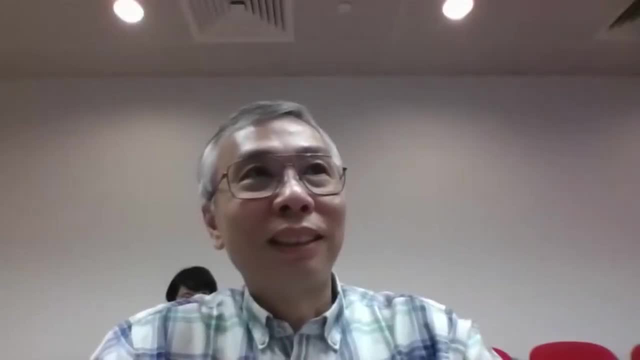 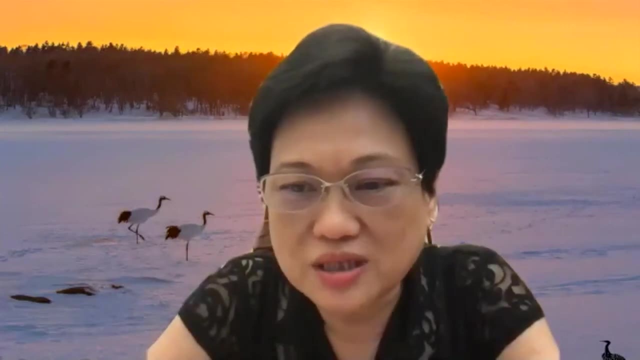 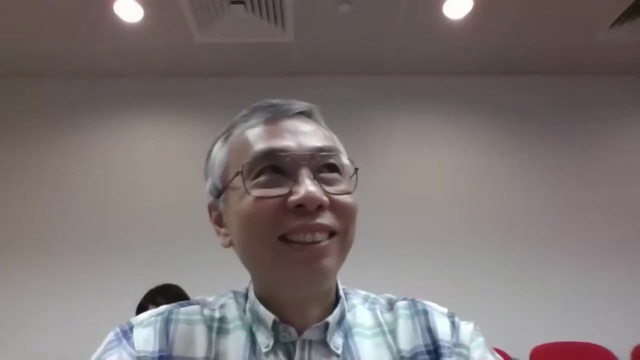 Any other questions from the floor? Uh, Dr Wei, I just have a comment about this. uh, the, the, the structure of this uh juvenile hormone. Actually, they look like some of the flavor compounds. You know, flavor industry, all pharmaceutical industry. they do make a lot of those similar compounds. 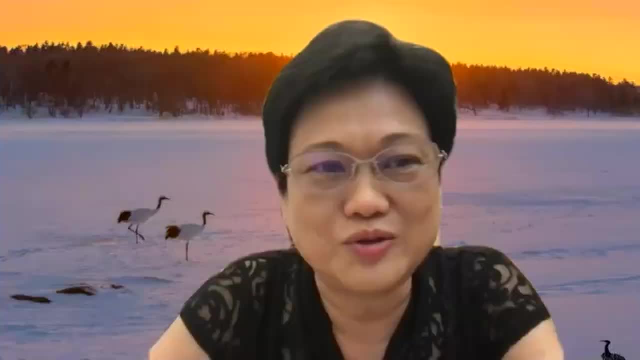 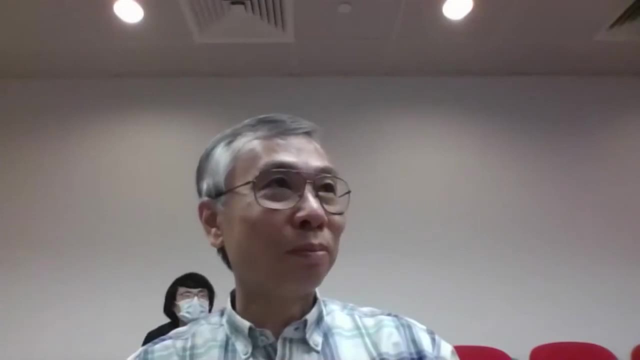 So you can consider that route. for you know, So, uh, that when I first met Professor Lam, he said, uh, I met him and his wife, And then he said, oh, that is called juvenile hormone, And he's thinking about exactly the same thing. 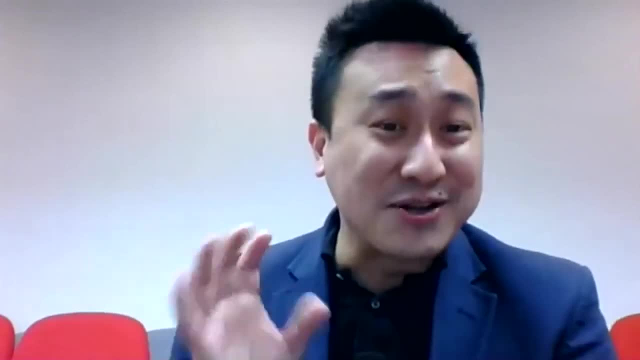 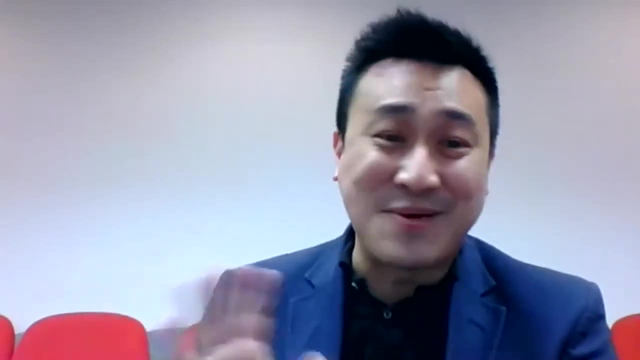 Uh, as a scientist, I have to say that hasn't been passed. They're called juvenile hormone. It has never been tested in human et cetera. Uh, uh, we can try to explore but, uh, there's no evidence so far. 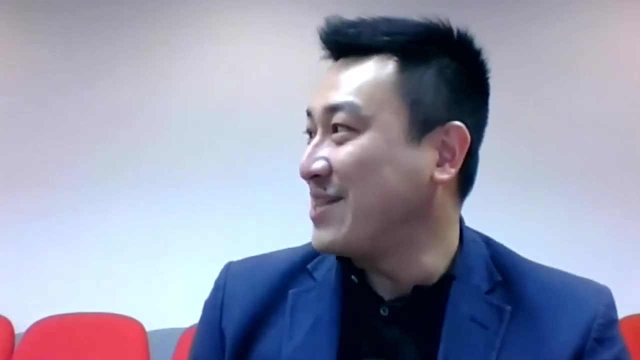 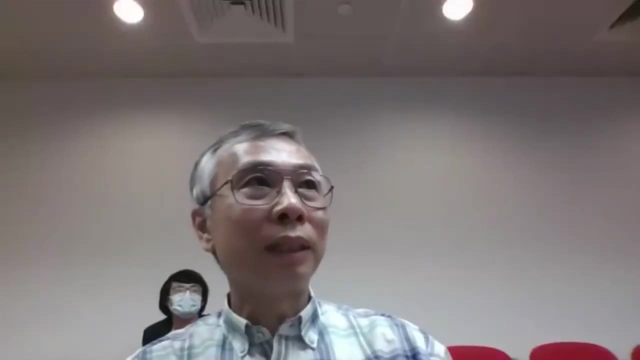 But uh, uh, here we can try SK2, right, SK3, that's cool, Yeah, I think. I think Dr Joanna Chan is talking about the, the flavor, Oh, the flavor, no, The flavor. 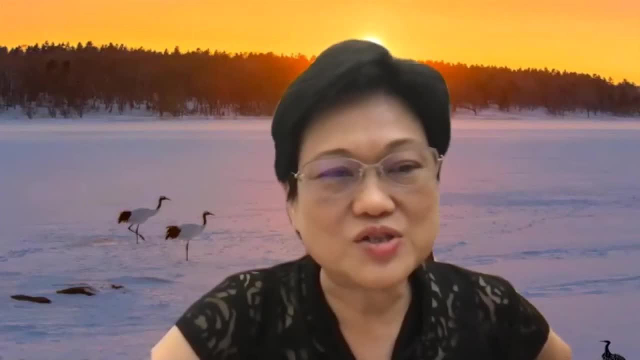 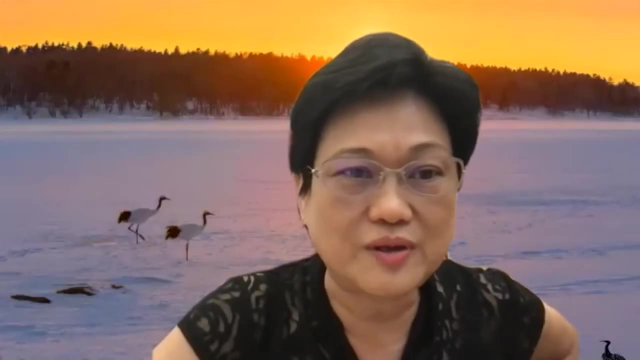 The taste. The taste. Oh, I see. Sorry, Okay, Because, uh, um, flavor industry, uh, identify many different flavor compounds in different from the plant or region, from the animals, and they carry all kinds of structure. Oh, I see. 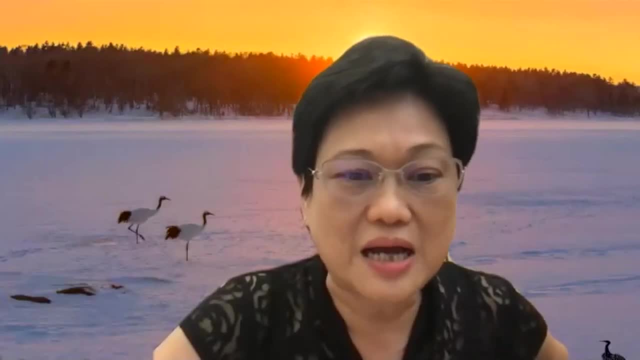 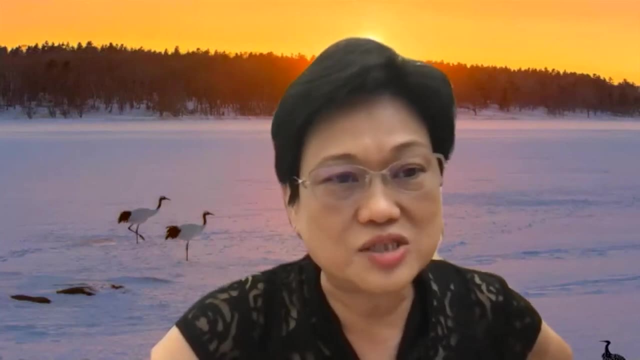 So when I look at the structure you draw, you know they look like some of the flavor compounds which, uh, some of the advanced flavor company they do this, uh synthesize. So they do have advanced research and invest a lot in this area. 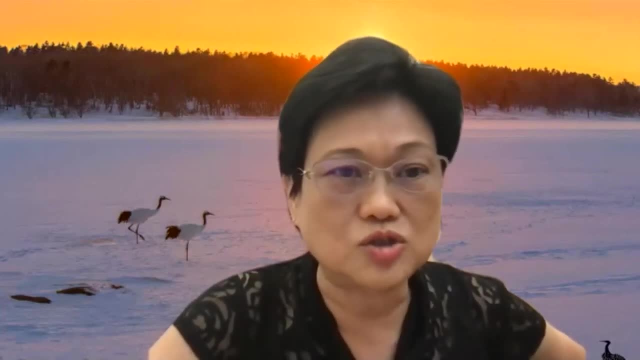 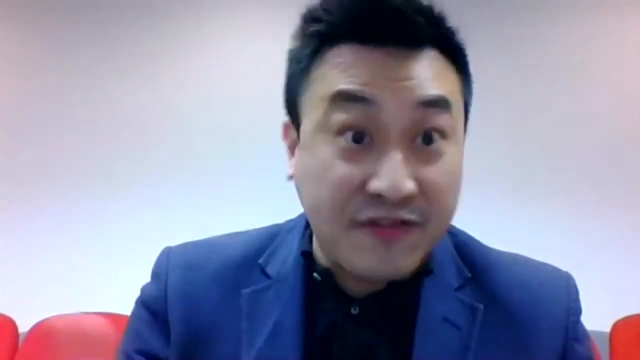 Maybe there's a chance to talk to this uh research team. Maybe there's a possibility they can synthesize similar compound or extract from different uh origin sources. Yeah, that that is uh extremely good idea. I mean uh. thank you for for for the suggestion. 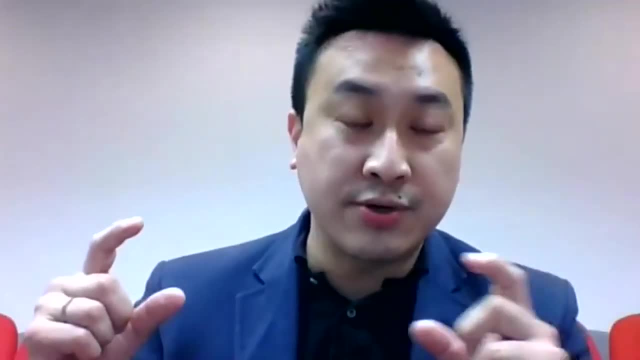 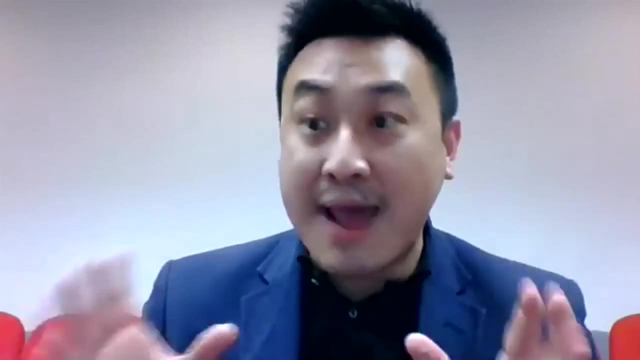 The reason is because when- if you remember the talk I've shown on the military right, So I I'm talking about hydrogen cyanide. Why am I so excited? It's because of chemists. They've been using that case. 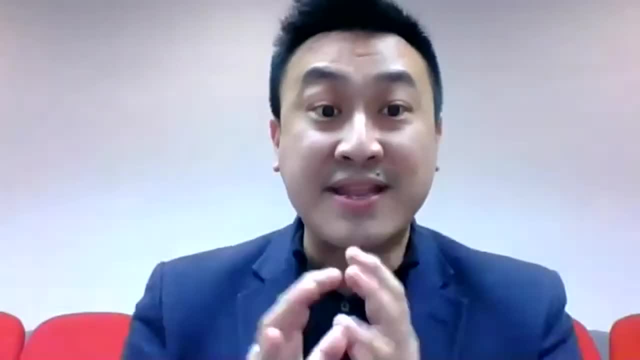 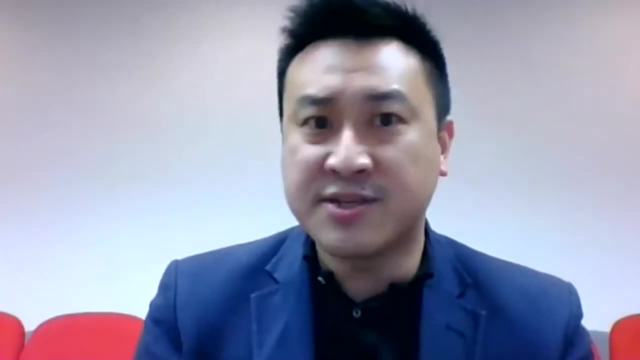 They only know the compound, the products, but they never know what is actually the whole pathway when we have the genome. Now we know. So, uh, I think, yeah, we, we should actually look into possibilities combining genomics and also look into flavors. 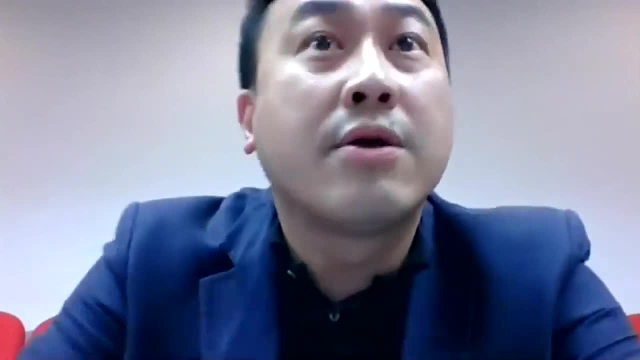 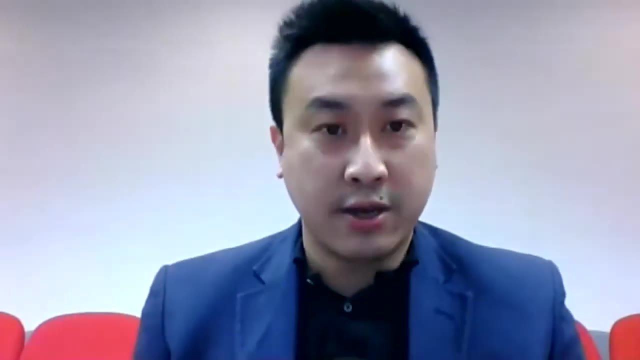 That is a very good idea, Thank you, Yeah, I'll be happy to facilitate, because I used to work for flavor company who devote a lot on the, you know, the chemical research. Yeah, So that's one question, My. my other question is: 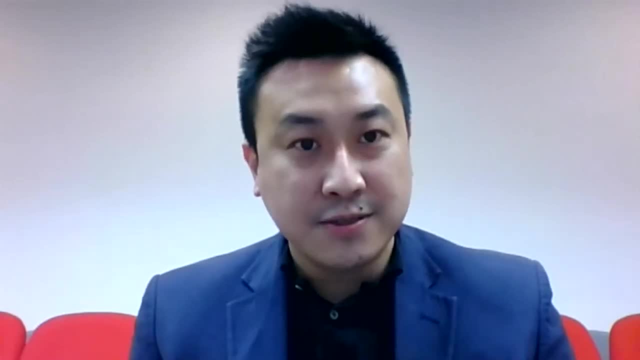 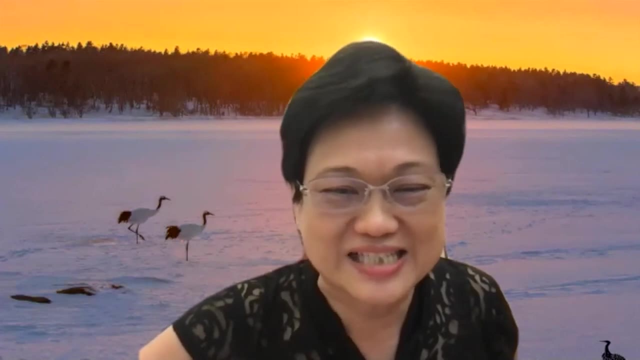 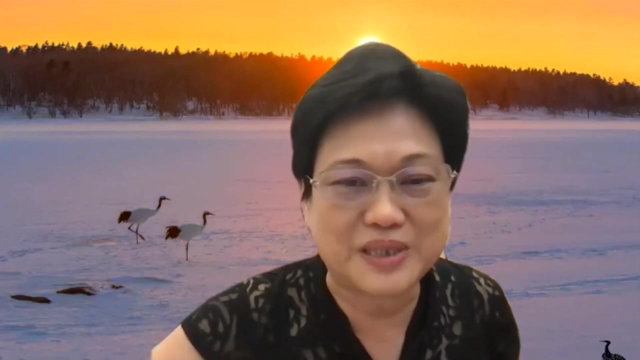 As a as a layman, I see many insects in my backyard when I pick into the soil. So how do I know? is too, too many insects or not enough insects? and for the apps that you were making for the past, where you indicated you know the the bad type that we should. 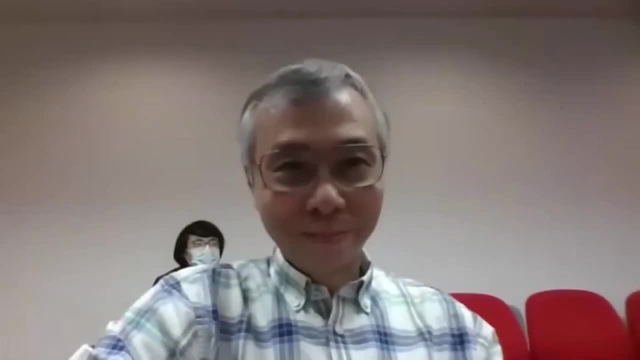 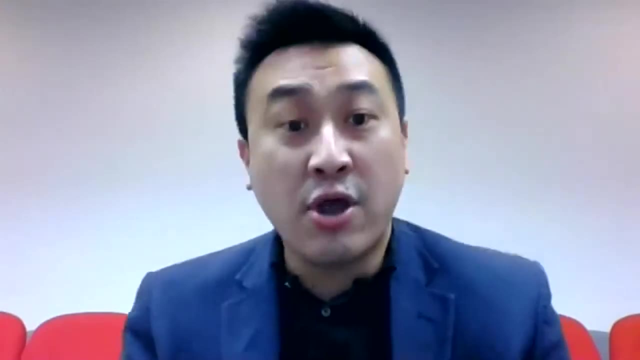 eliminate. So there are two questions, Thank you. So I I answered the second question first, which is easier. So, uh, uh, uh, for the app: uh, so we are actually showing you a whole survey that we have been doing in biodiversity in Hong Kong for for the farmers. 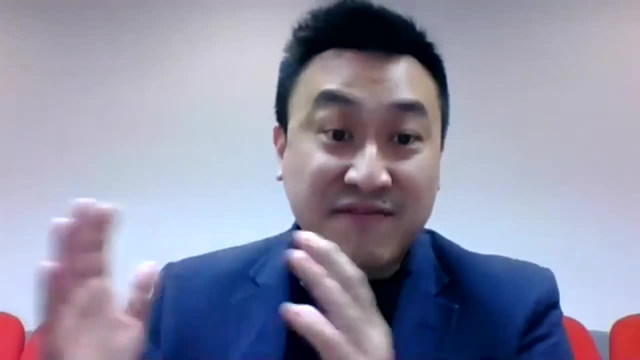 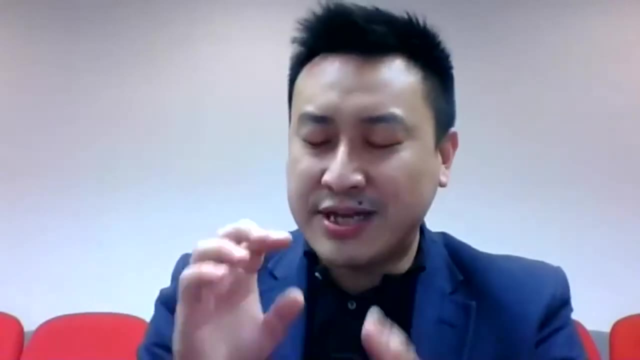 So you will see not only the pest. you also see beneficial insects, but also the one that we identify as neutral. Okay, So, uh, it's only not a web. I mean, I'm sorry, It's not only an app. 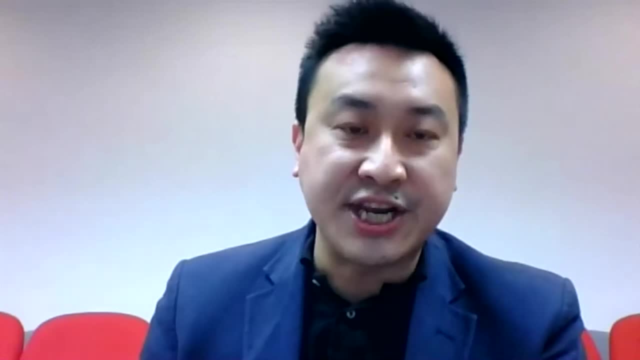 It's also on the website. I mean, uh, we will launch it later this year. So, uh, you, you have everything. Yes, You will have idea of which is good, which is bad. Regarding numbers, I mean, I think that really depends not only on the numbers, but actually what you have. 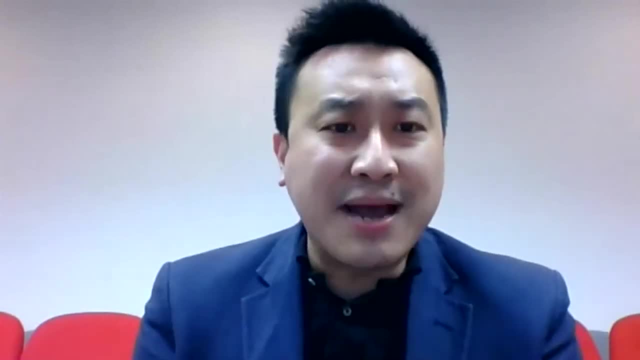 been planting on your back yard. So, uh you, you will have everything. Yes, You will have idea of which is good, which is bad, Regarding numbers. So, uh you, you have everything. Yes, You will have idea of which is good, which is bad. 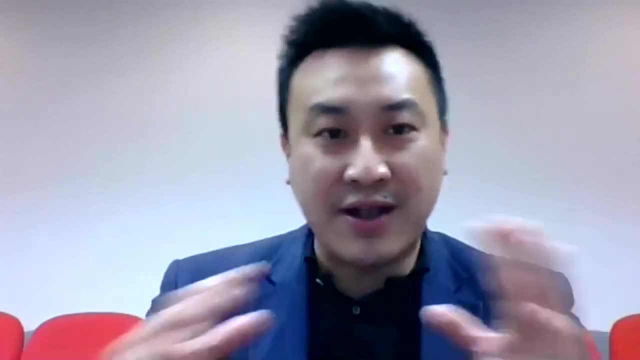 Regarding numbers, I mean, I think that really depends not only on the numbers, but actually what you have been planting on your backyard, Right? So, uh, it needs to have a combination of both. So, uh, that is the second question. 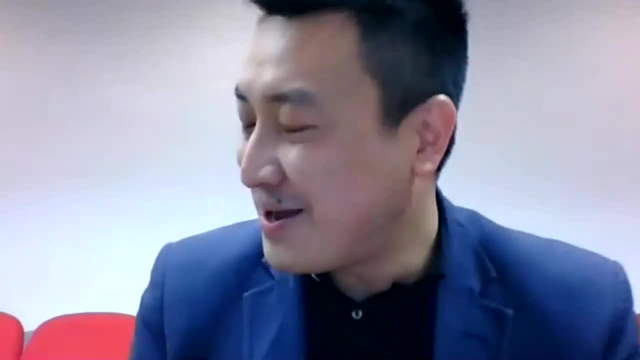 So for the first part, uh, uh, that is what was the first question Is it? is it related to the backyard? Um, no, First question is backyard. The second question is the app. Right, Yeah, Okay. 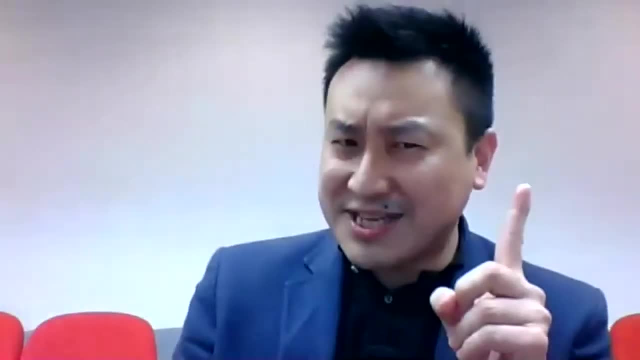 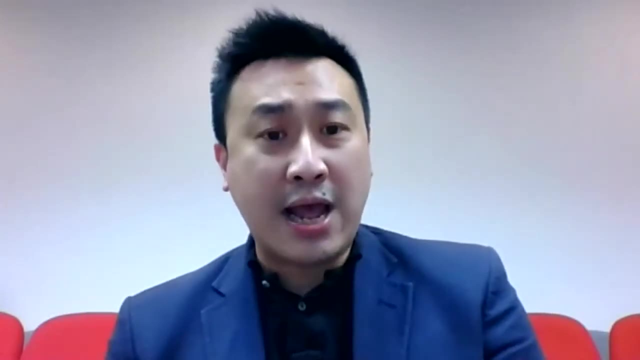 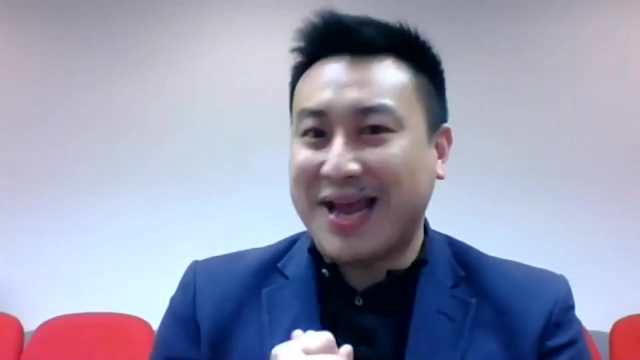 Good, Okay, I got it. Yeah, So, uh, yeah, I personally also look very much forward to to the app because, um, yeah, yeah, we, we are excited, We are very excited. I mean it's the first time that we tried to use a pretty model for insight and uh. 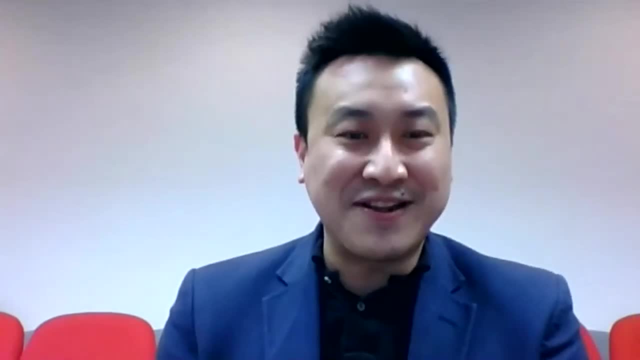 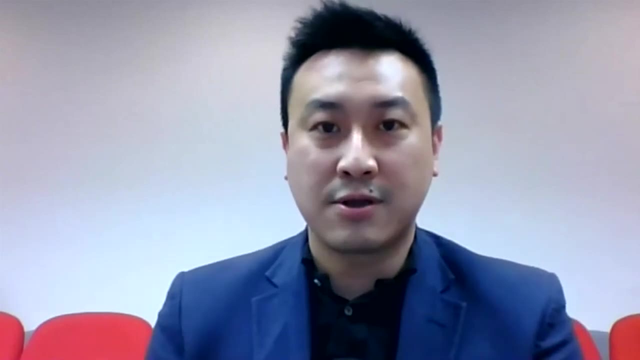 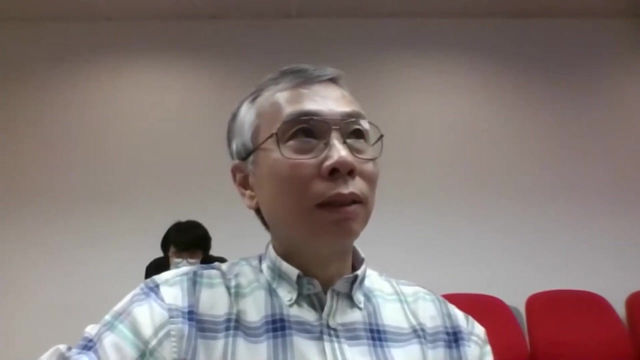 because of Fort Hood. I mean, we will see how the citizens are feeling. Yeah, Thank you, Very interesting, Thank you. Thank you So, um, Is there any further questions for Jerome? Well, I guess I need to explain the name of Jerome, right? 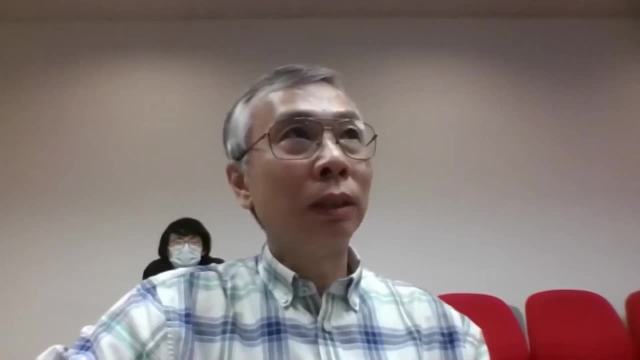 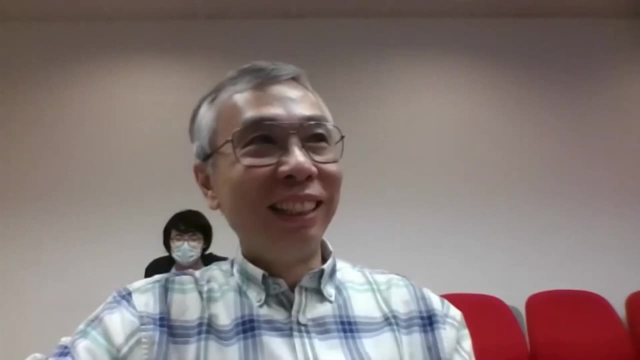 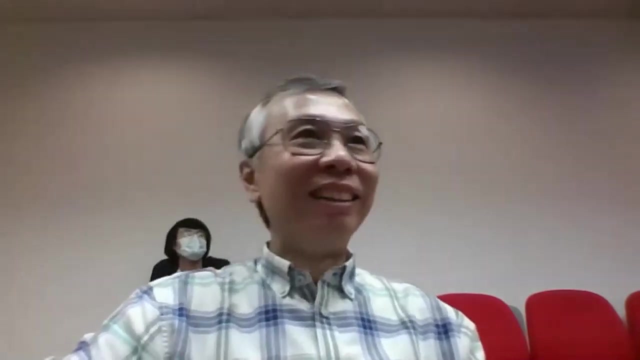 So, Jerome Hoi, you saw his J-H also similar to Tufenai Hormone. So I always believe that is the reason why he is addicted to the study of Tufenai Hormone, because of his leg, Anyway. Uh, is there any other questions? 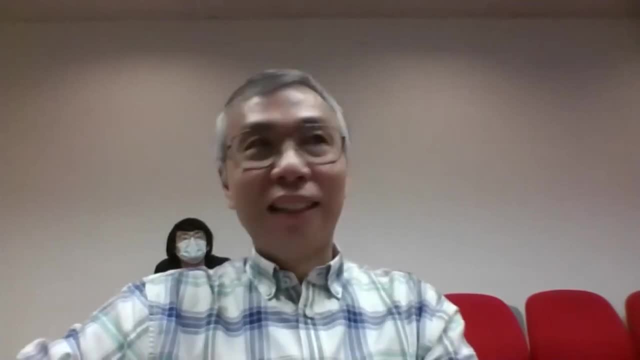 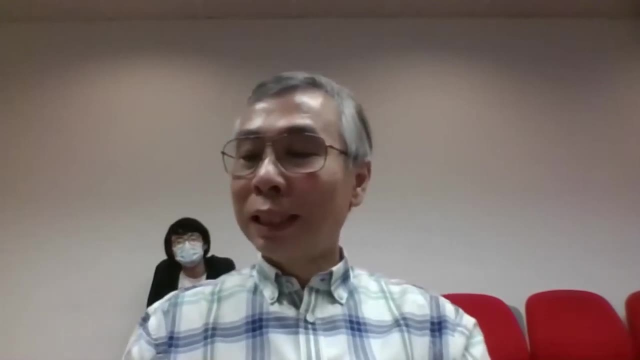 Uh From the floor. Okay, So if not, let me um first of all. first of all, let me thank you everyone for your active participation and uh discussion. So I would like to do some advertisement for our next talk. 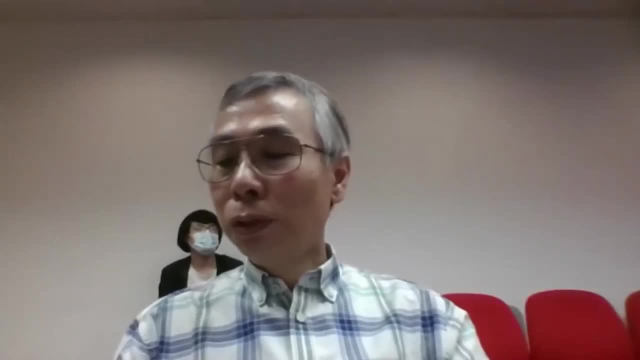 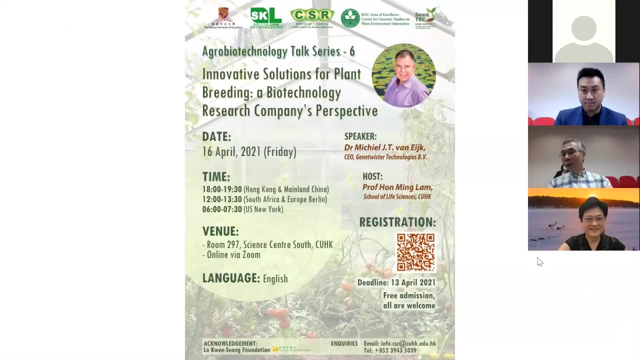 So our next talk will be on the topic of innovative solutions for plant breeding, a biotechnology research company's perspective by Mathieu Van Eyck from Netherlands. So Van Eyck is the uh, the principal scientist in the agricultural industry plant, and he 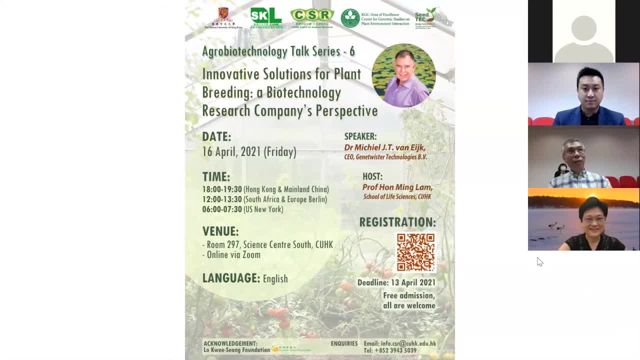 invented many technology, you know, for agricultural application. So we we are very honored to have him to discuss agriculture in in the viewpoint of a company, So a research company. So I hope that uh his perspective will help those who would like to develop in uh agricultural. 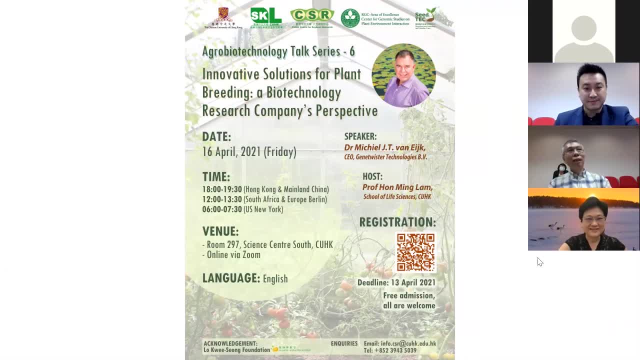 industry, especially our friends in South Africa. Okay, So if you're interested, you can just using your cell phone to register by scanning the QR code, And my assistant will also send you the invitation later, if you have leave your email to us.